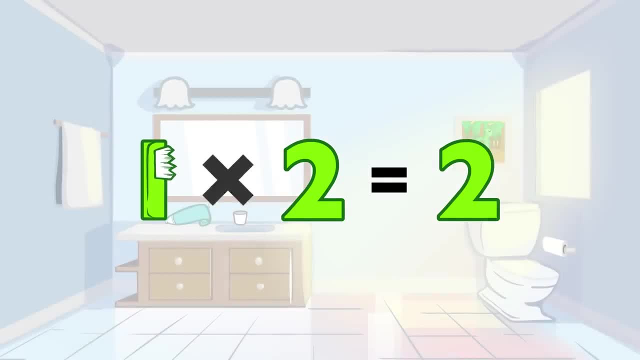 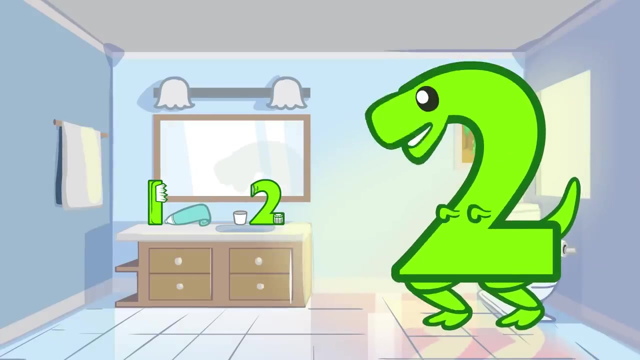 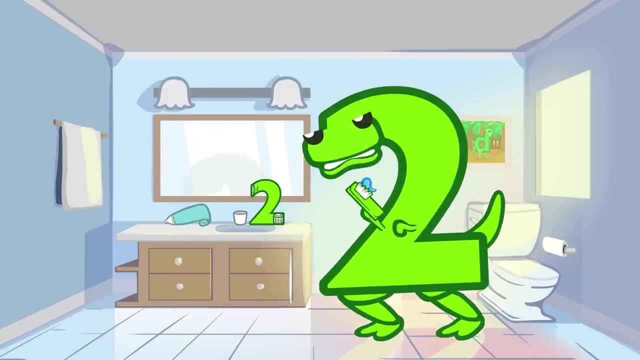 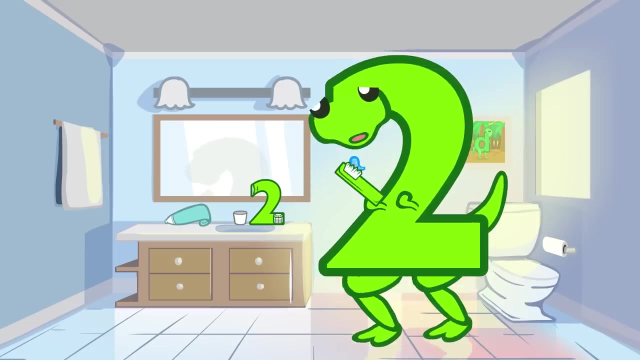 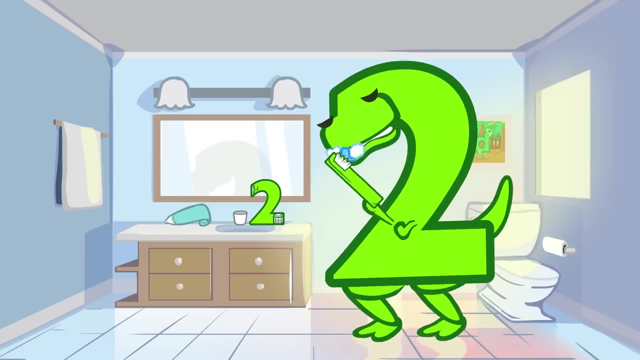 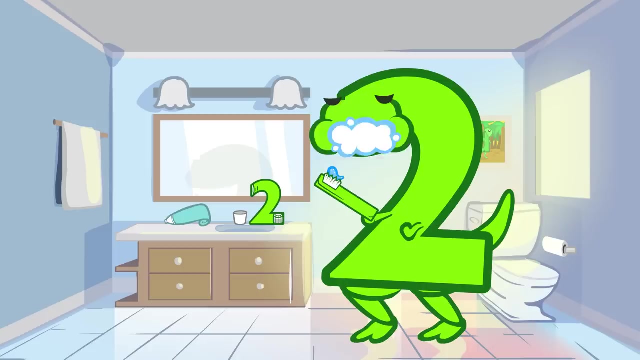 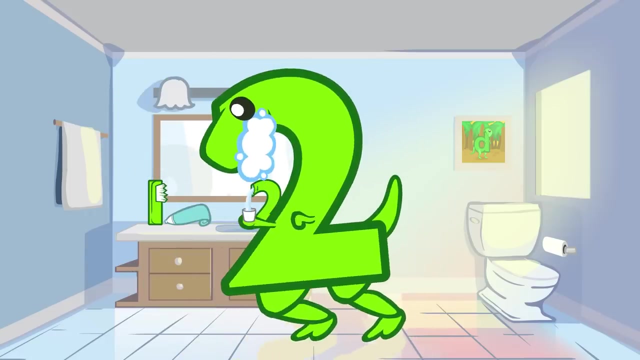 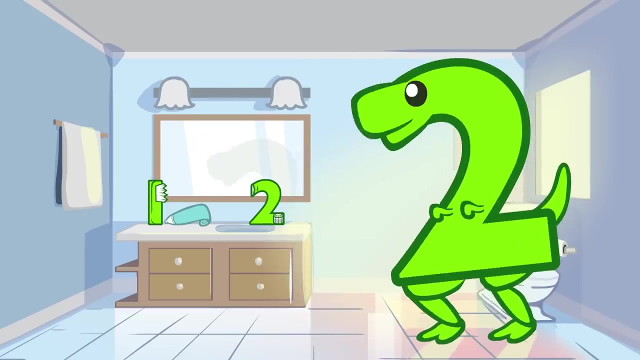 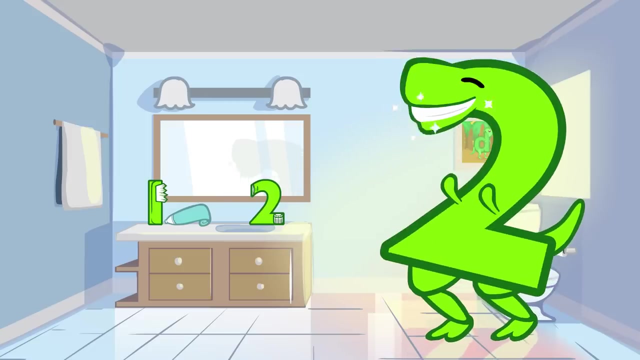 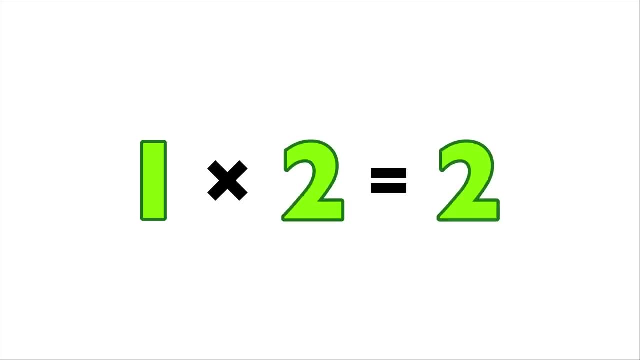 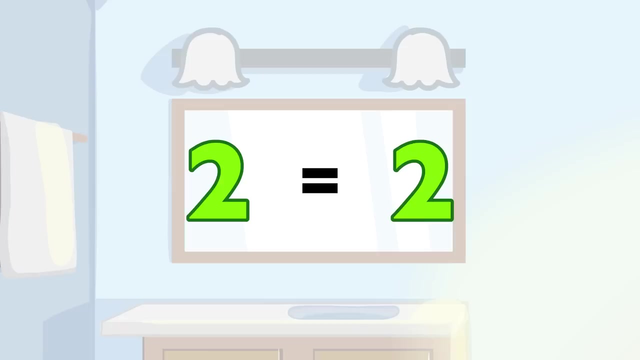 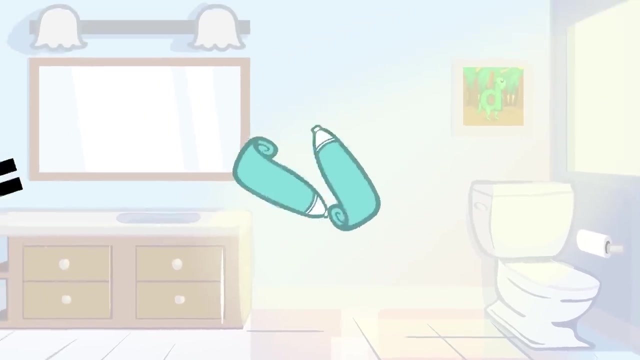 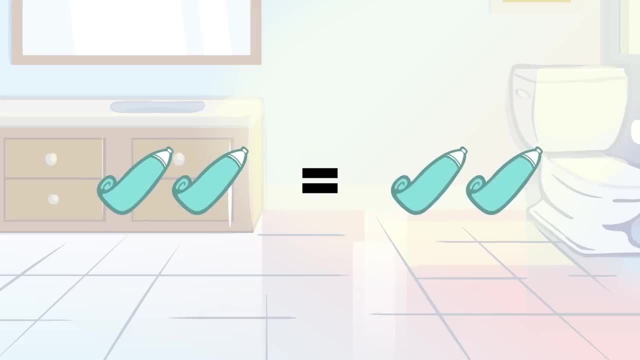 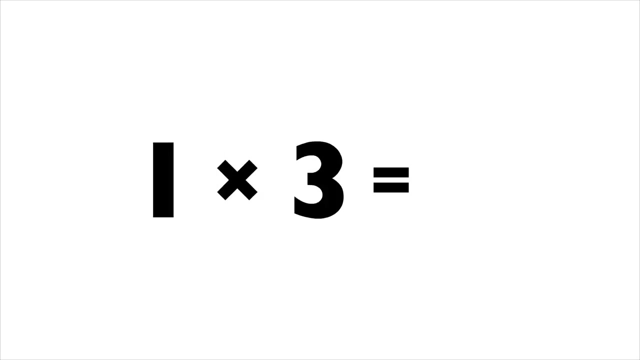 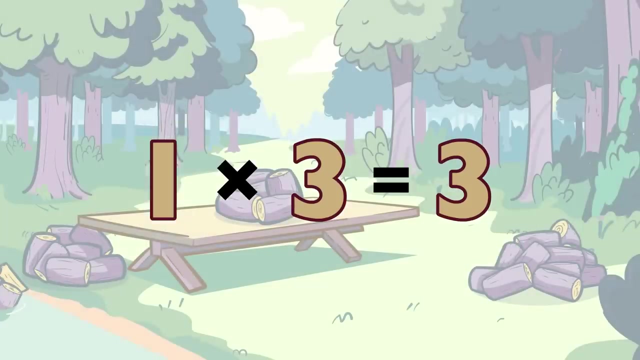 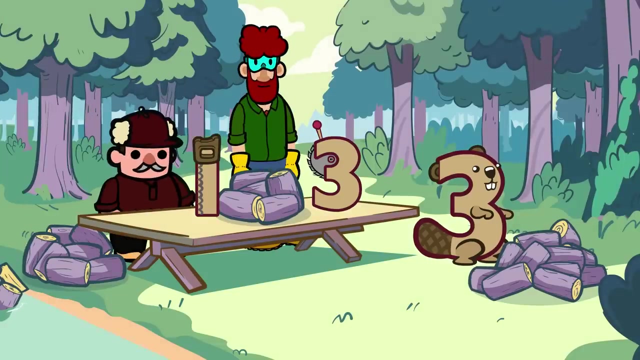 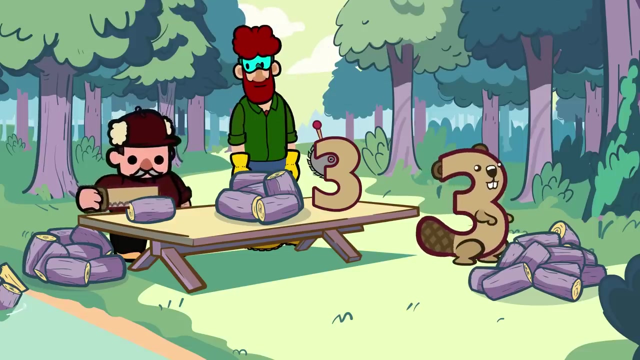 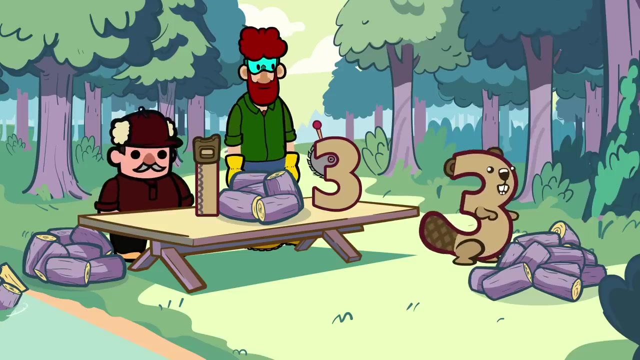 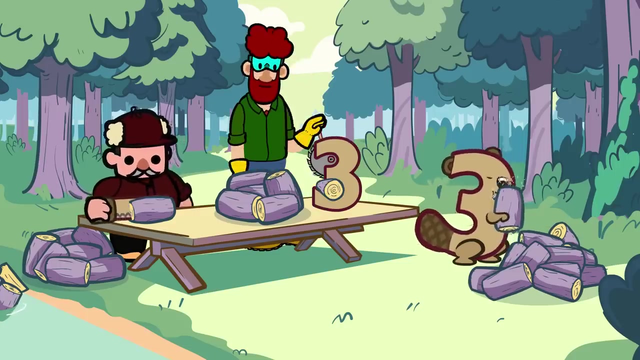 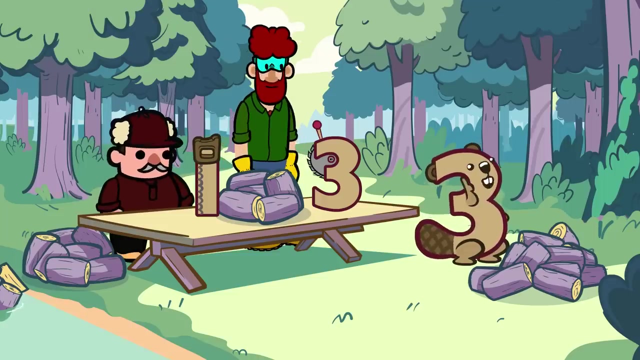 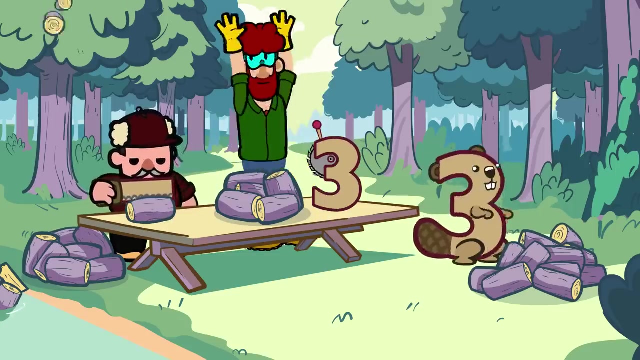 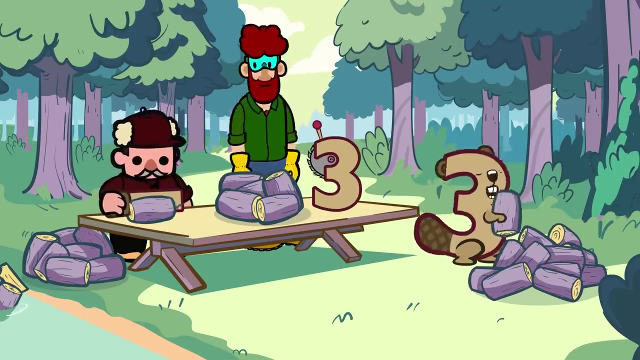 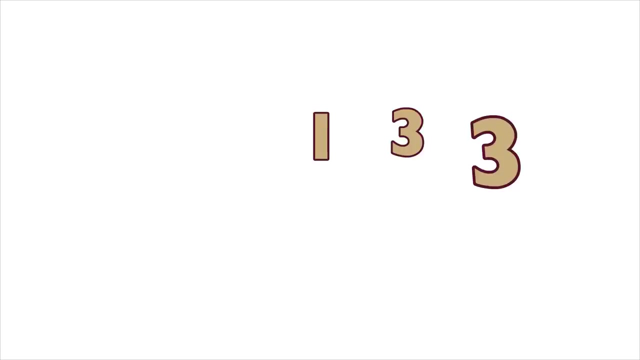 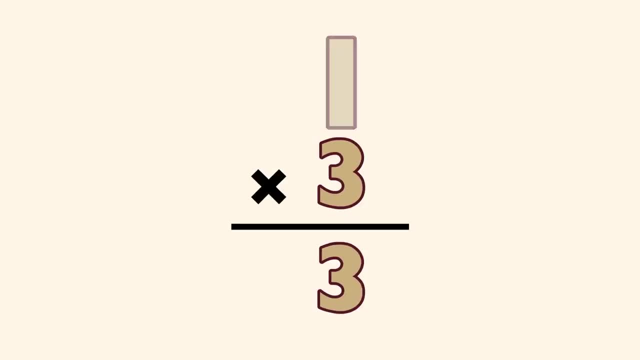 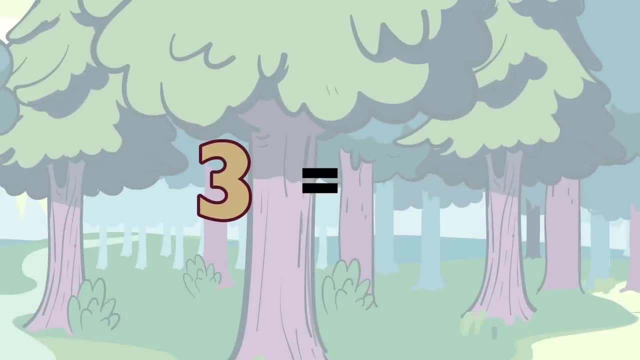 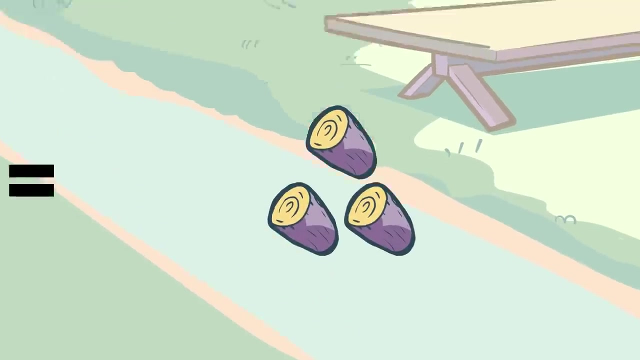 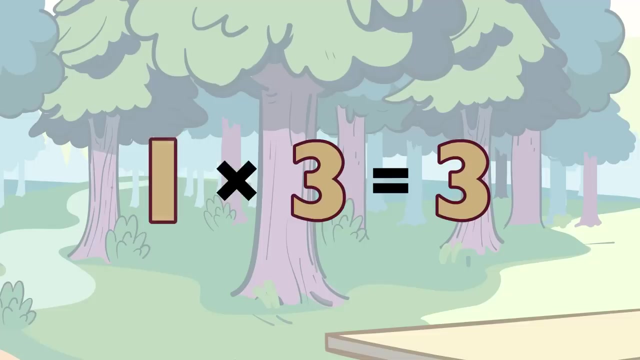 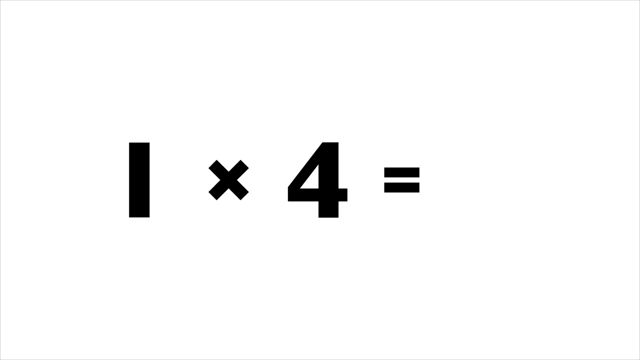 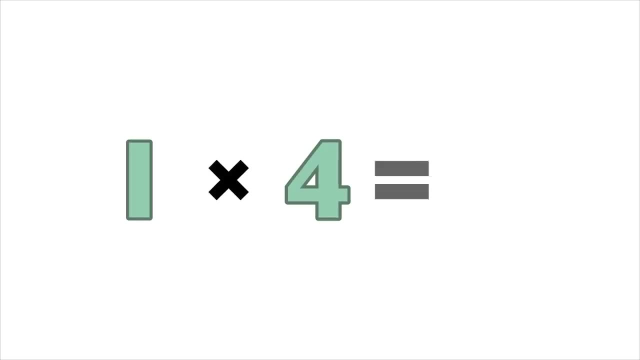 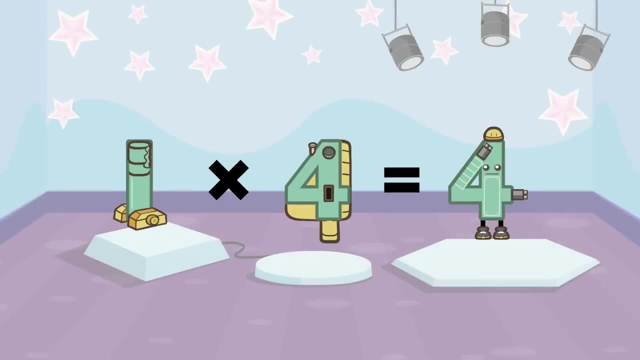 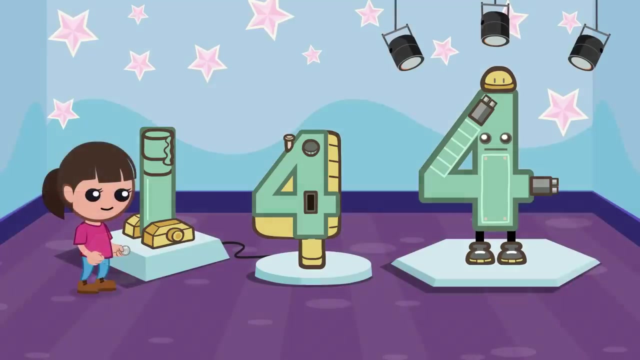 1 times 4 equals 4.. 1 times 4 equals 4.. 1 times 4.. 1 times 4: equals 4.. 1 times 4: equals 4.. 1 times 4: equals 4.. 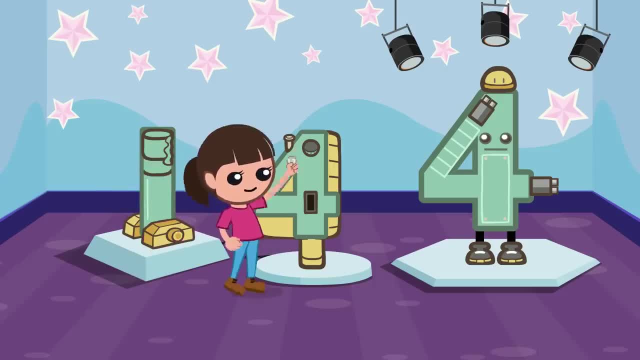 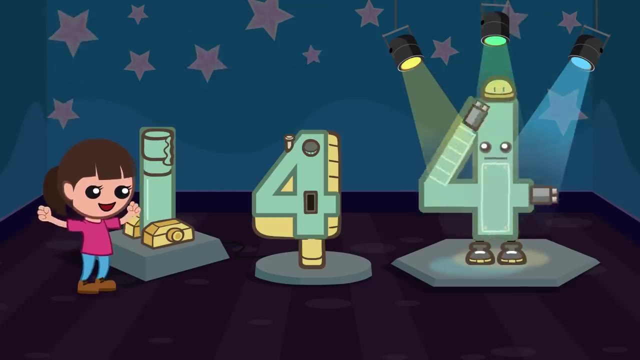 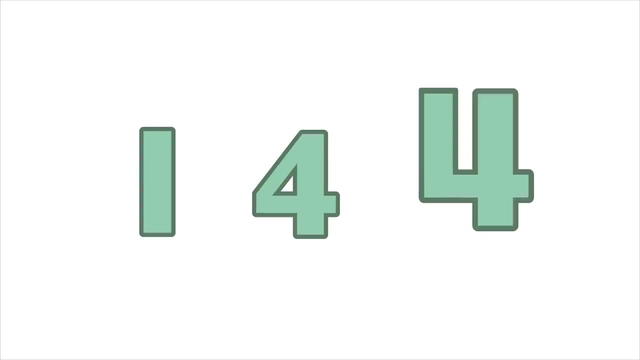 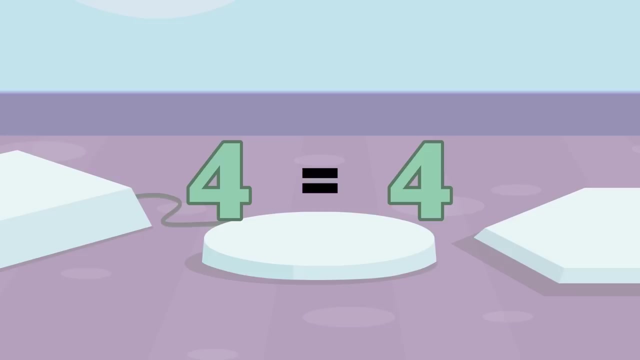 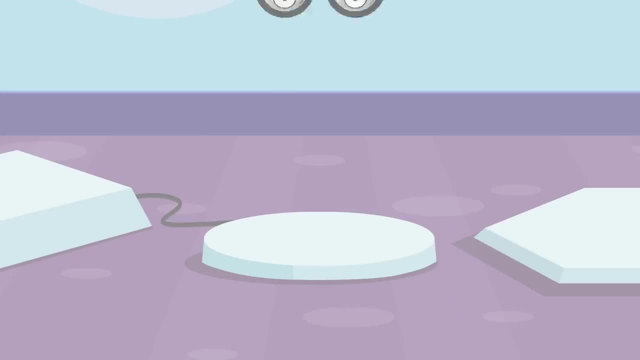 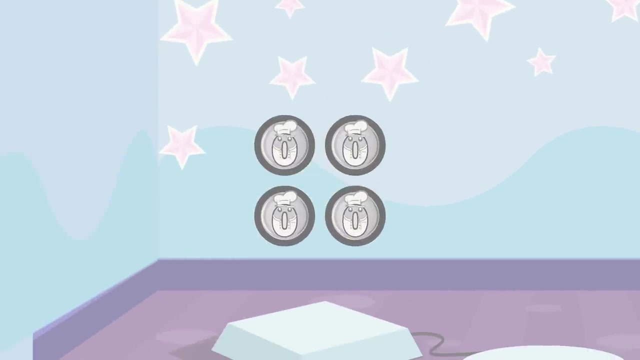 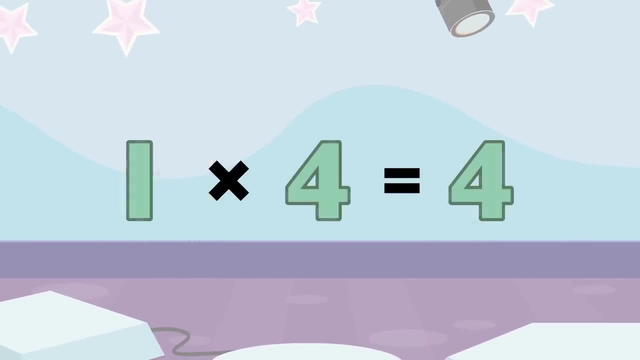 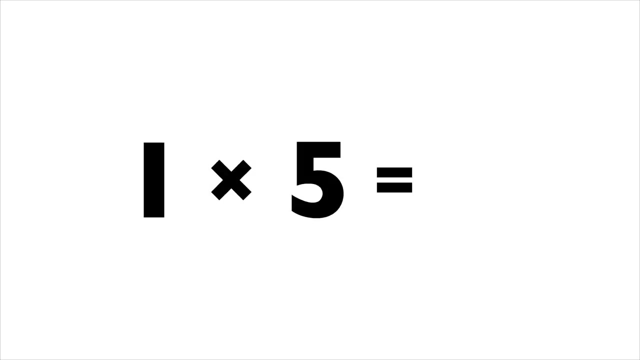 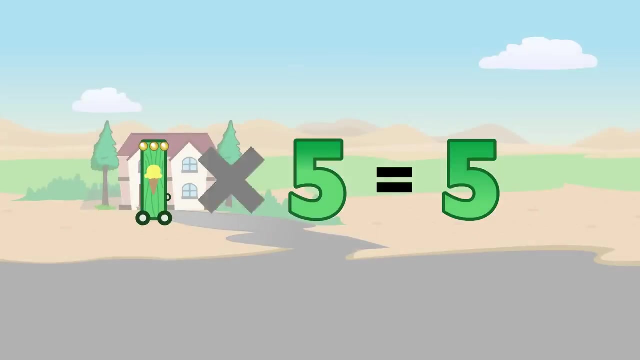 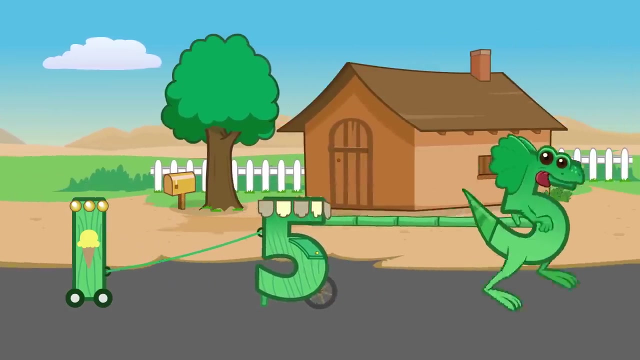 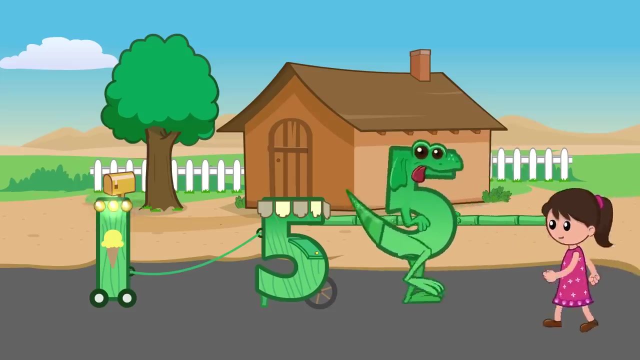 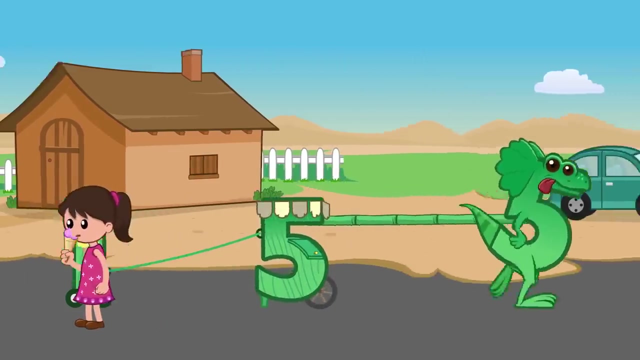 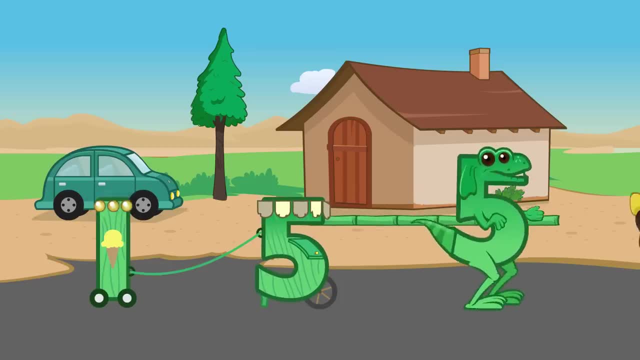 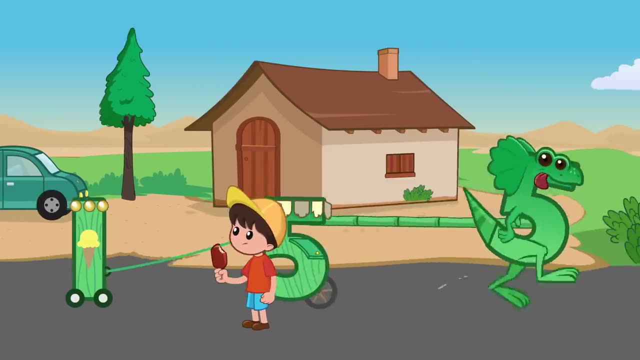 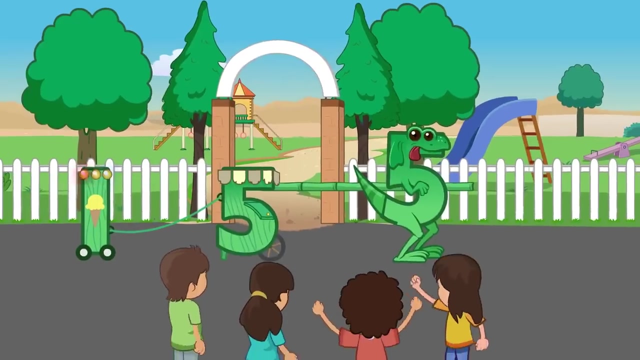 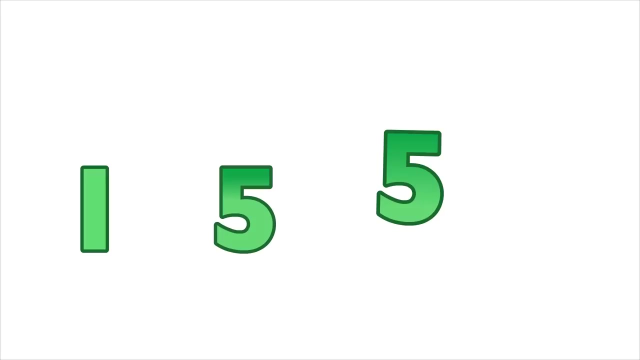 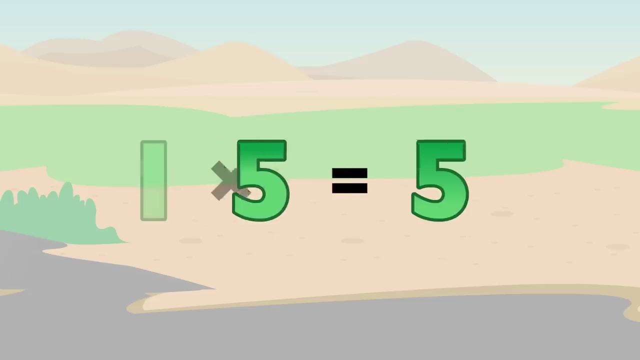 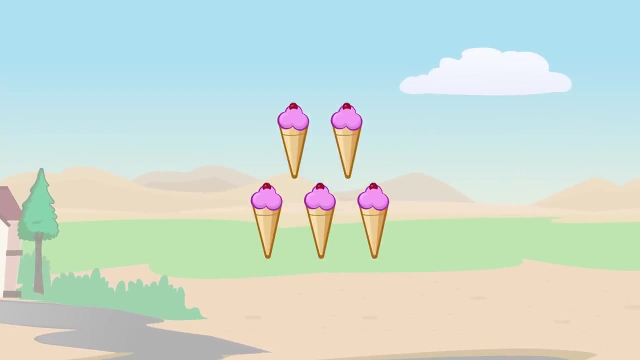 One Hoggie Two. Four equals four. Four equals four. How many are there? One times five equals five. One times five equals five. One times five equals five. One five equals five. One times five equals five. Five equals five. 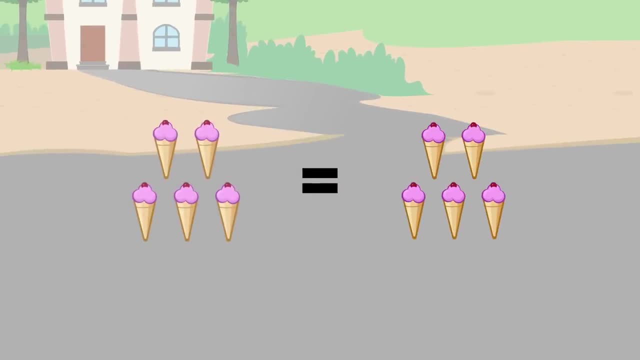 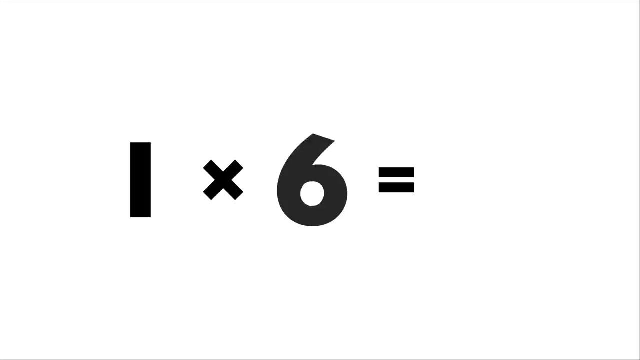 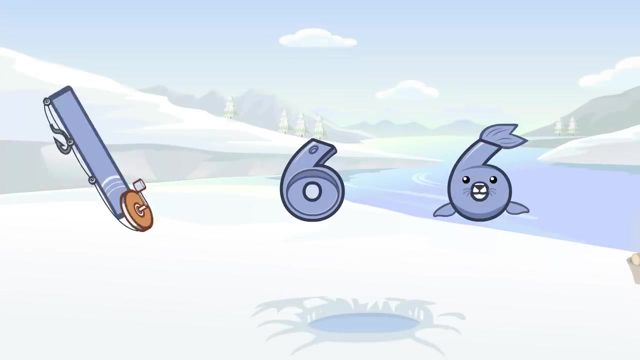 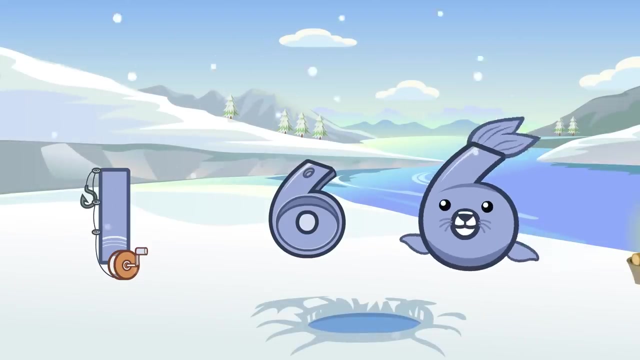 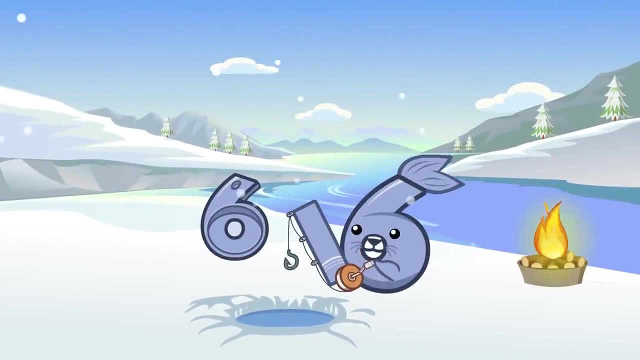 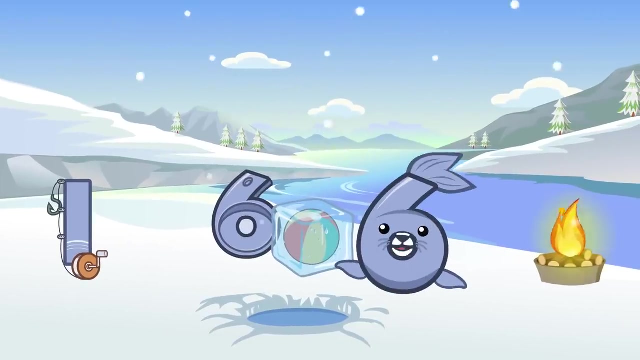 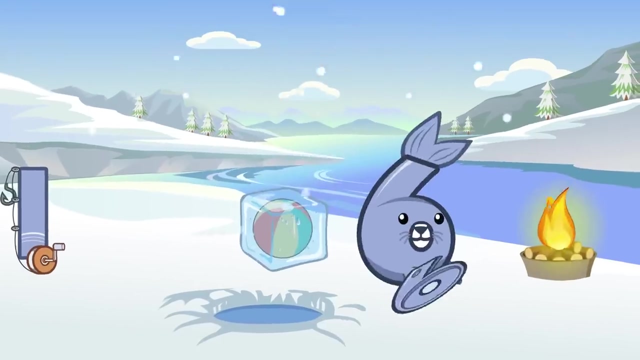 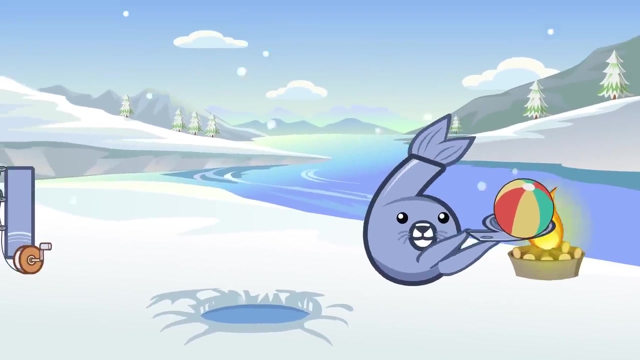 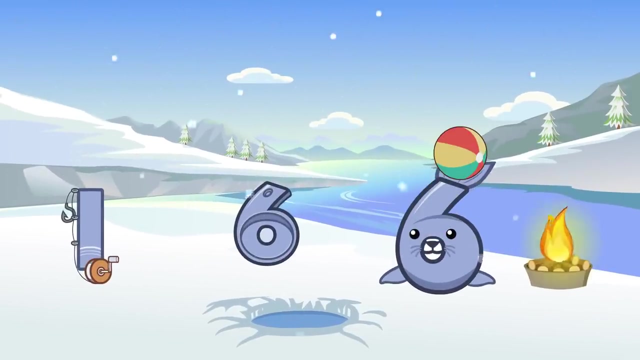 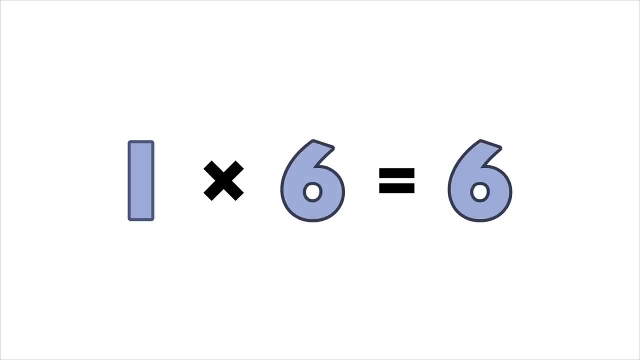 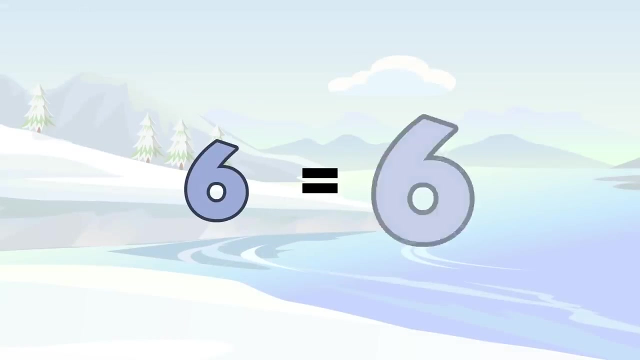 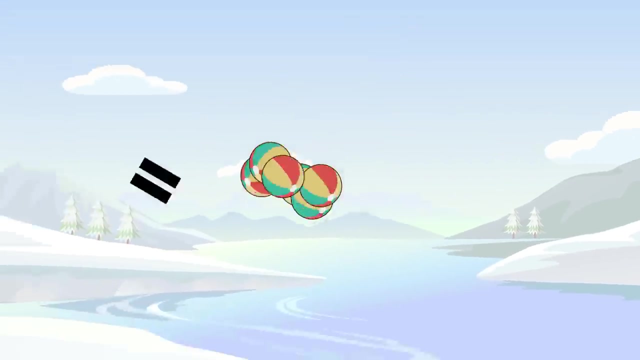 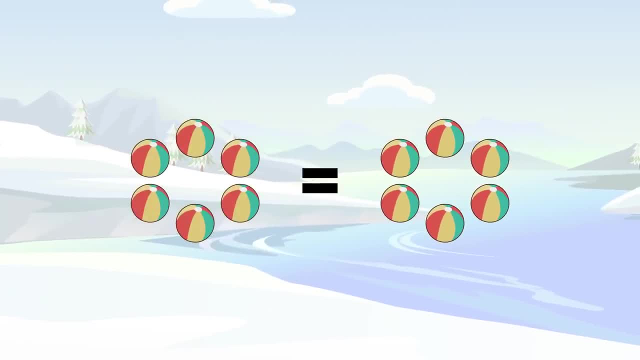 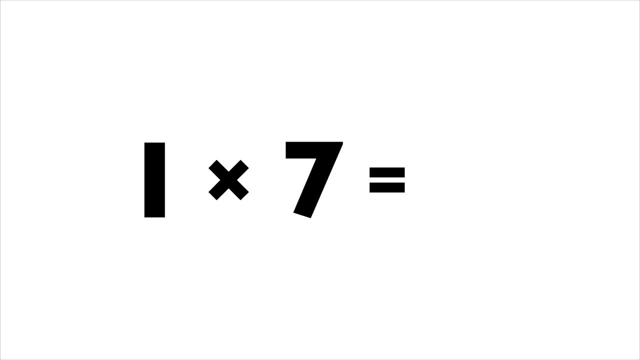 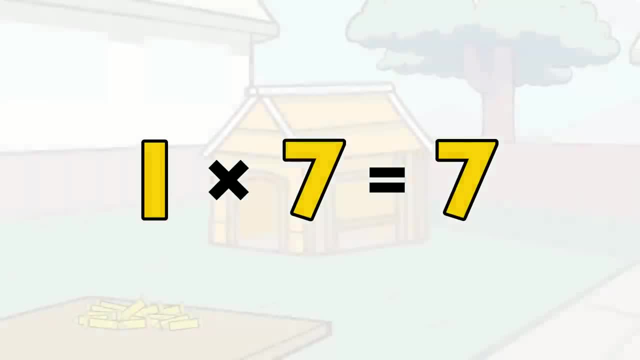 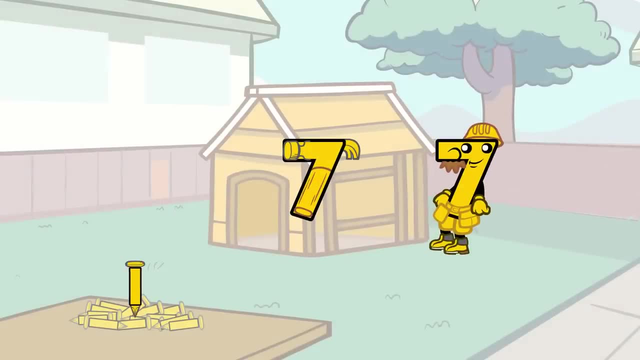 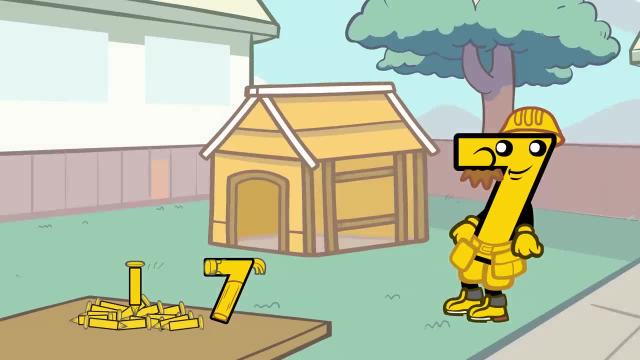 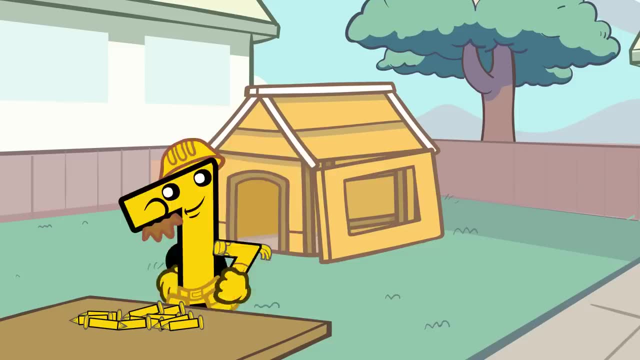 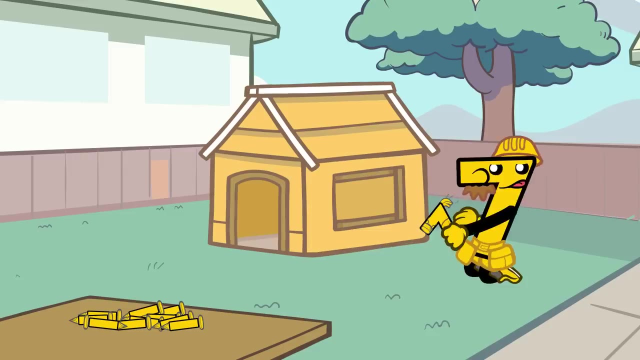 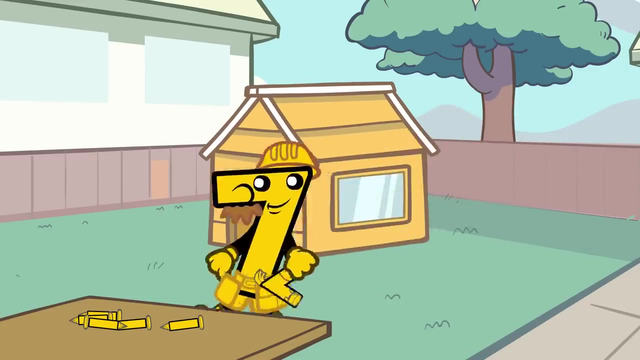 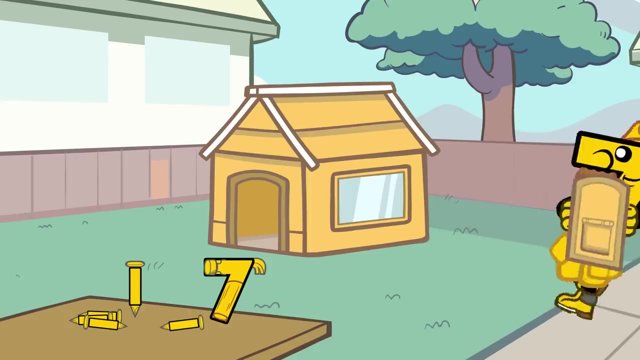 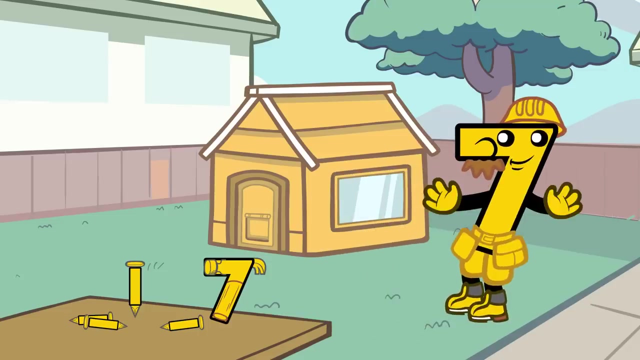 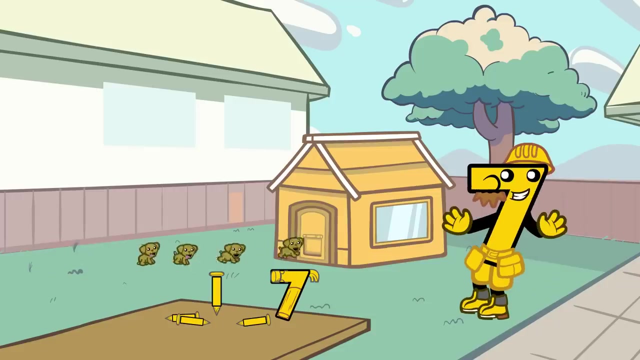 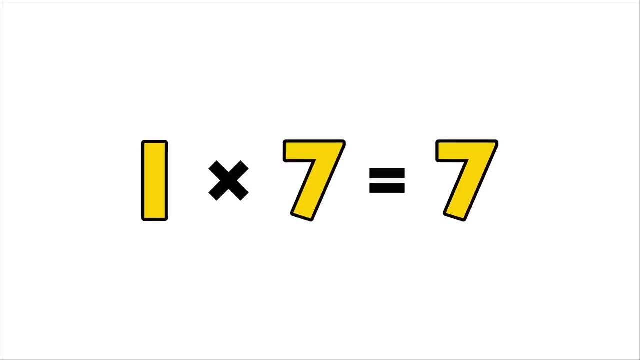 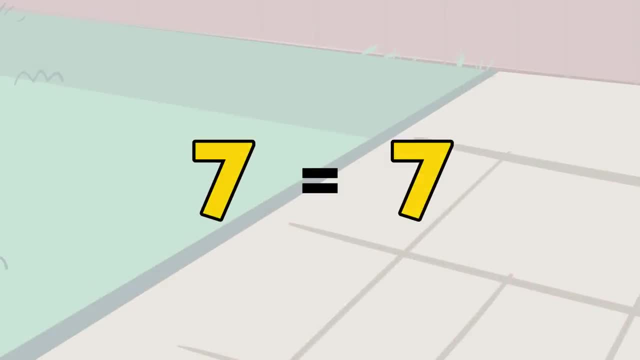 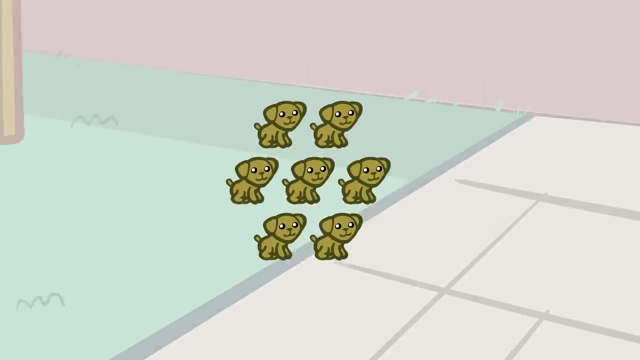 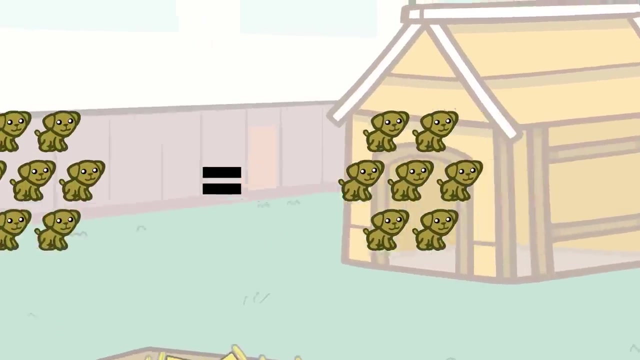 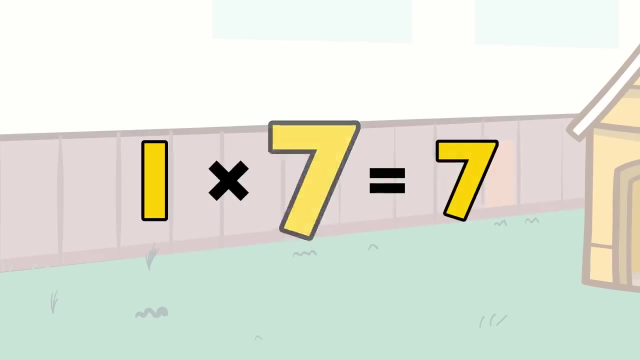 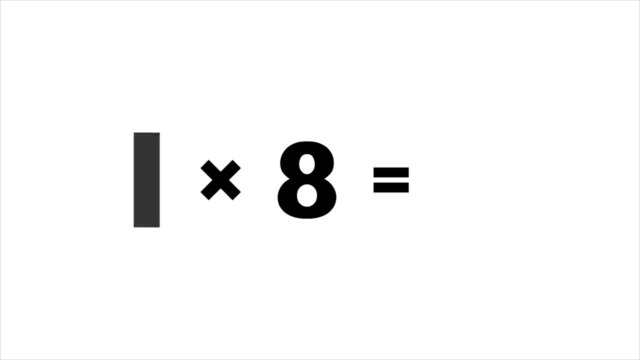 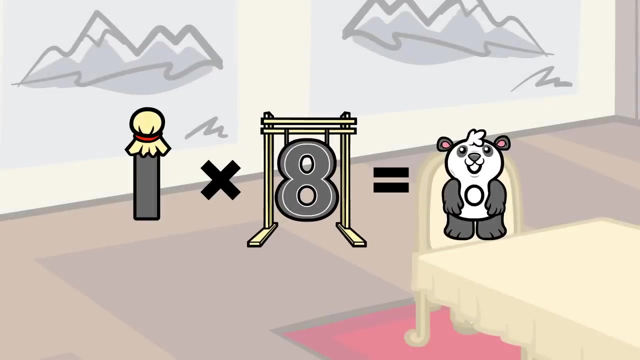 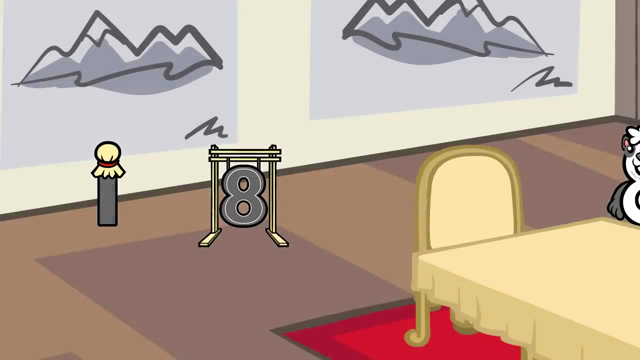 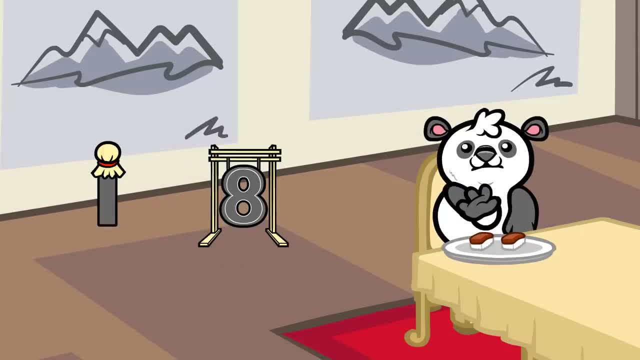 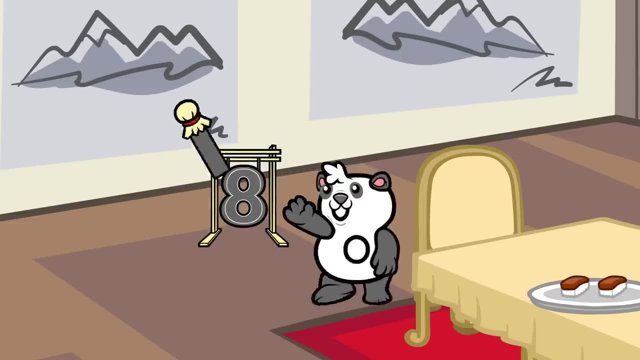 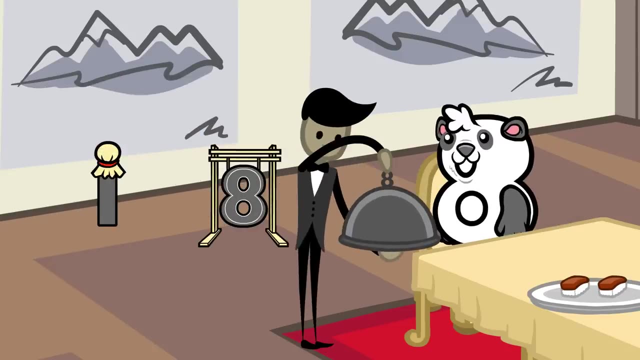 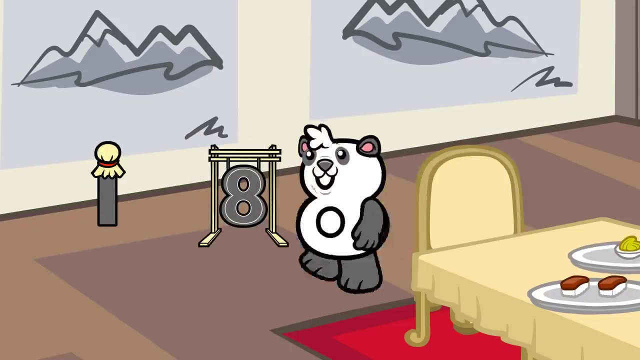 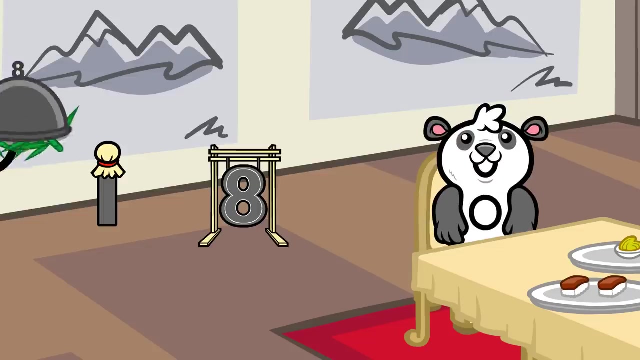 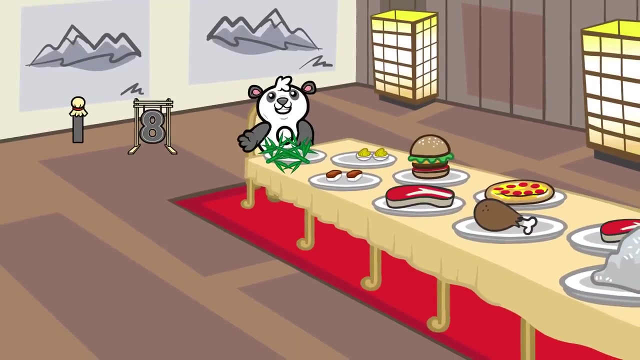 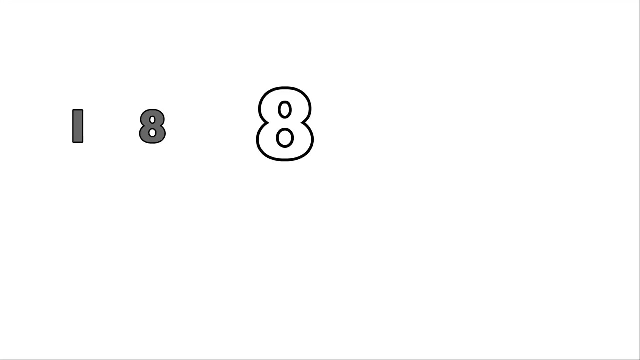 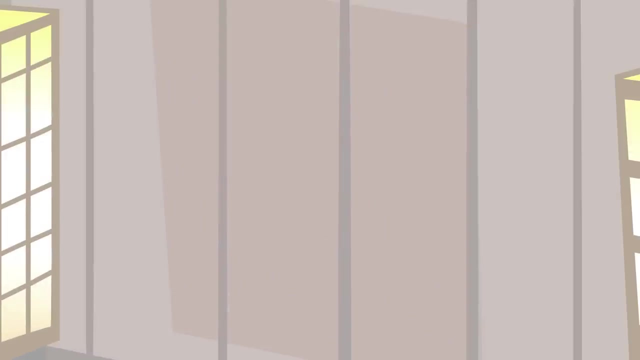 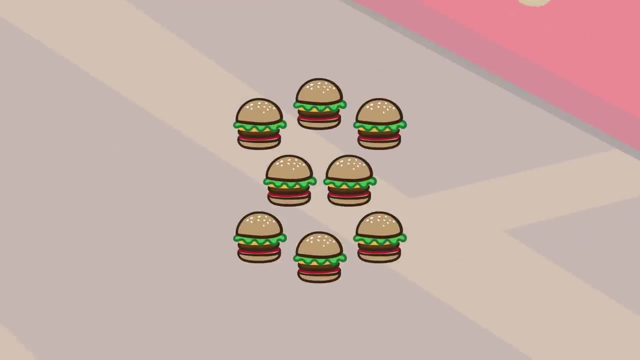 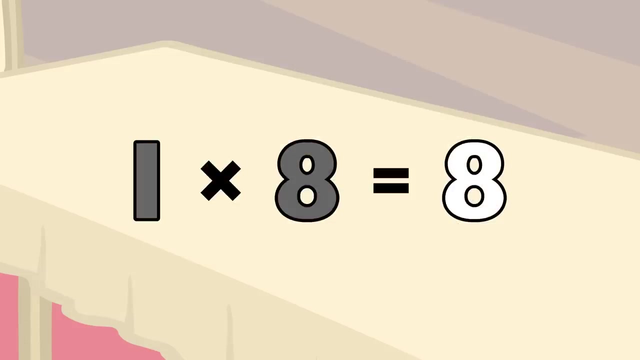 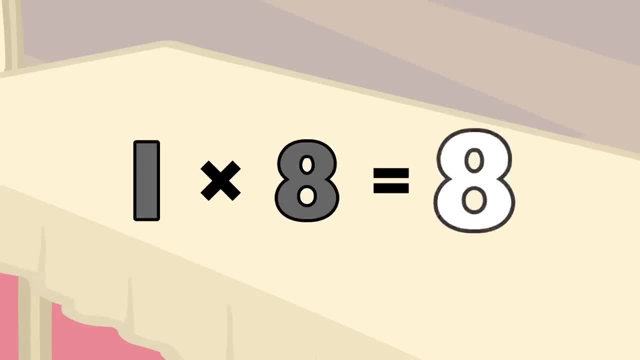 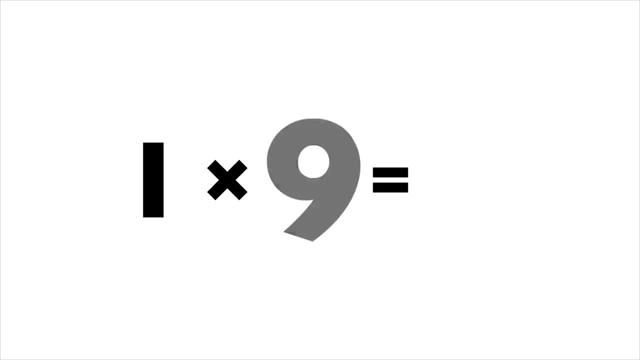 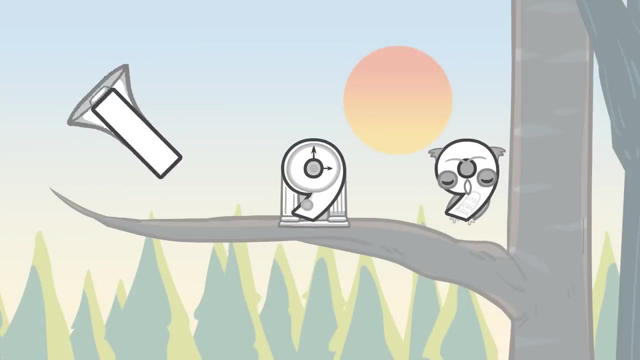 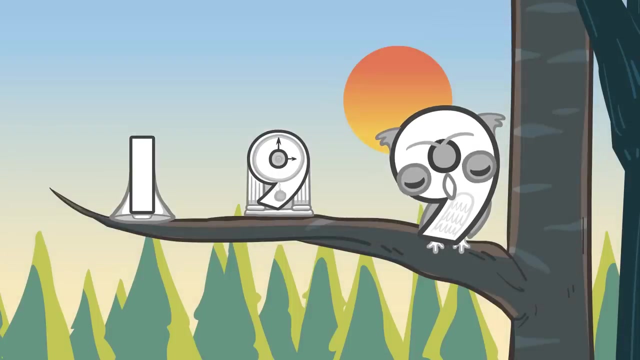 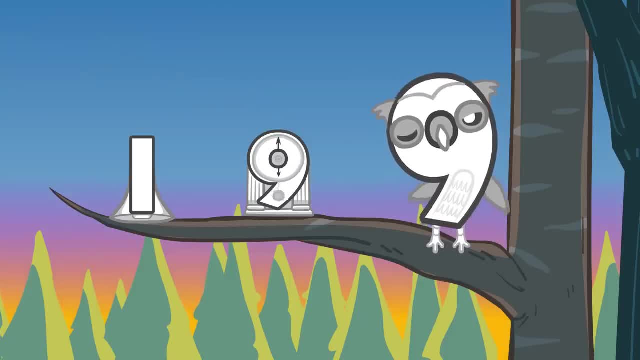 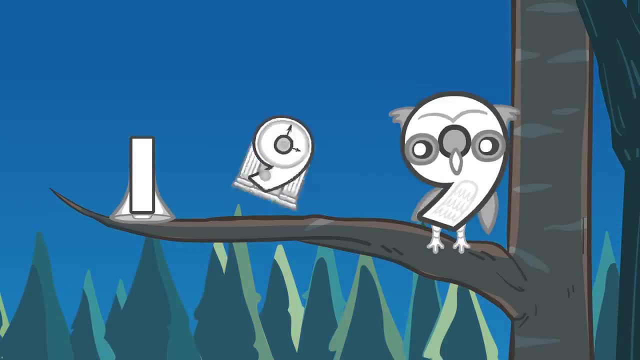 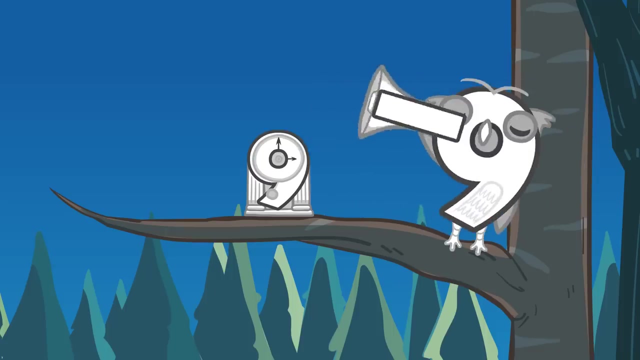 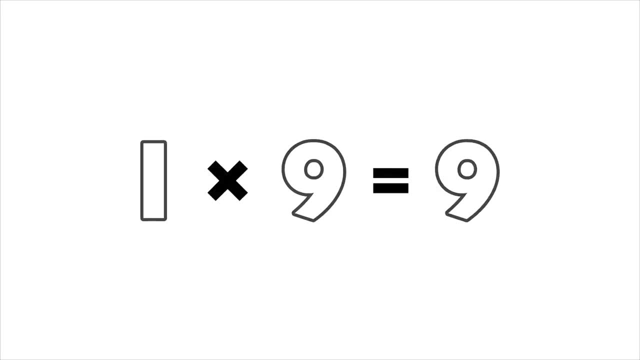 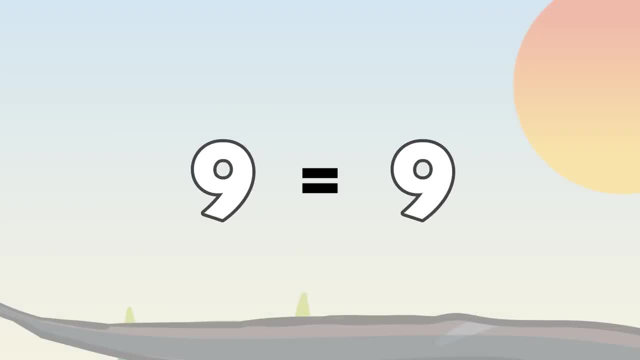 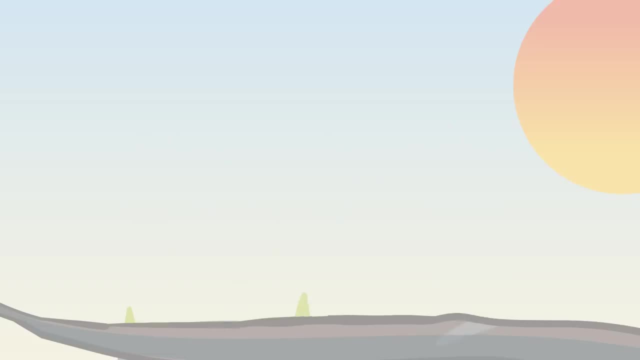 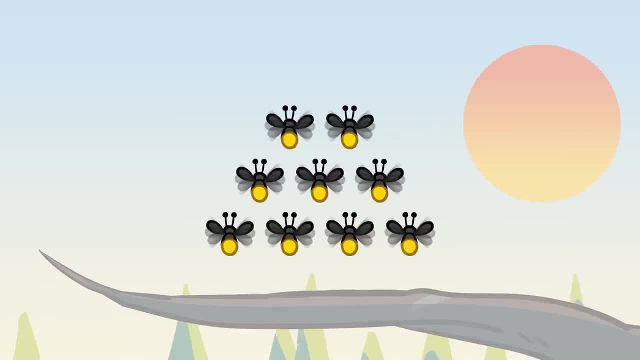 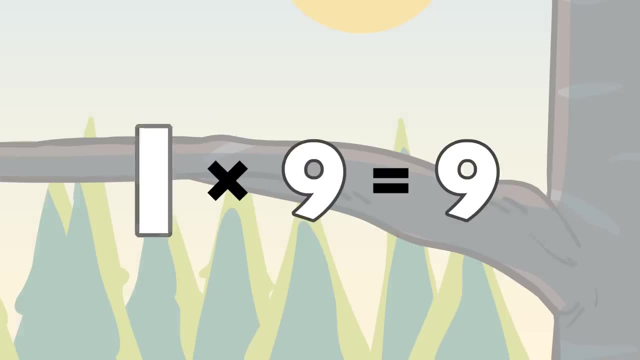 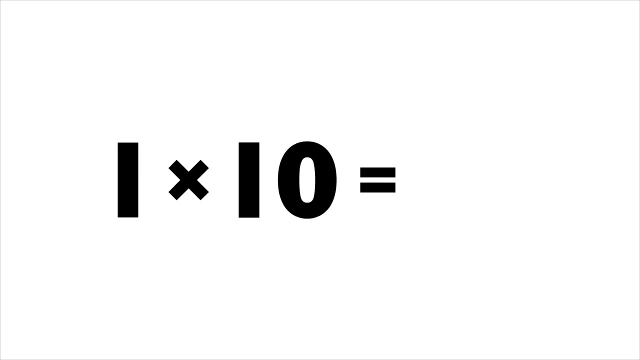 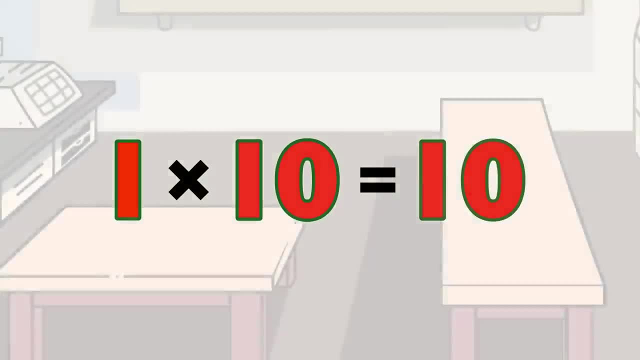 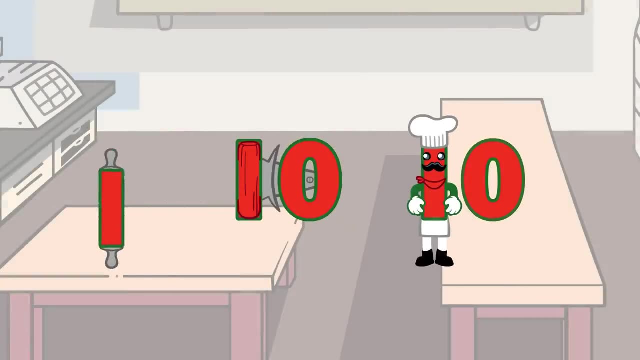 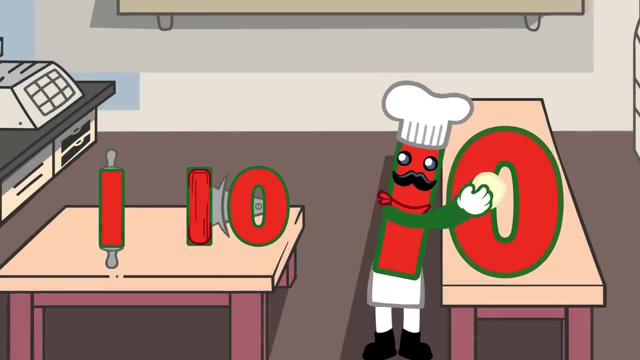 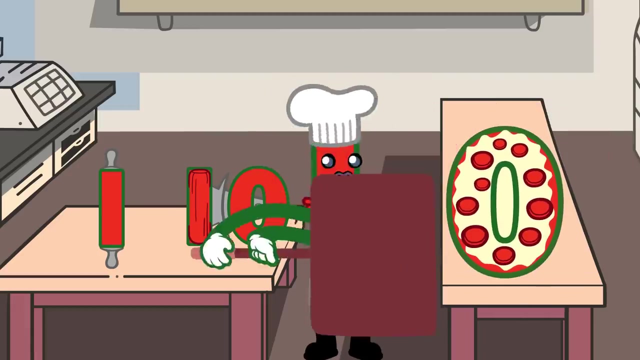 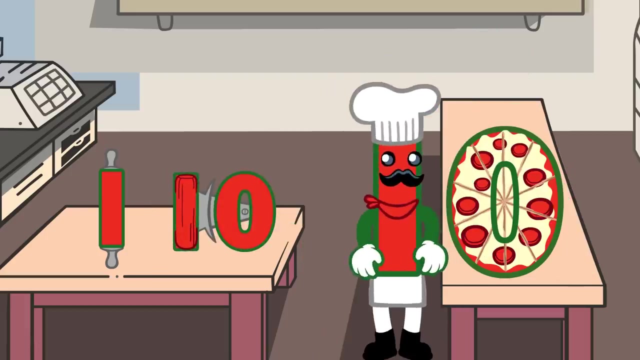 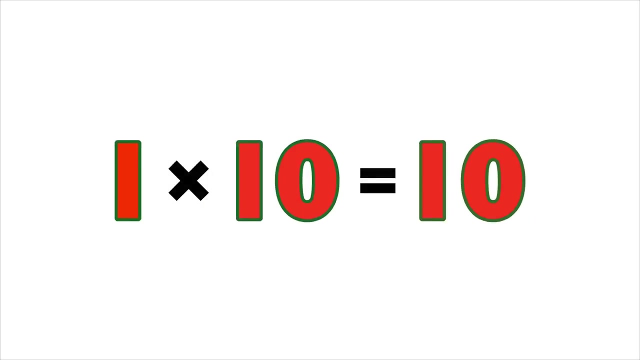 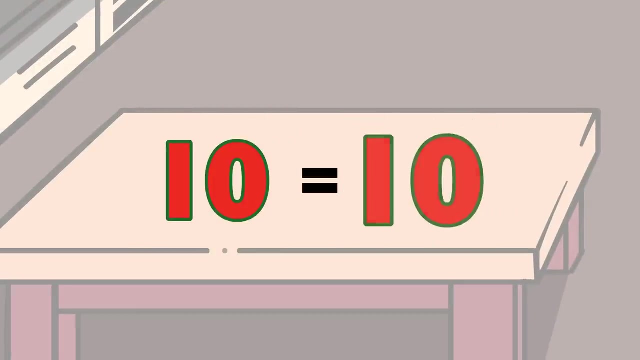 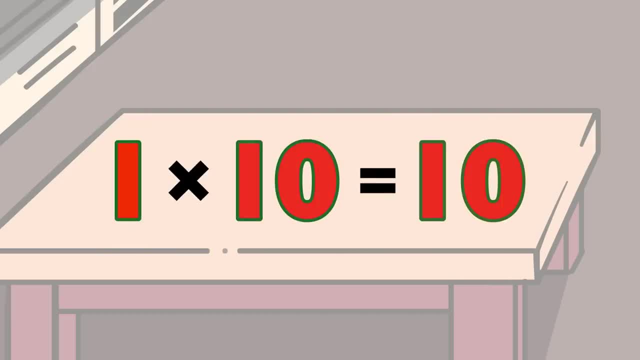 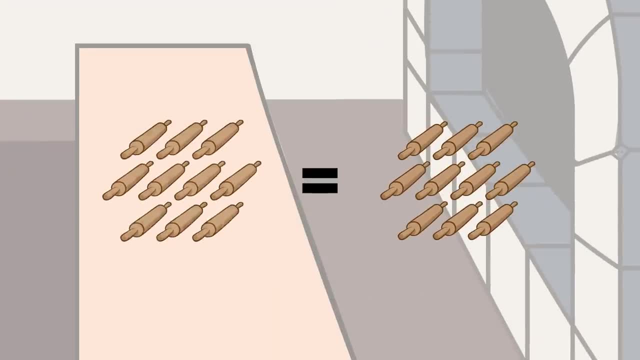 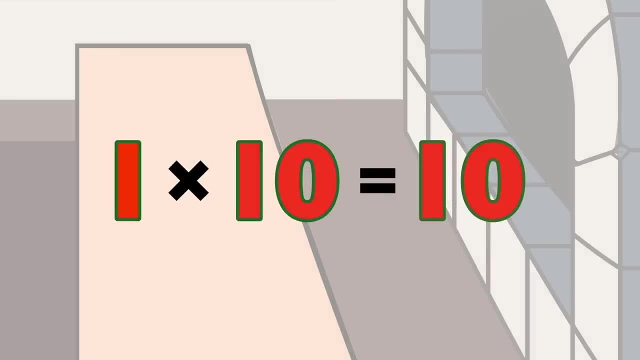 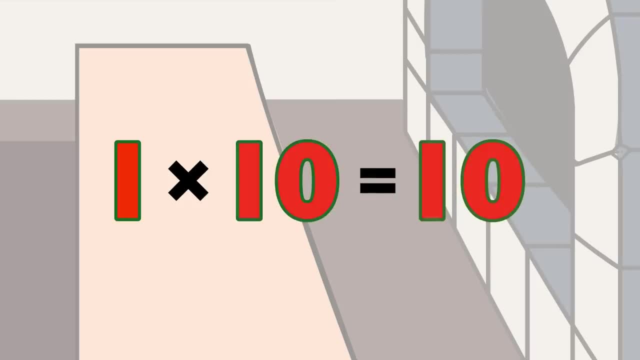 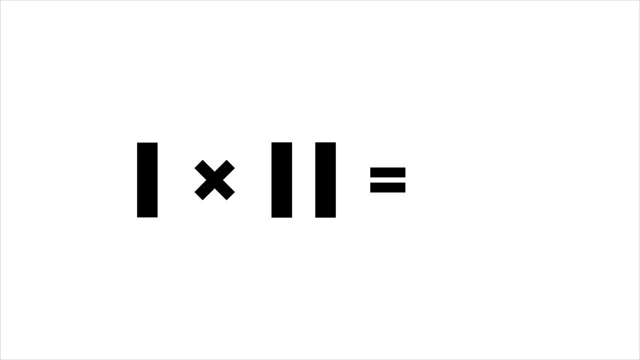 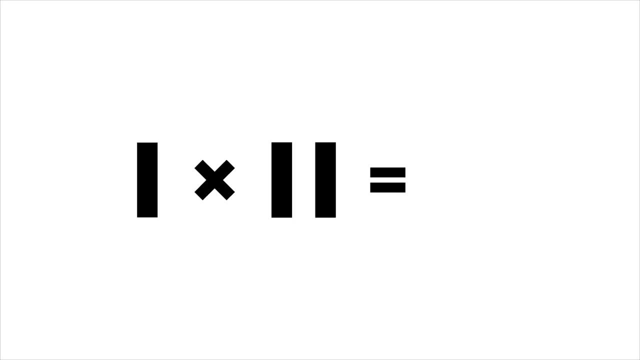 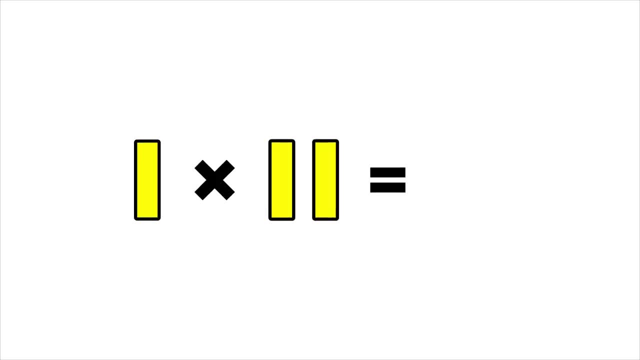 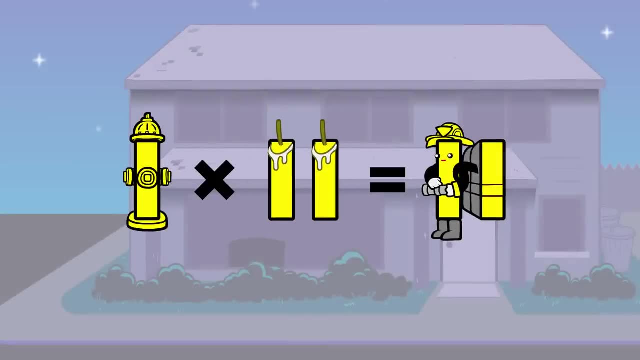 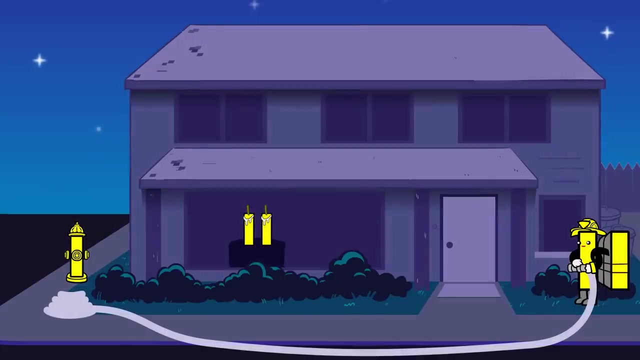 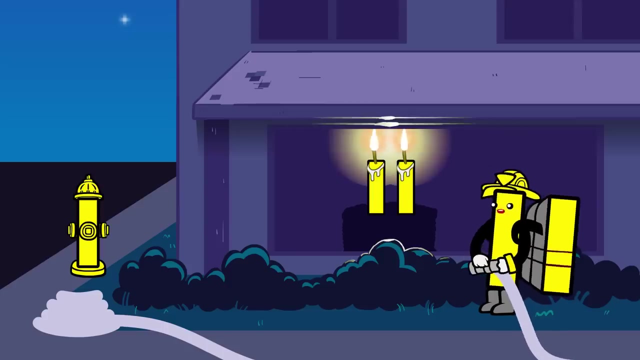 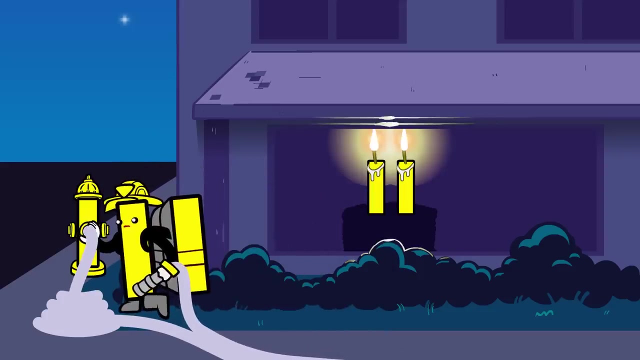 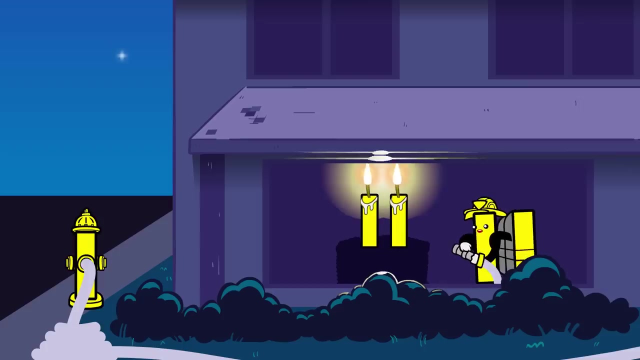 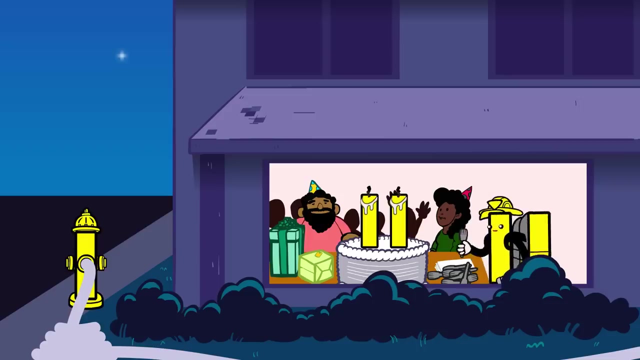 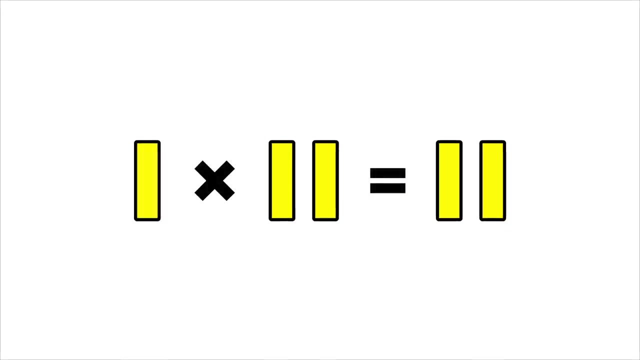 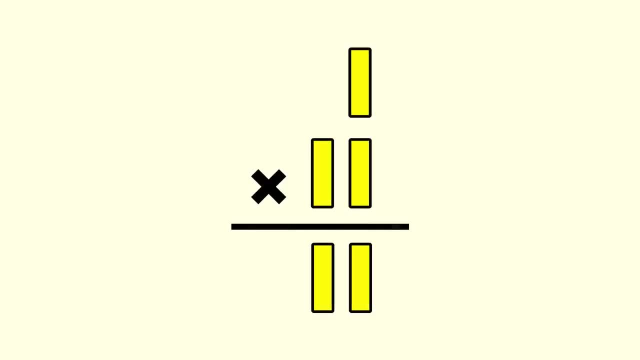 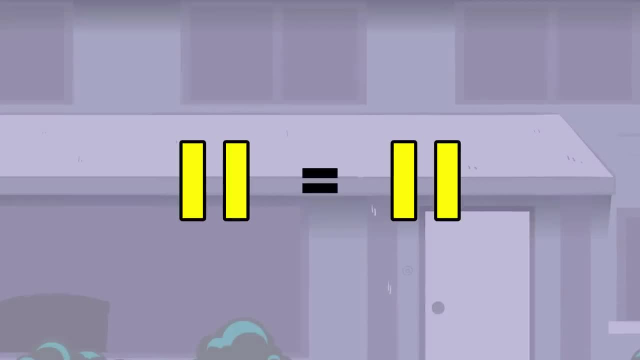 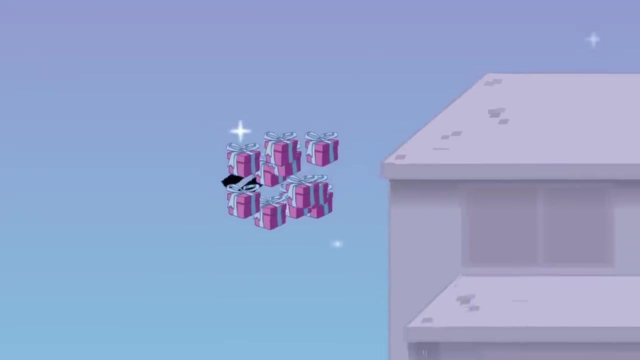 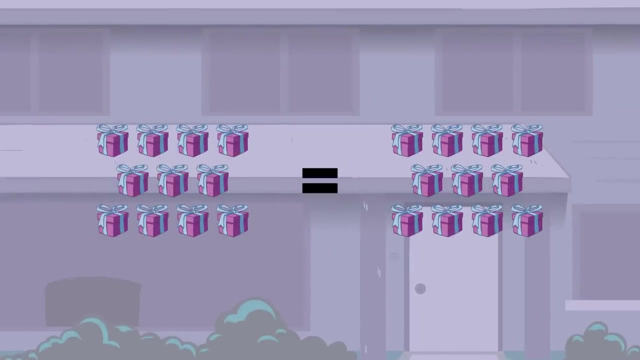 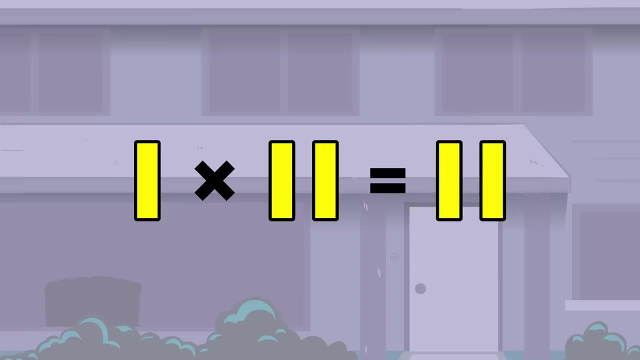 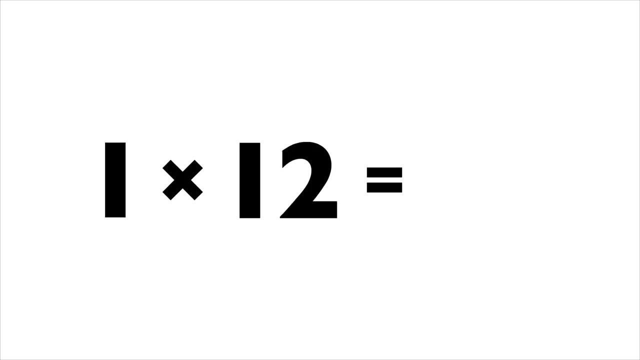 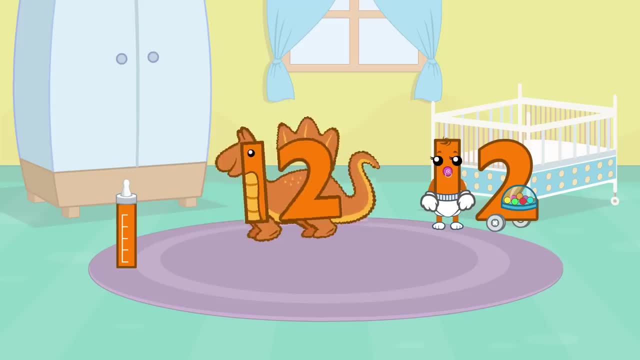 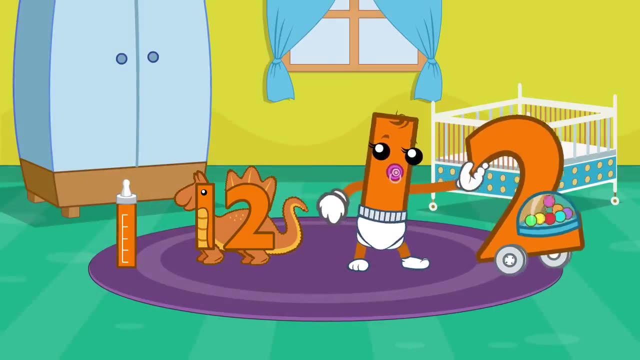 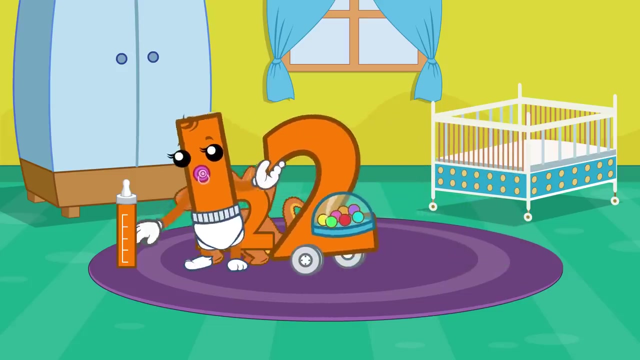 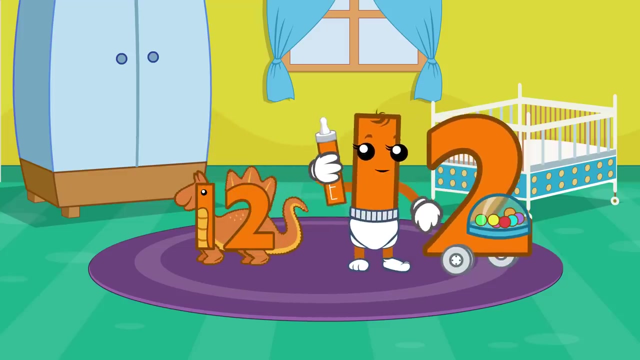 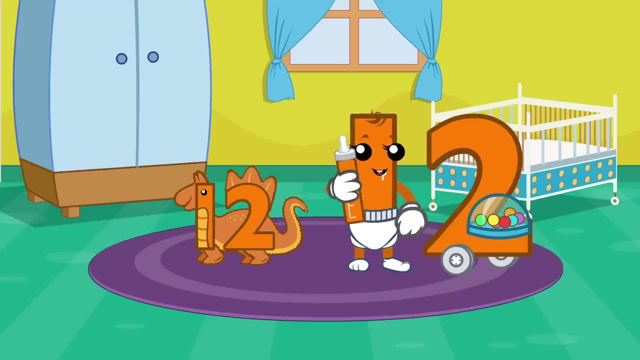 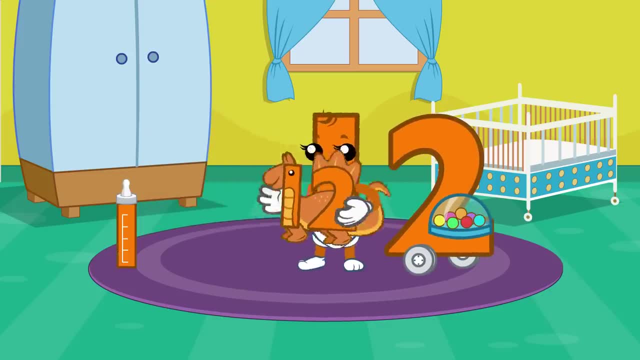 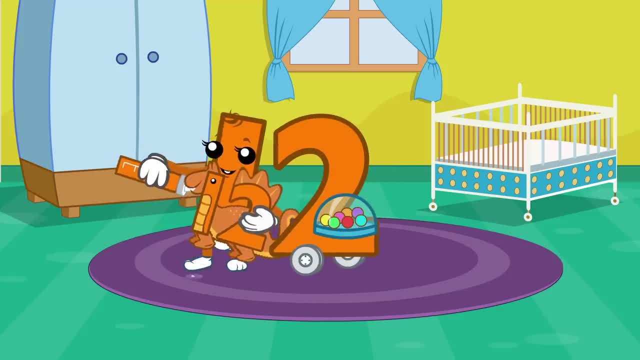 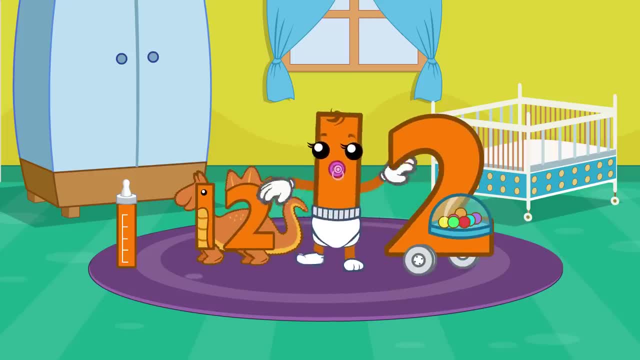 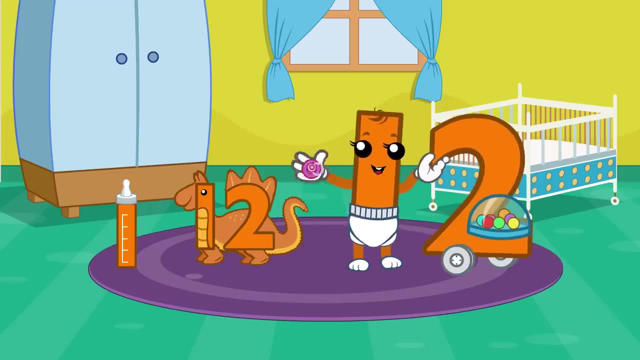 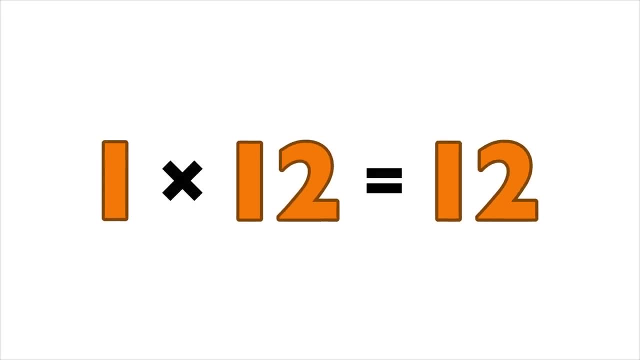 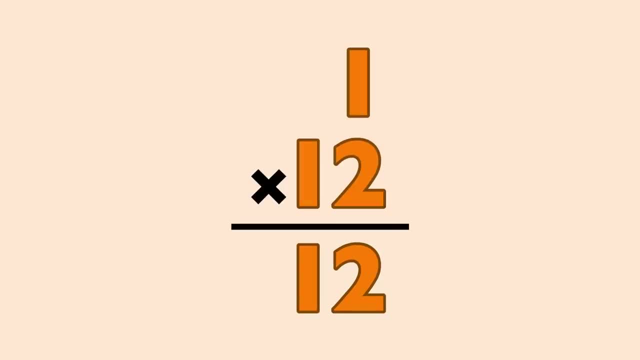 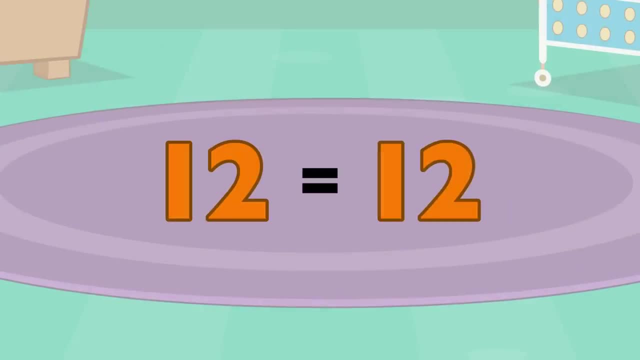 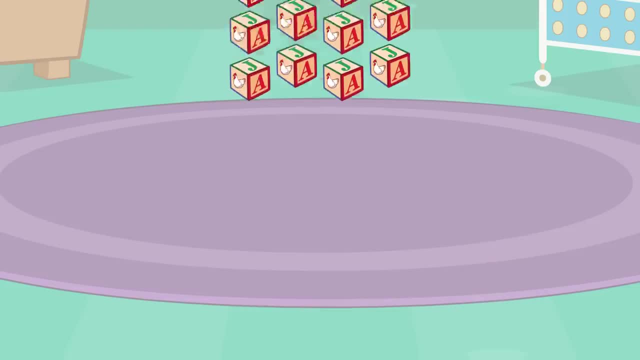 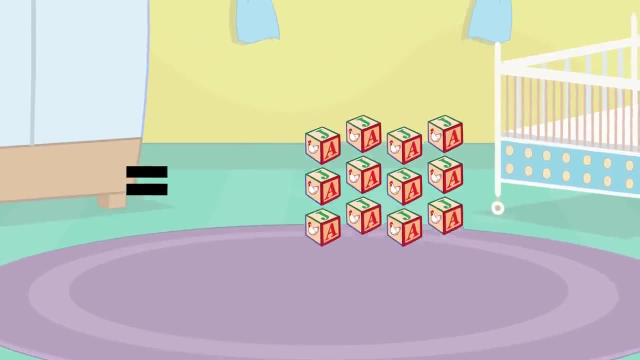 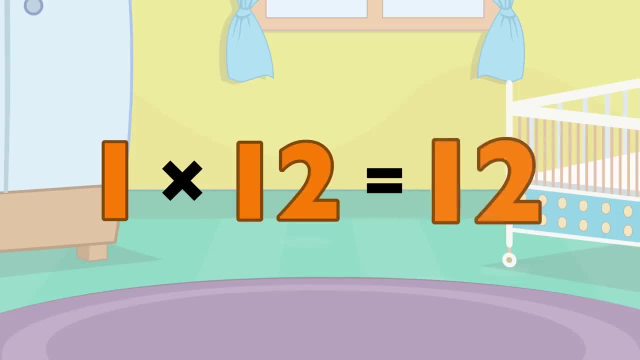 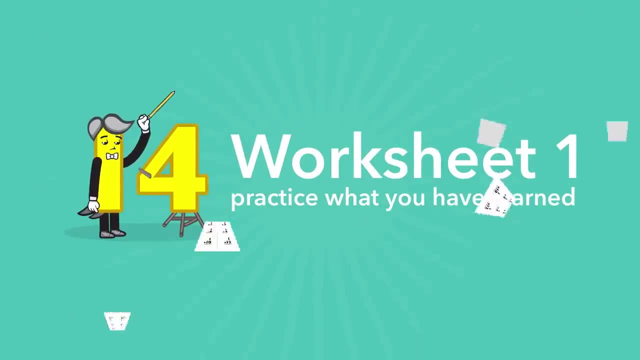 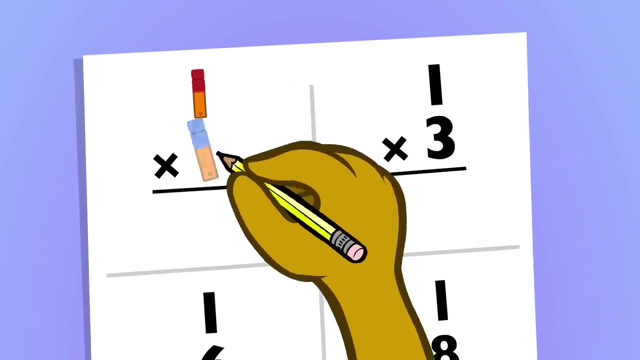 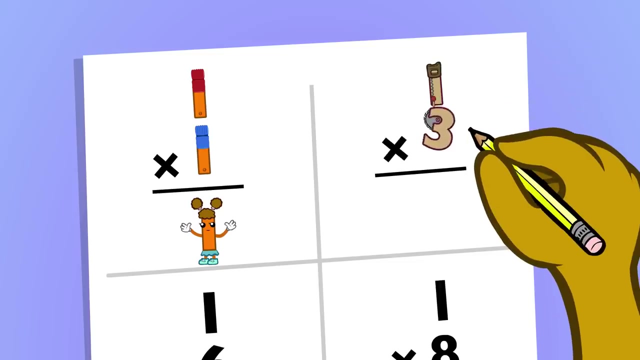 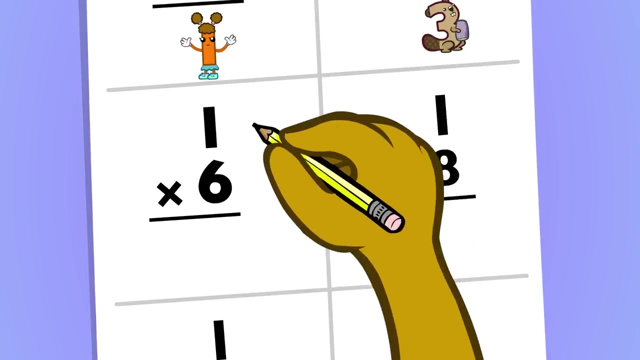 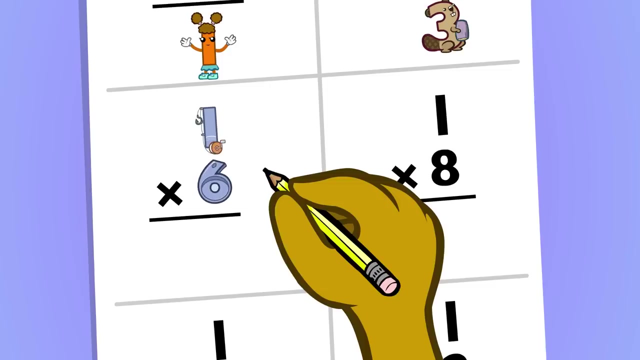 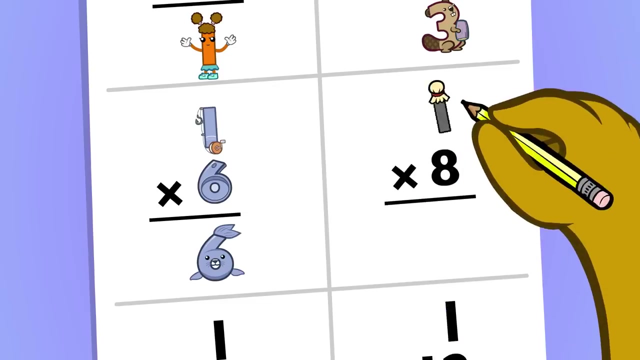 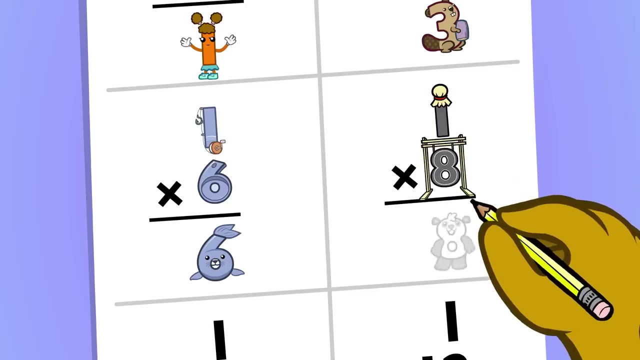 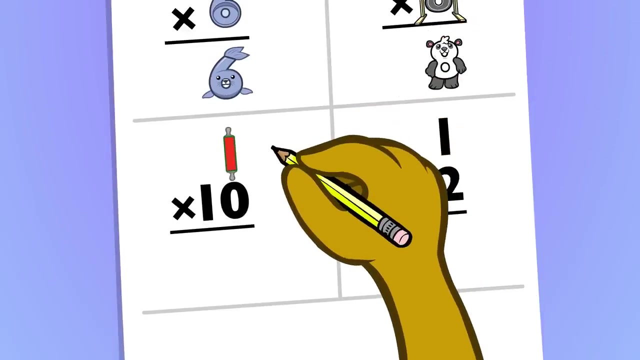 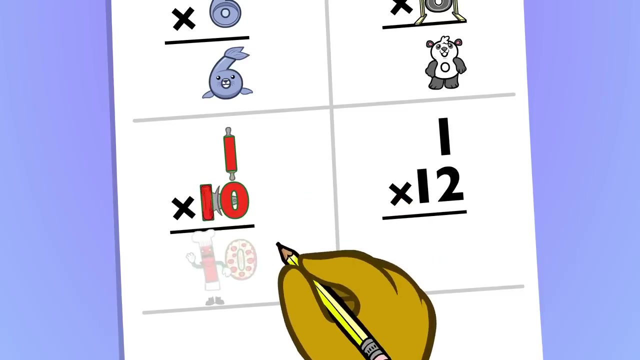 One times twelve equals twelve. One times twelve equals twelve. One times one equals one. One. One times three equals three. One times six equals six. One times eight. One times nine equals eight. One times ten equals ten. 1 times 12 equals 12.. 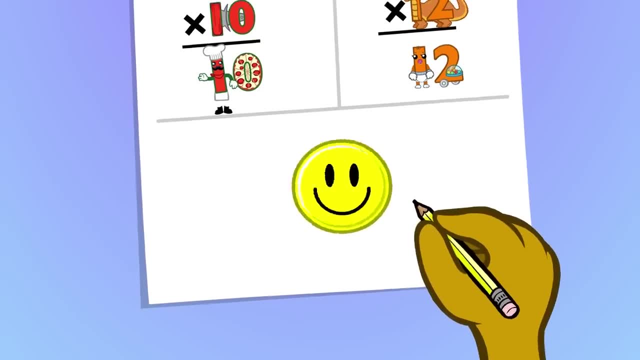 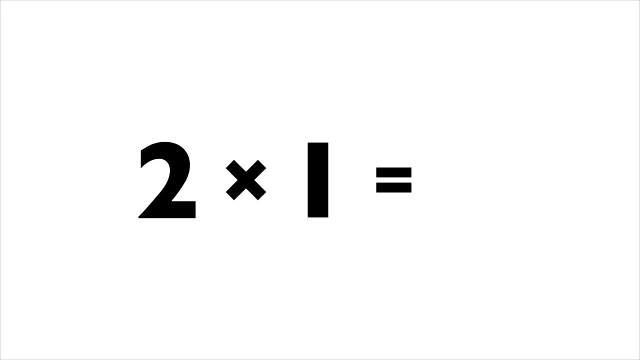 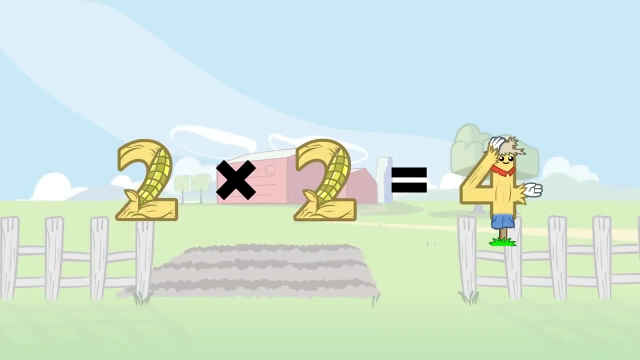 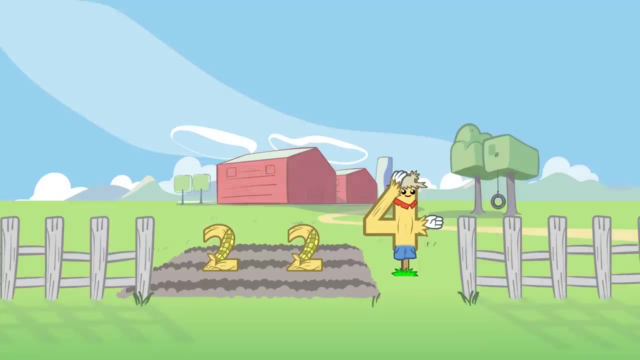 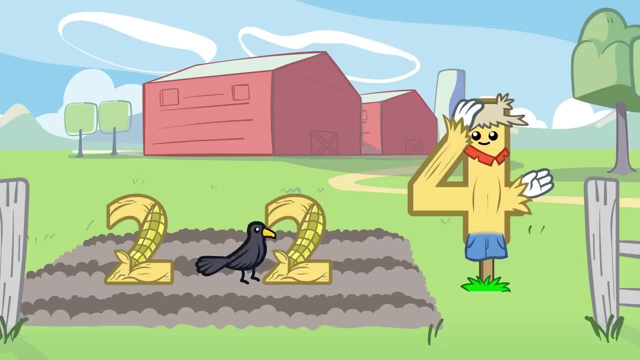 2 times 1 equals 2.. 2 times 1 equals, 2.. 2 times 2 equals. 2.. 2 times 2 equals 4.. 2 times 2 equals: 4.. 2 times 2 equals 4.. 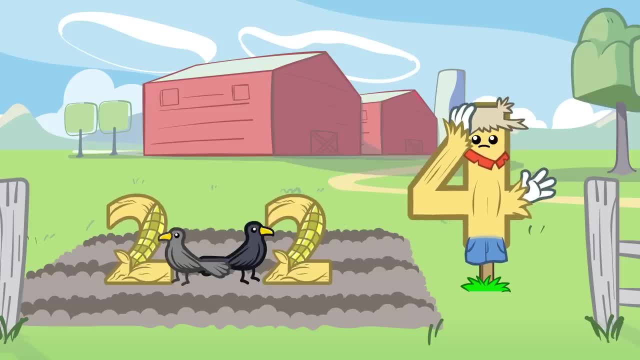 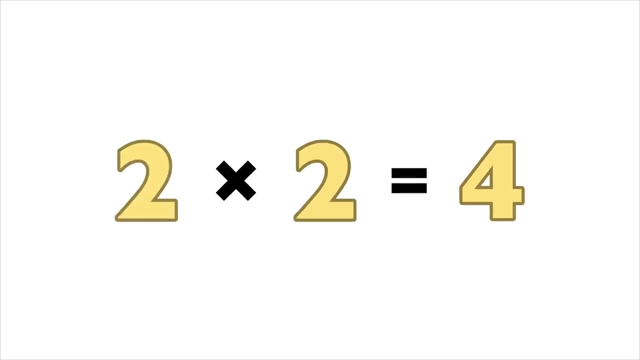 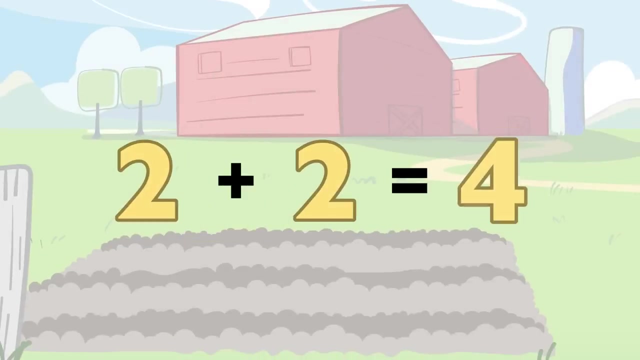 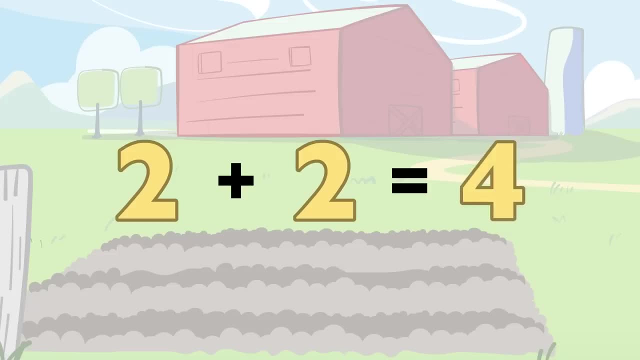 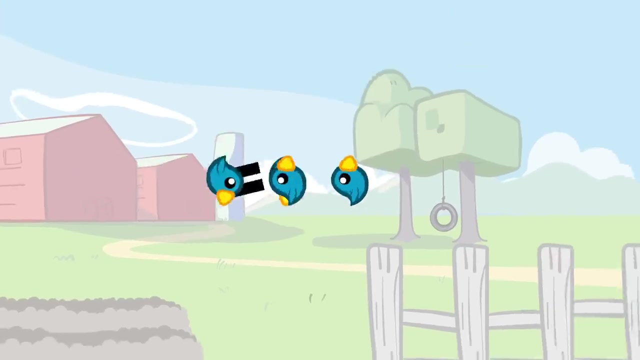 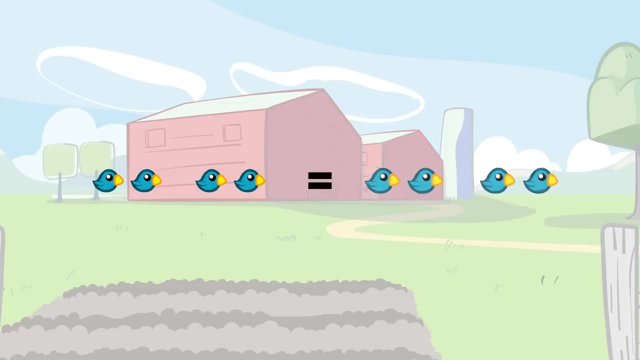 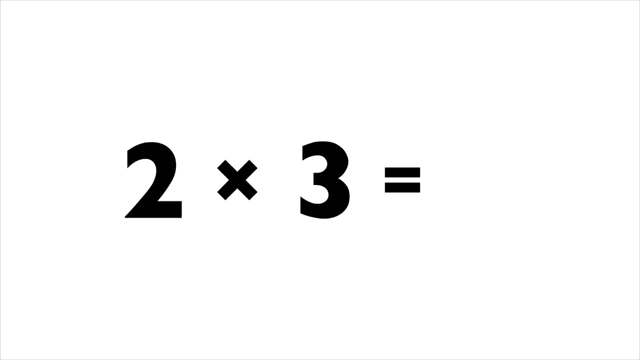 1, 2 twos equals 4.. 2 times 2 equals 4.. 2, 4 equals 4.. 4 equals 4.. 2 times 2 equals 4.. 2 times 3 equals. 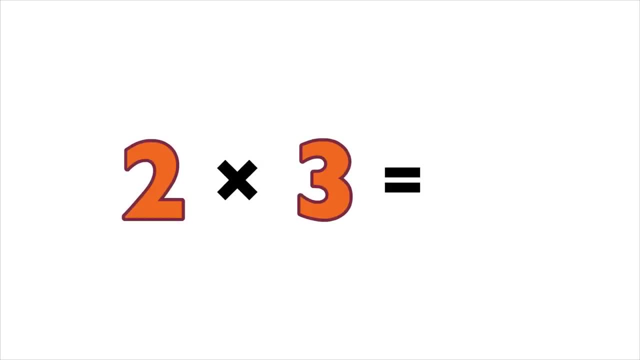 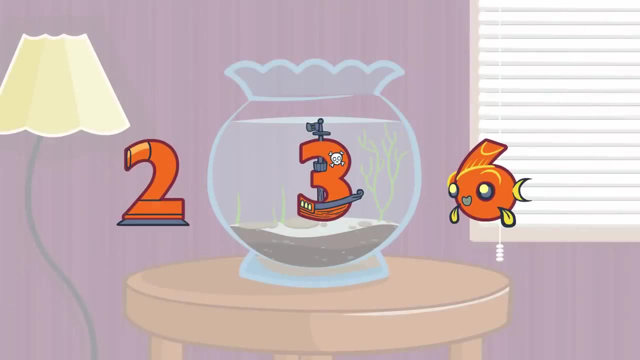 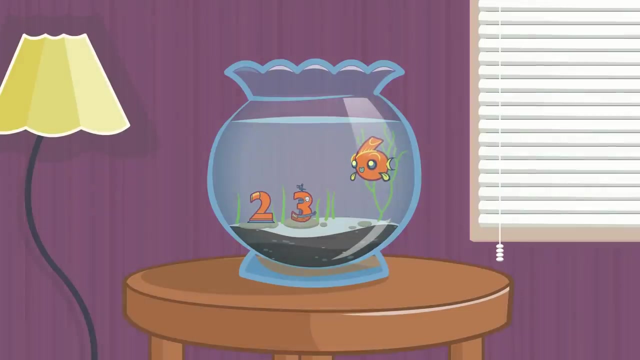 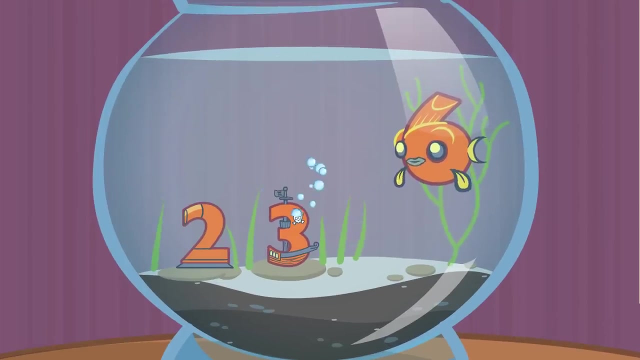 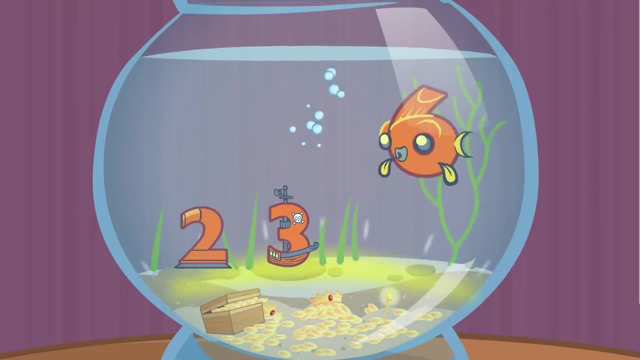 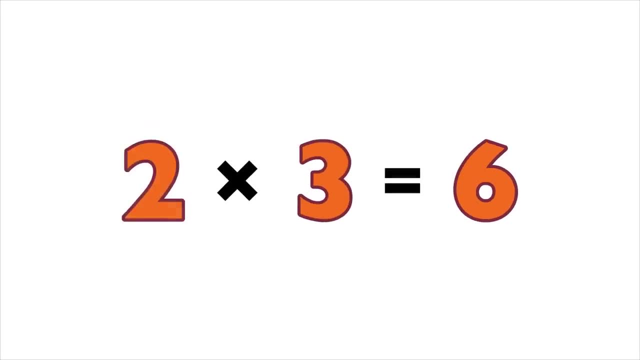 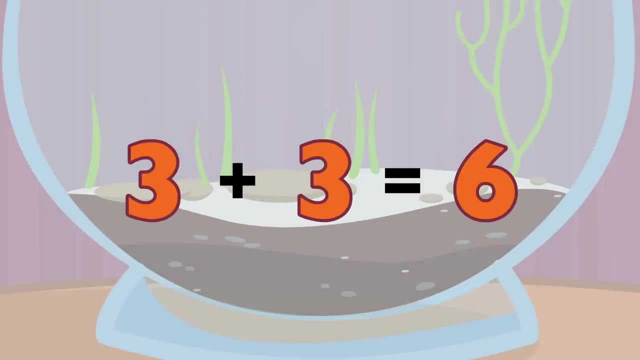 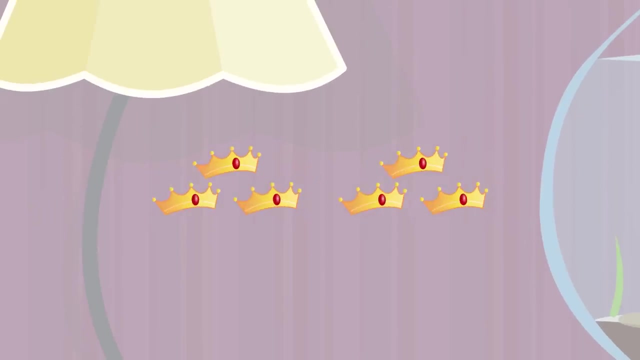 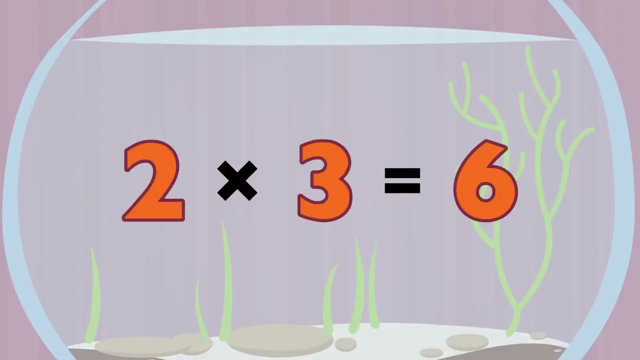 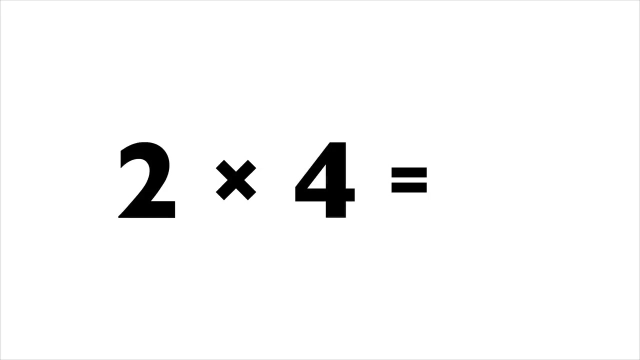 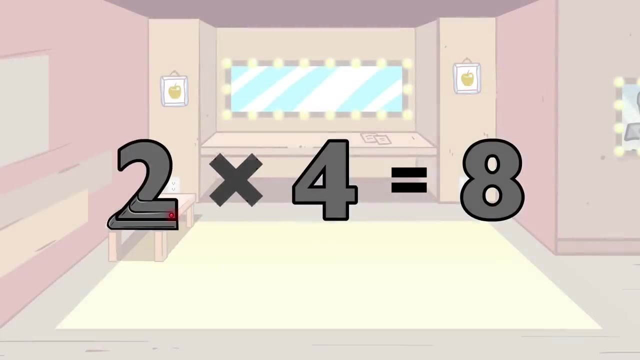 two times three equals six. two times three equals six. two threes equals six. one two threes equals six. two times three equals six, three. six equals six. six equals six. two times three equals six. two times four equals. two times four equals eight. two times four equals eight. 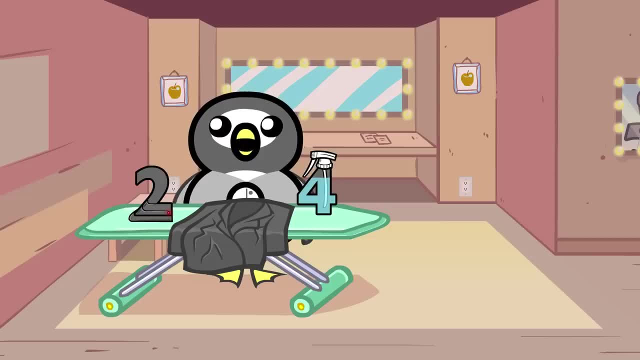 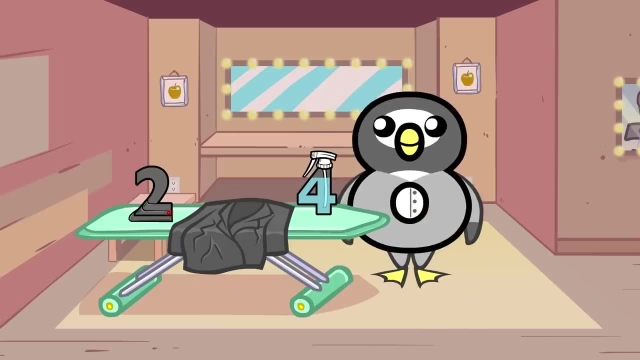 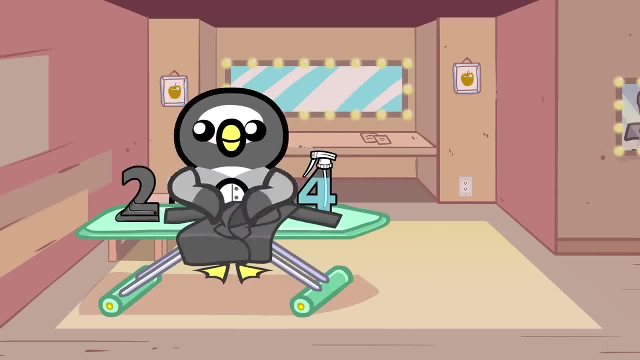 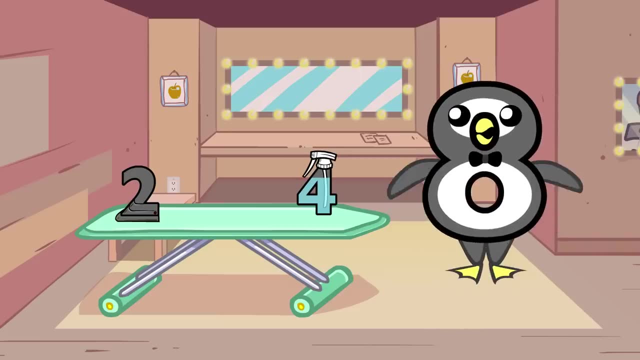 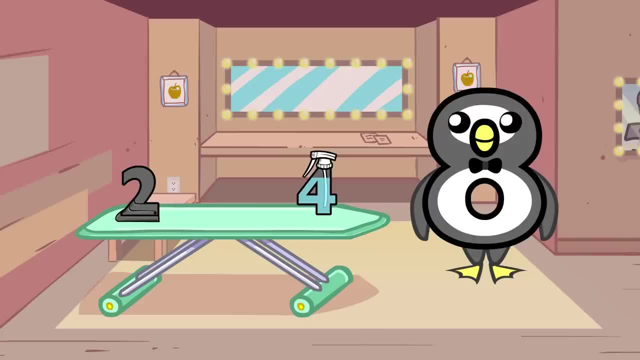 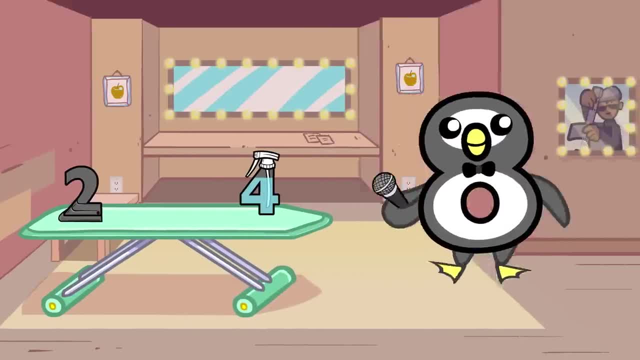 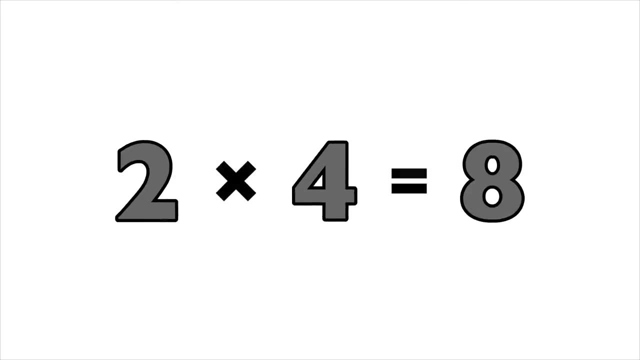 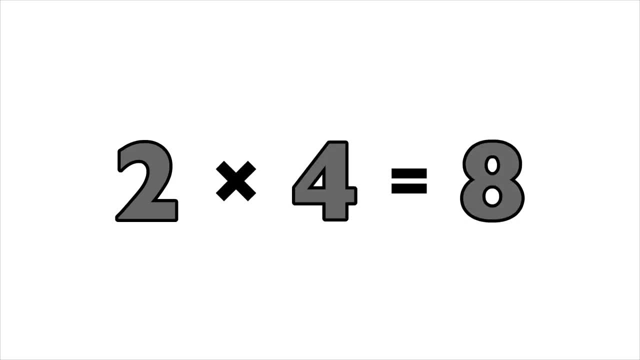 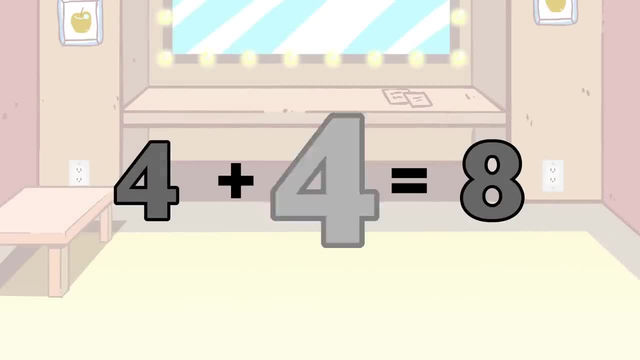 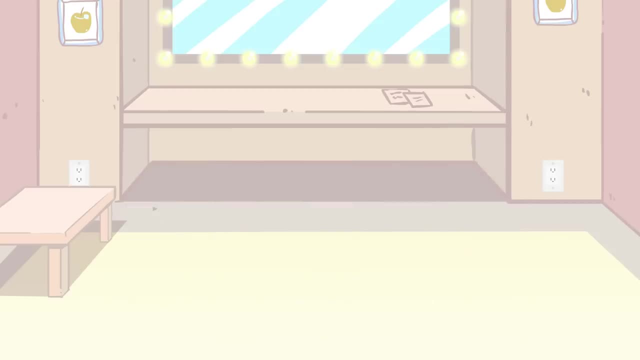 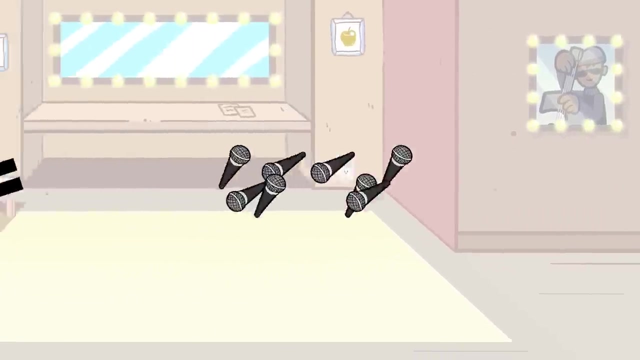 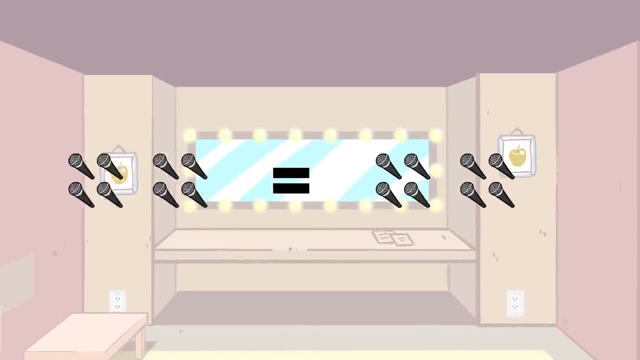 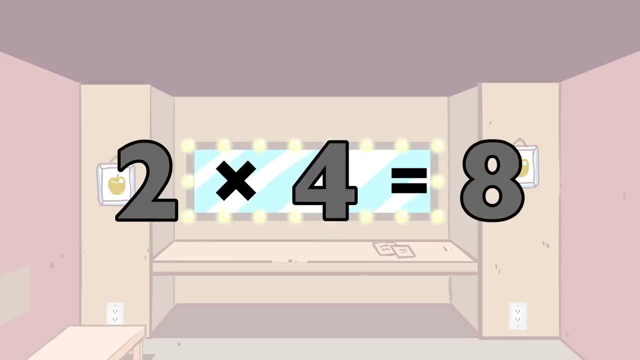 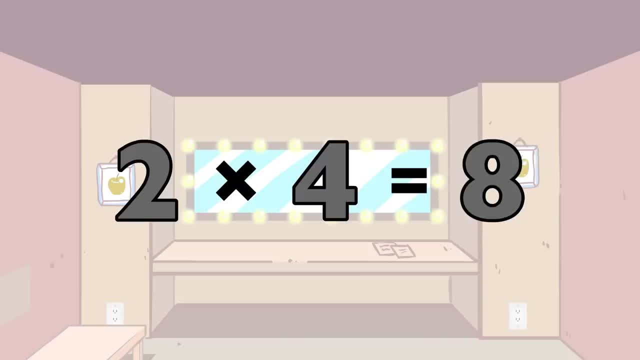 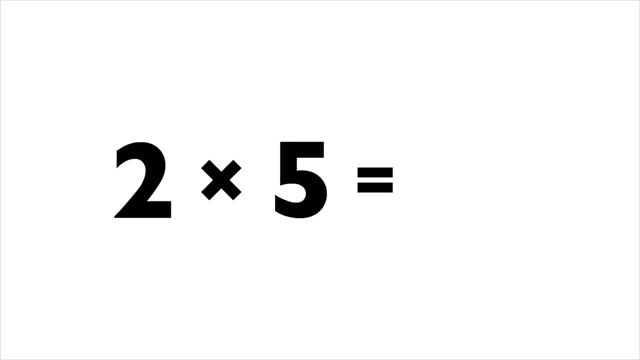 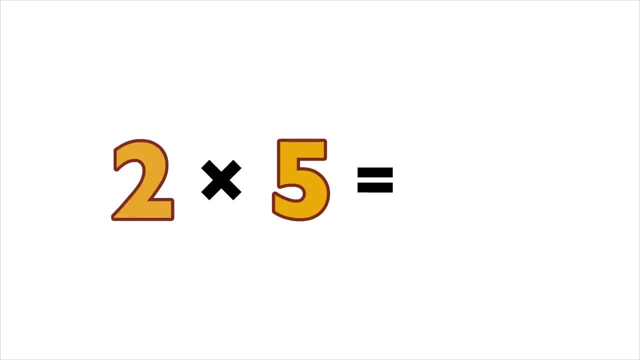 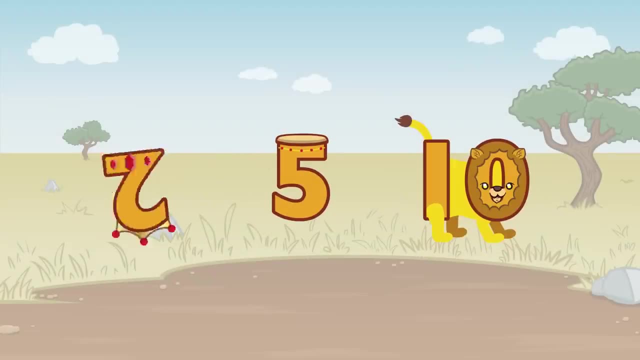 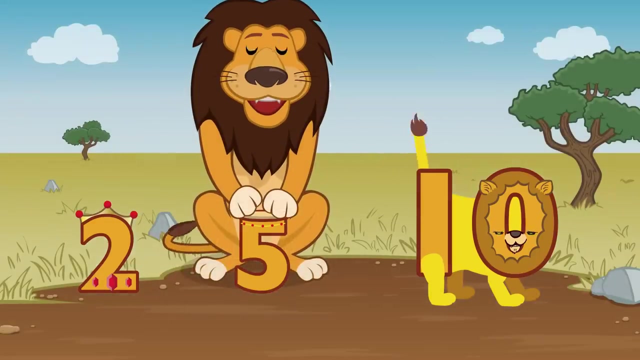 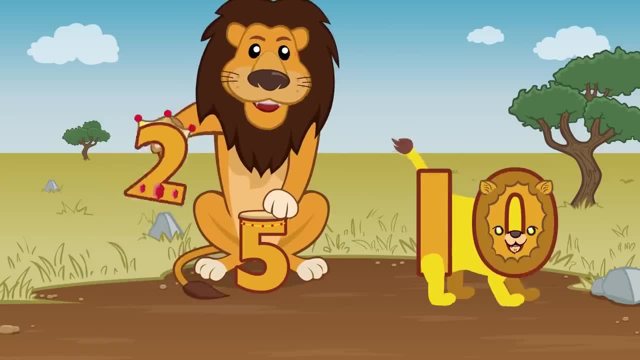 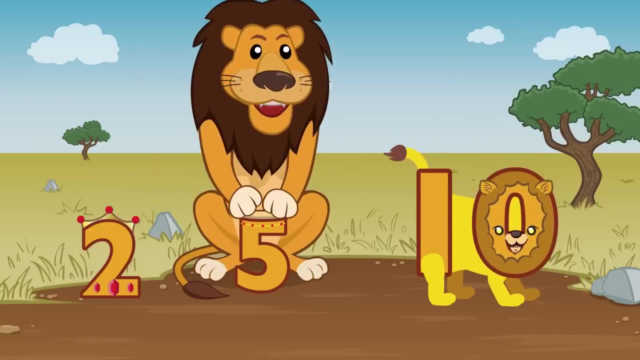 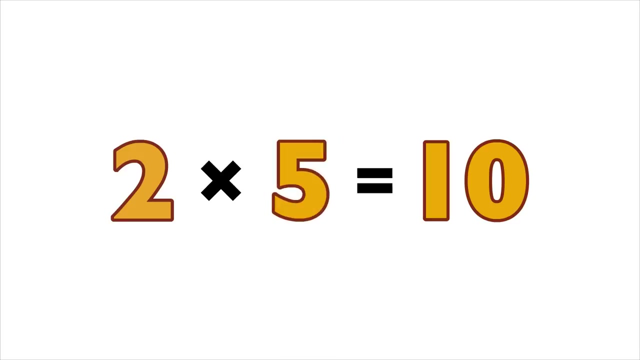 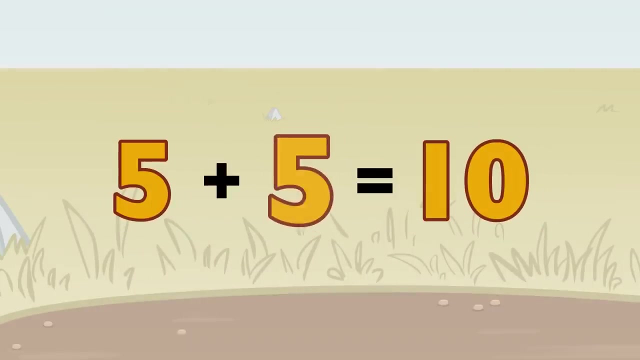 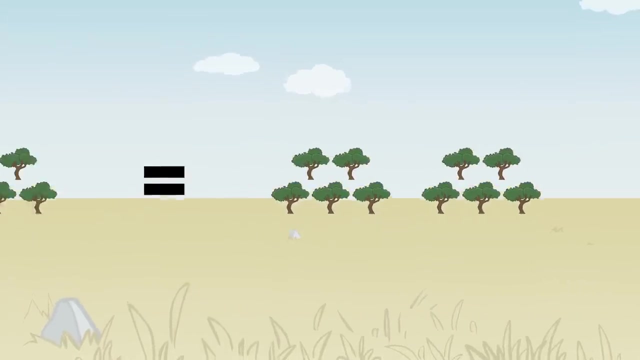 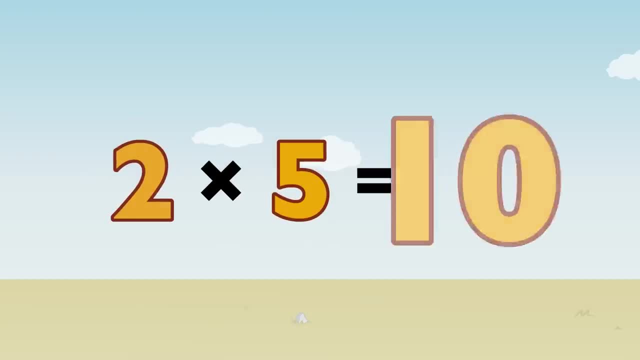 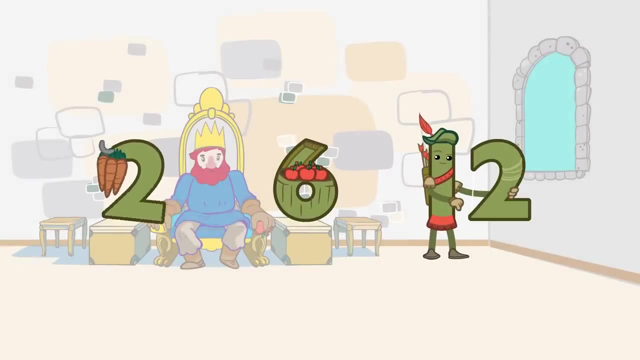 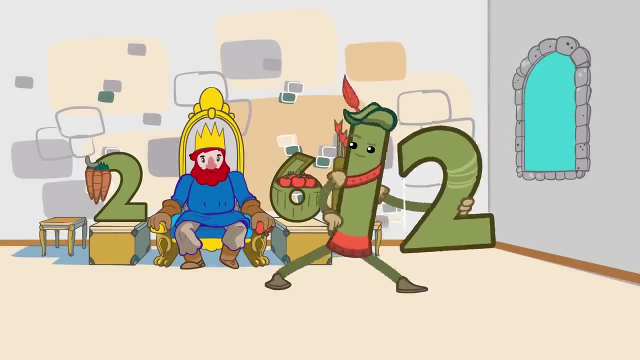 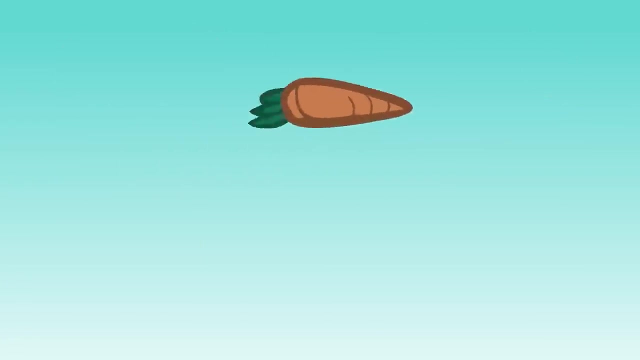 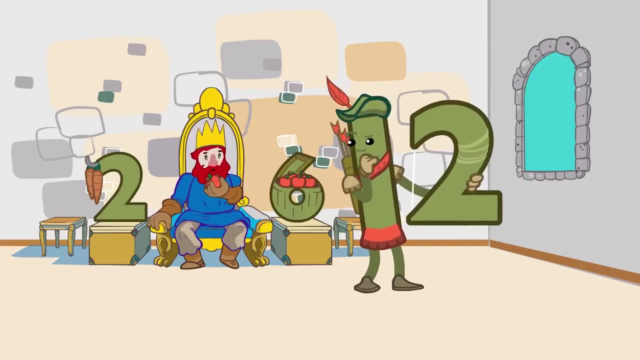 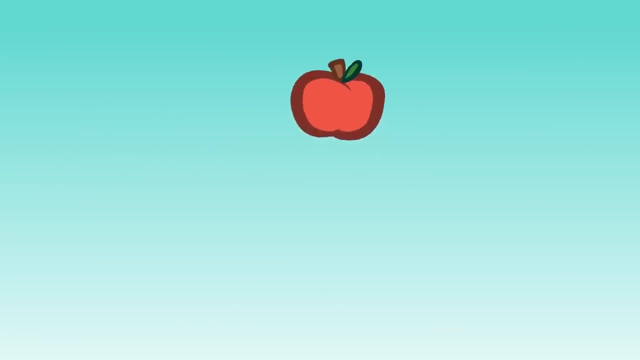 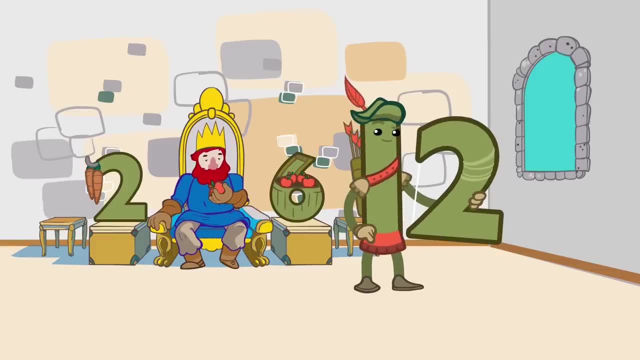 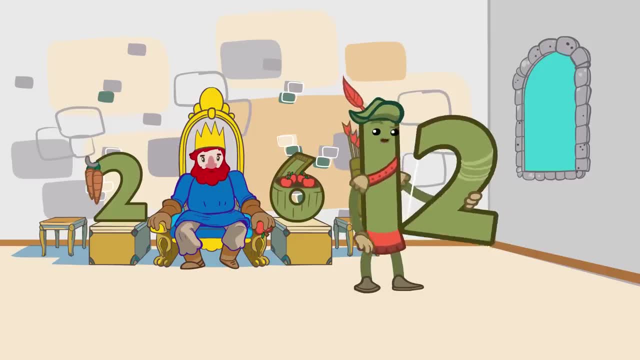 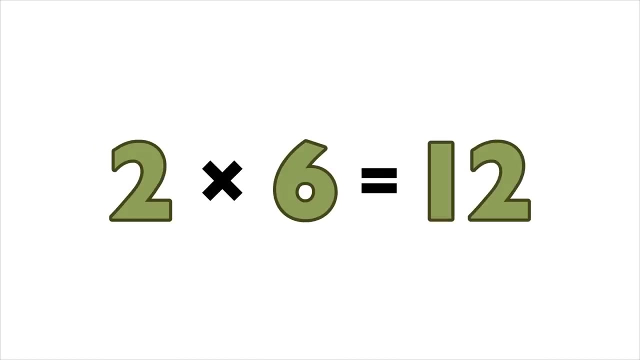 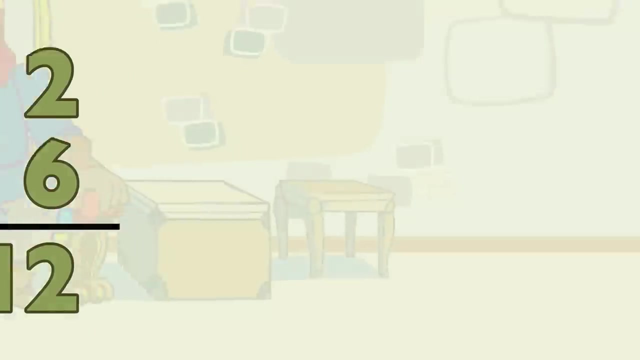 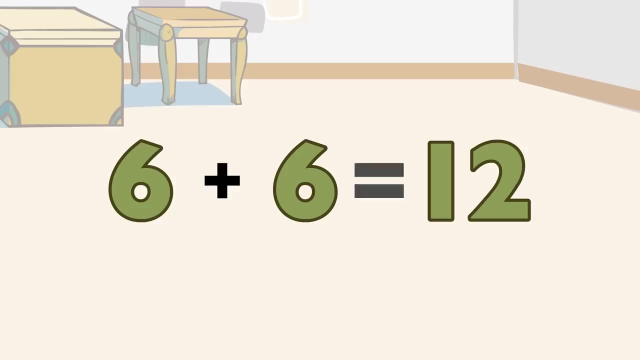 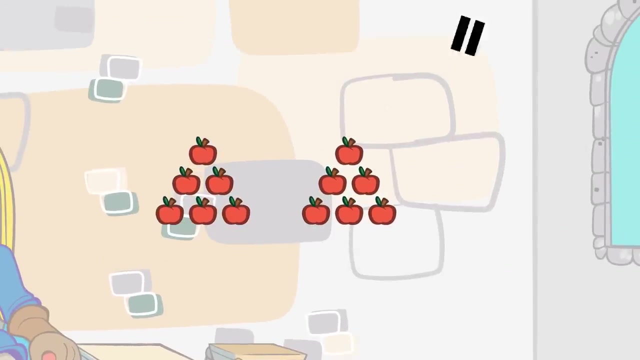 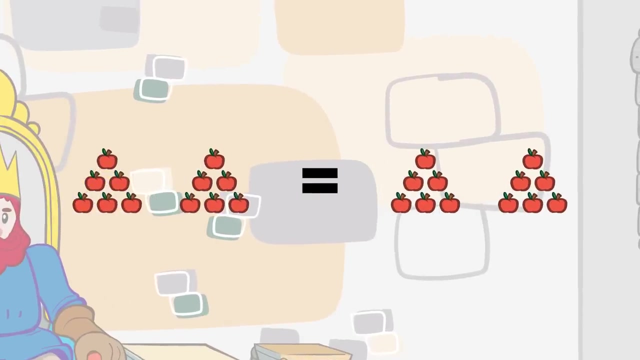 Ah, two times six equals twelve. Two times six equals twelve. Two times six equals twelve. Two sixes equals twelve. One two sixes equals twelve. Two times six equals twelve. Six twelve equals twelve. Twelve equals twelve. Two times six equals twelve. 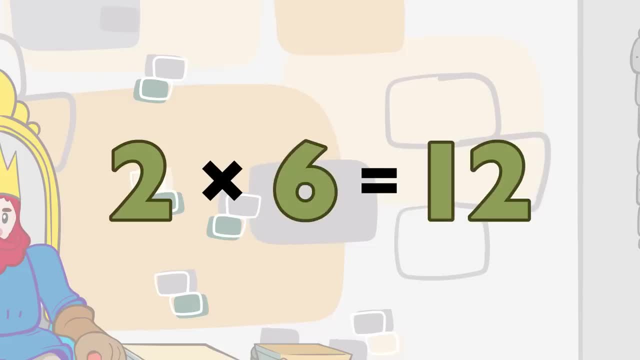 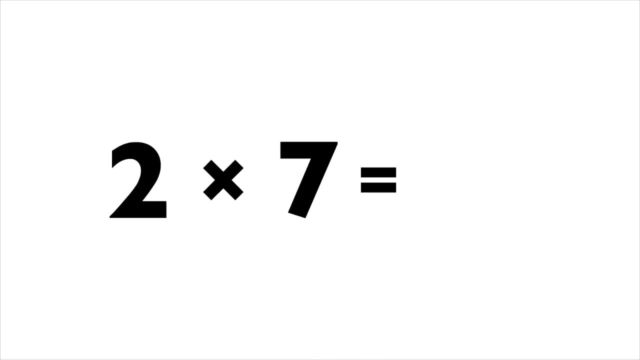 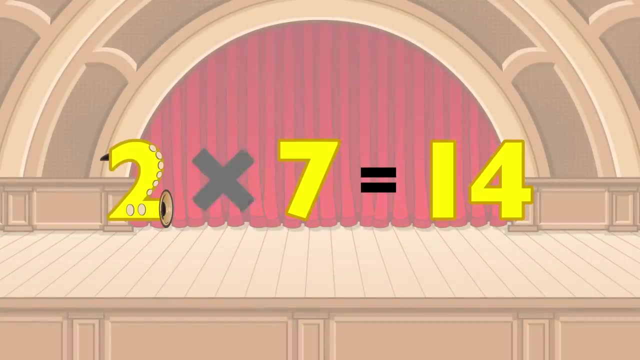 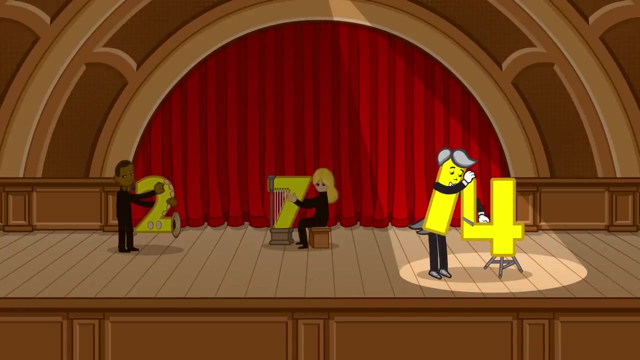 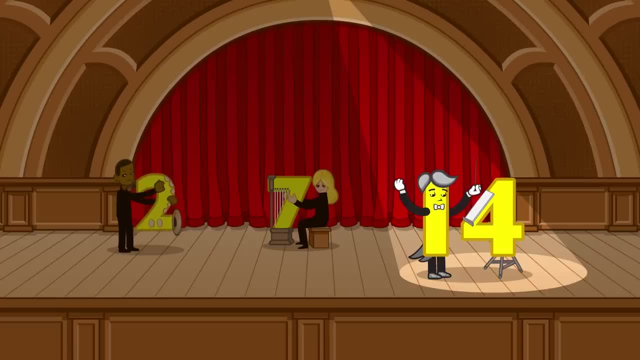 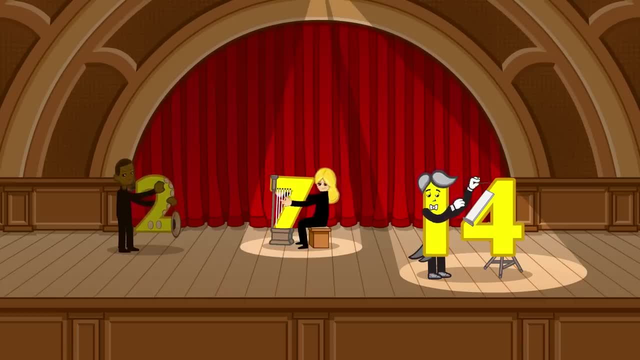 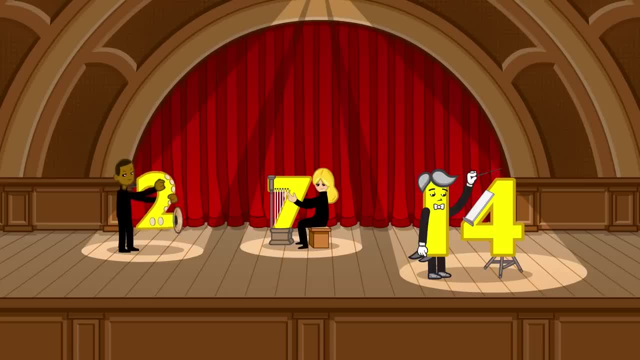 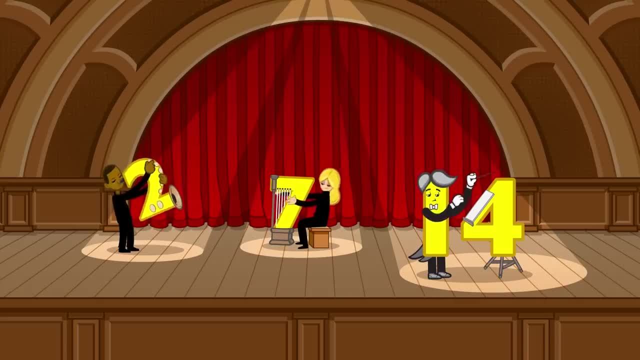 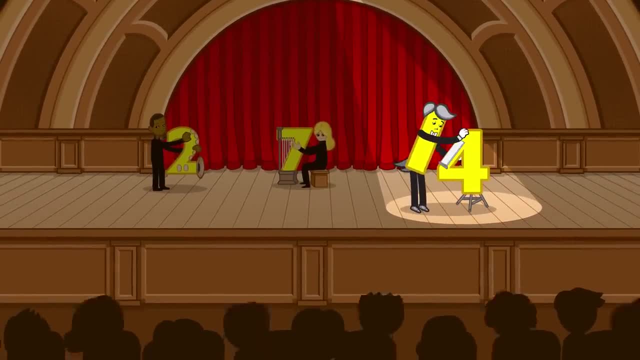 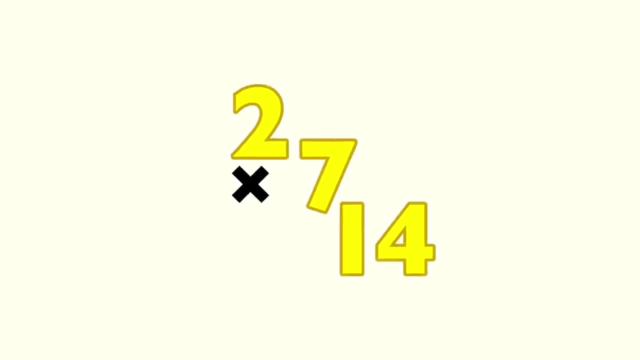 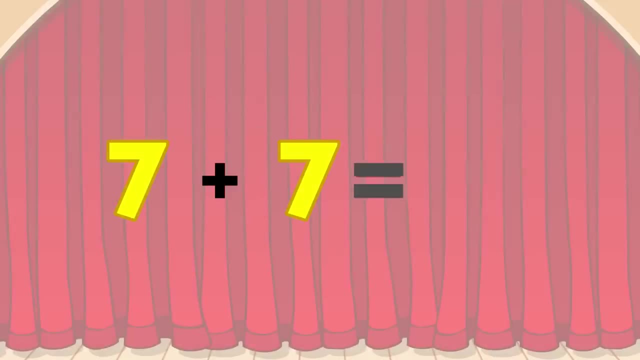 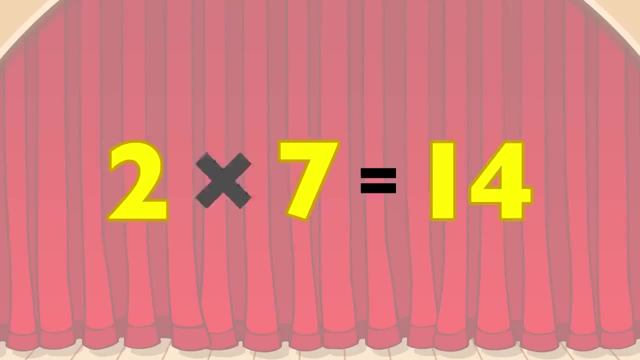 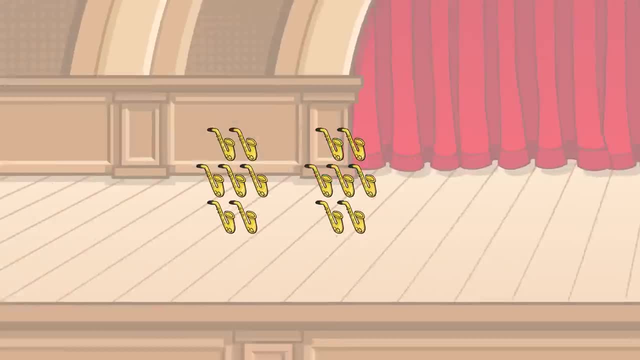 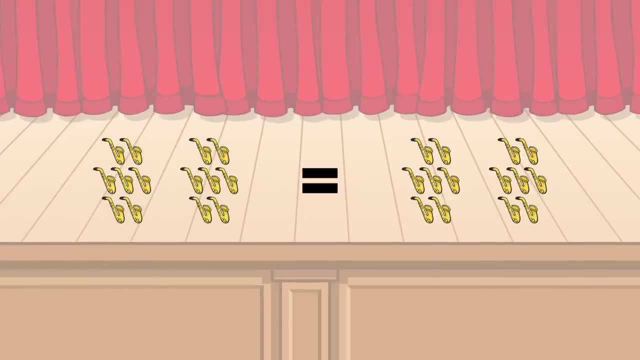 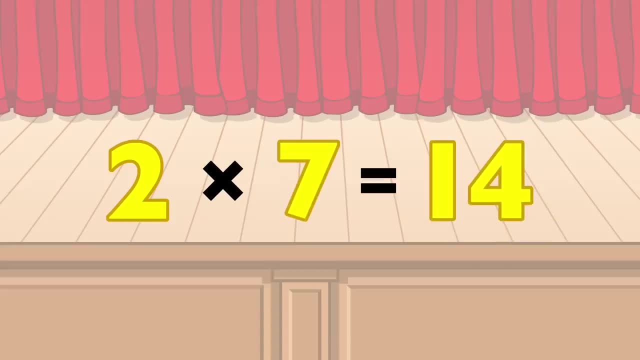 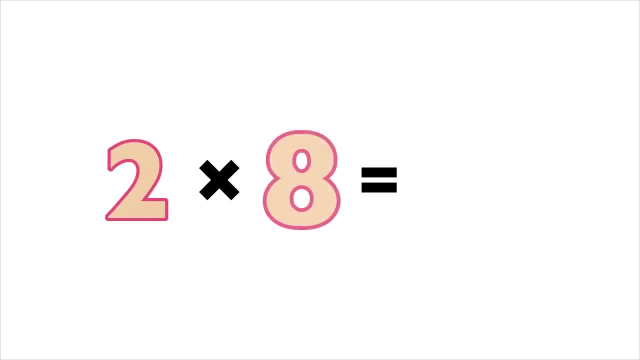 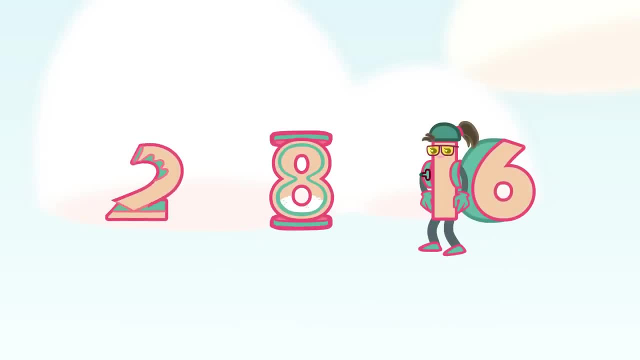 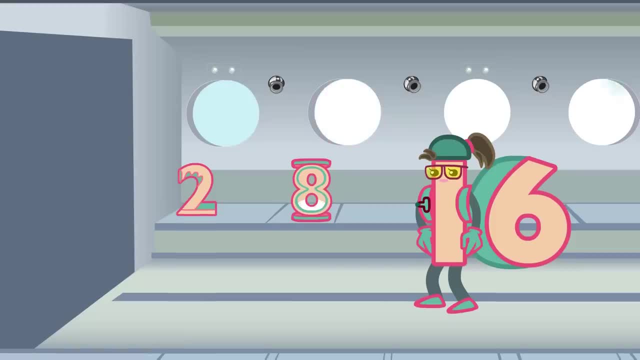 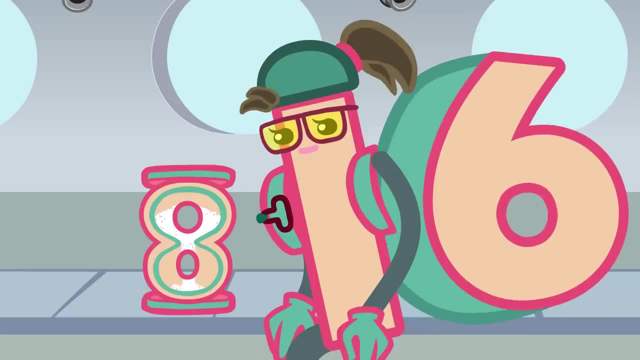 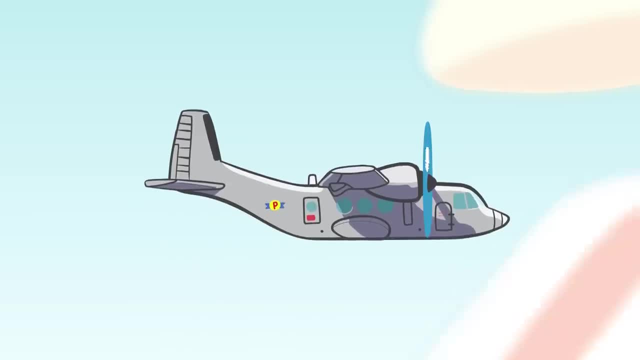 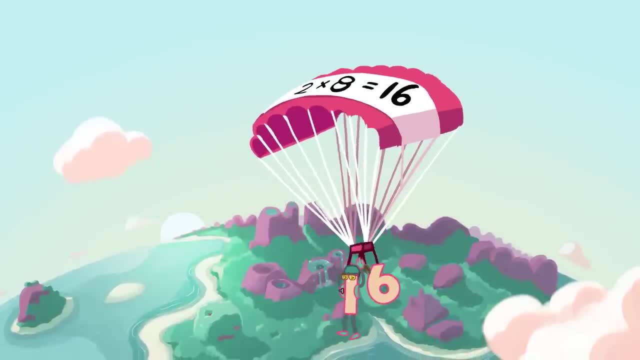 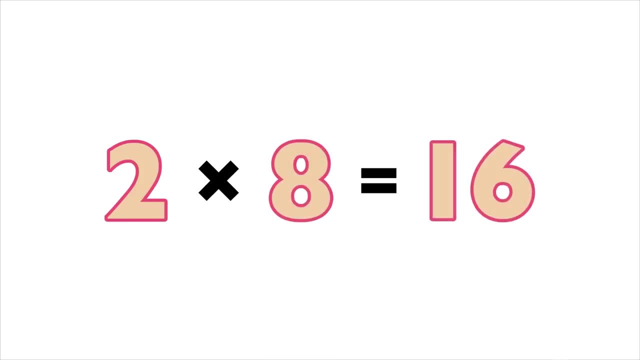 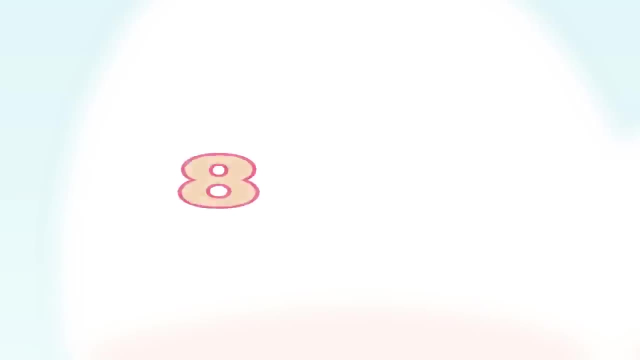 Two times seven equals sixteen. Two times seven equals sixteen. Two times seven equals sixteen. Two eights equals sixteen. Two eights equals sixteen One. two eights equals sixteen One. two eights equals sixteen One. two eights equals sixteen. 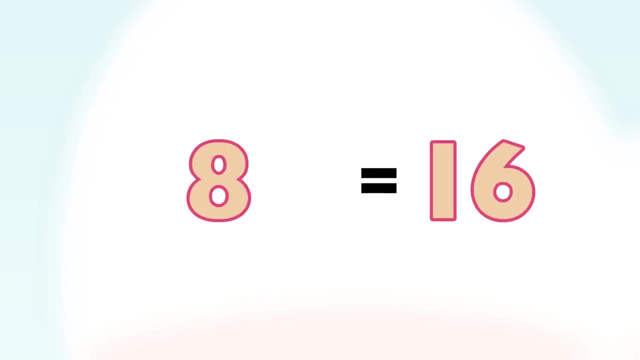 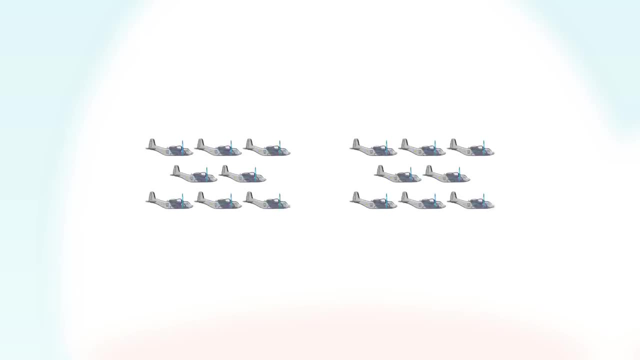 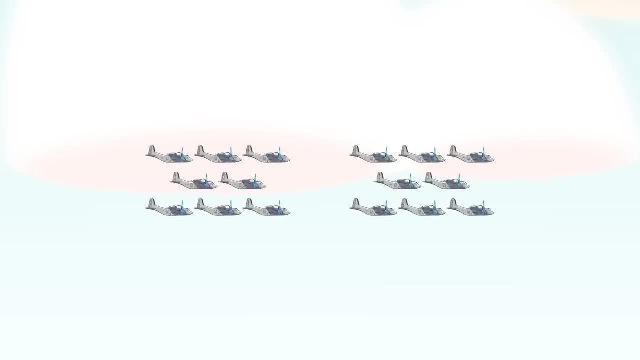 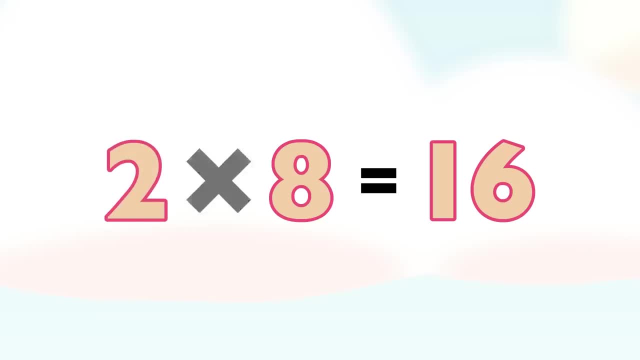 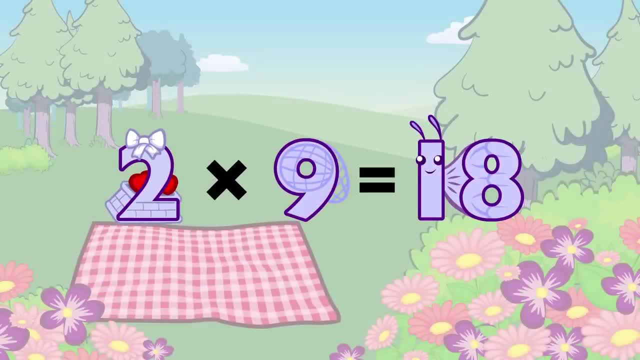 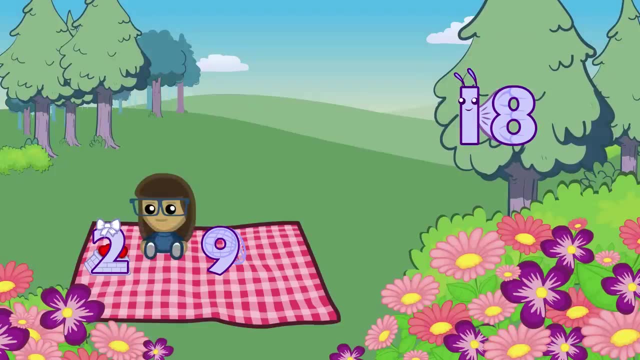 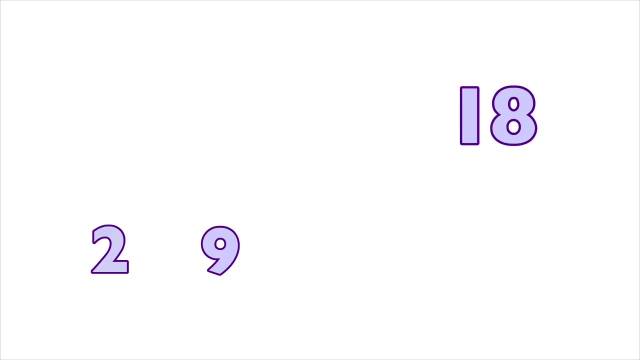 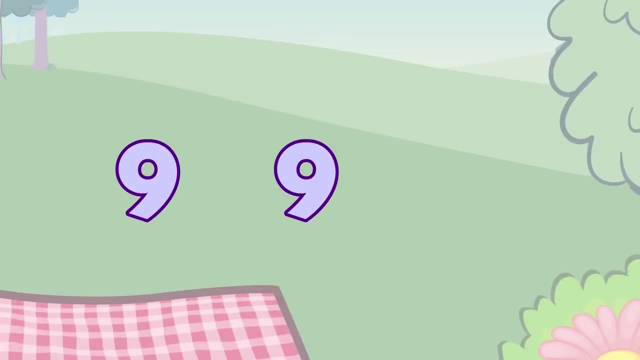 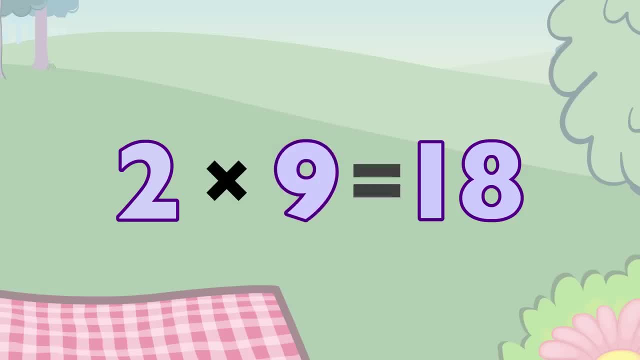 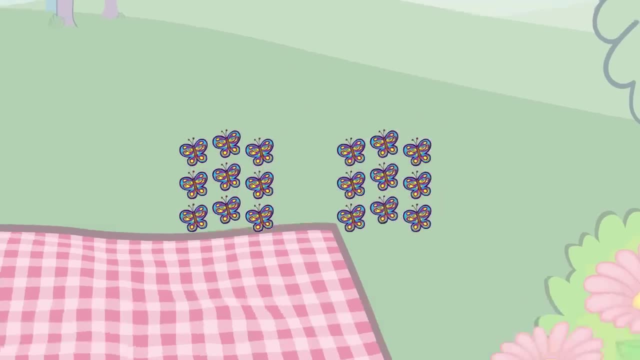 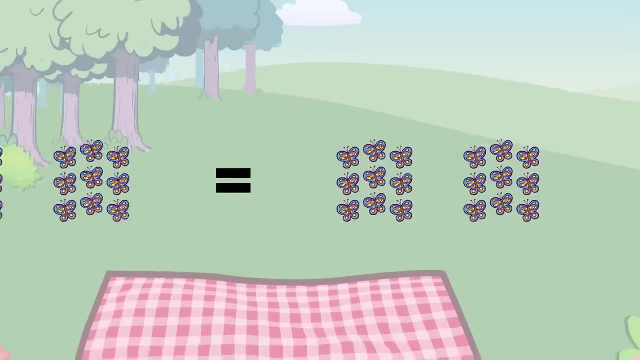 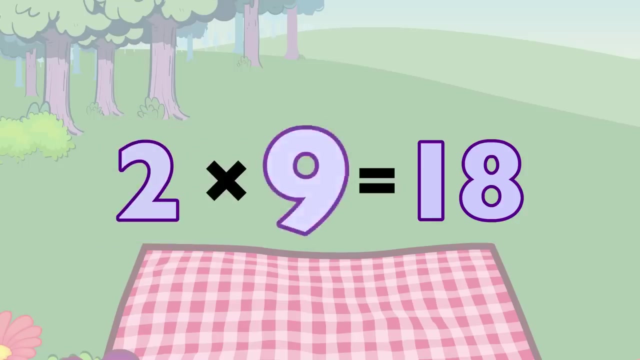 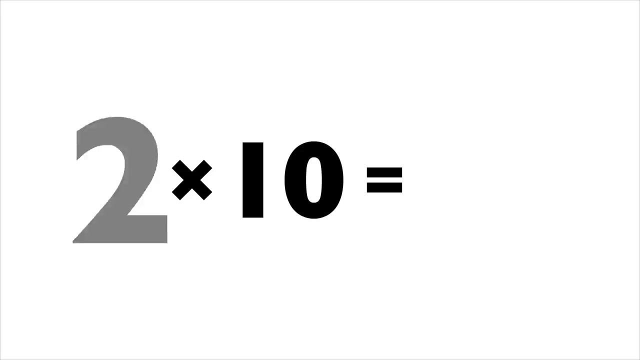 2 times 9 equals 18.. 9, 18 equals 18.. 18 equals 18.. 2 times 9 equals 18.. 2 times 10 equals. 2 times 10 equals 20.. 2 times 10 equals 20.. 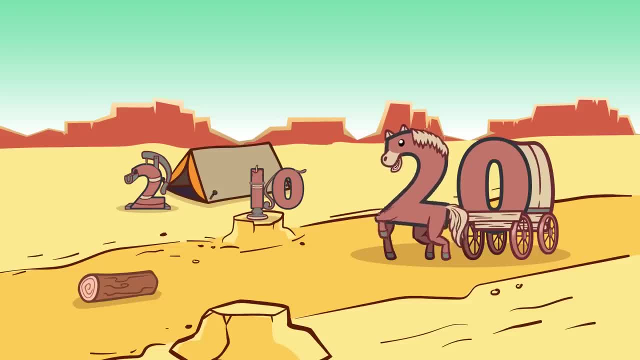 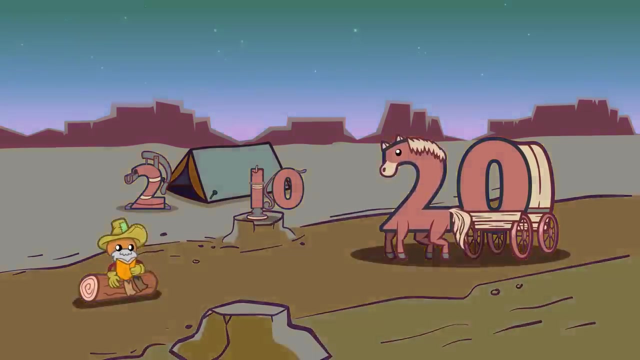 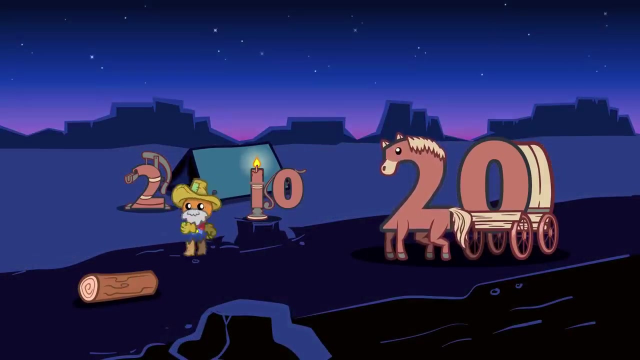 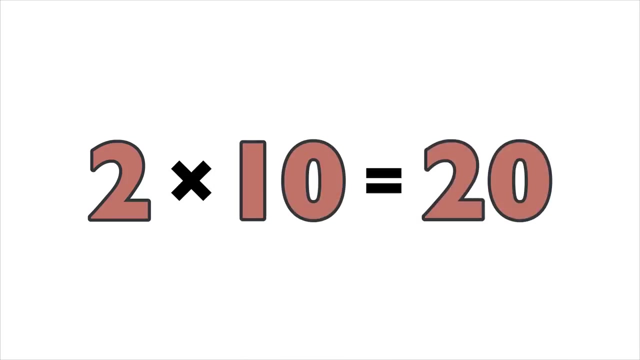 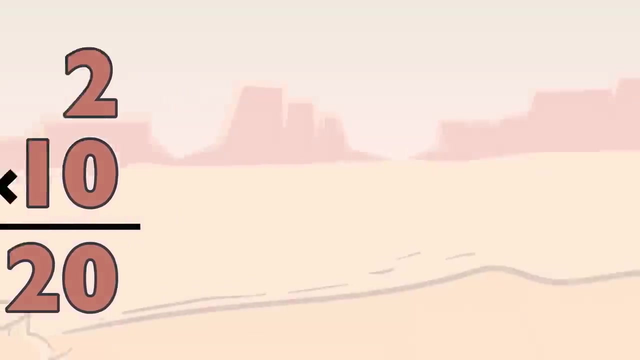 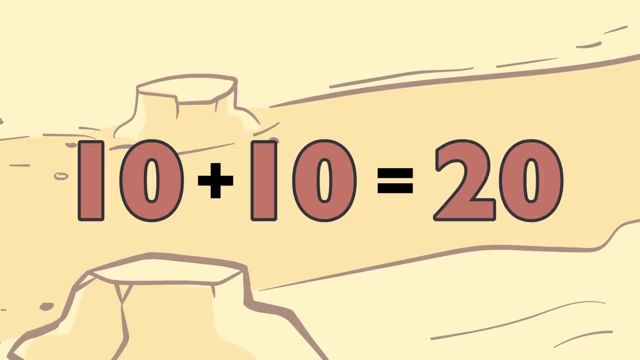 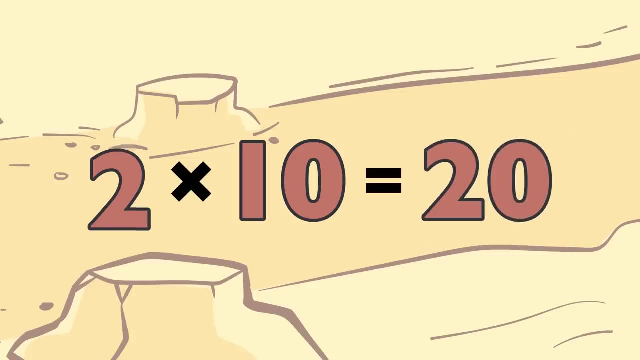 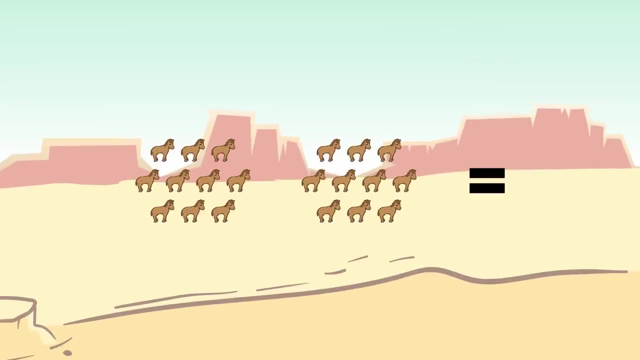 1, 2, 10s equals 20.. 2 times 10 equals 20.. 10, 20 equals 20.. 20 equals 20.. 2 times 10 equals 20.. 2 times 10 equals 20.. 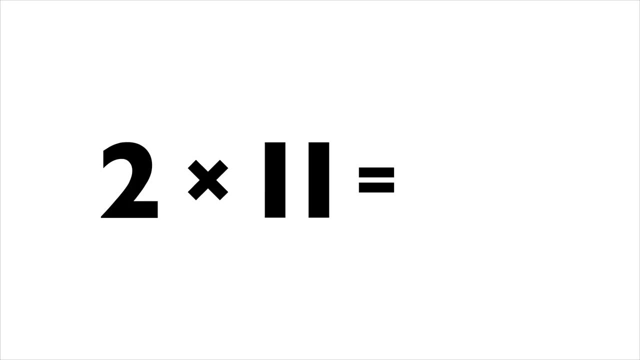 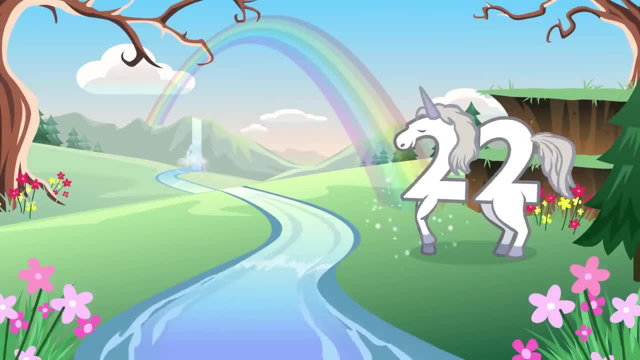 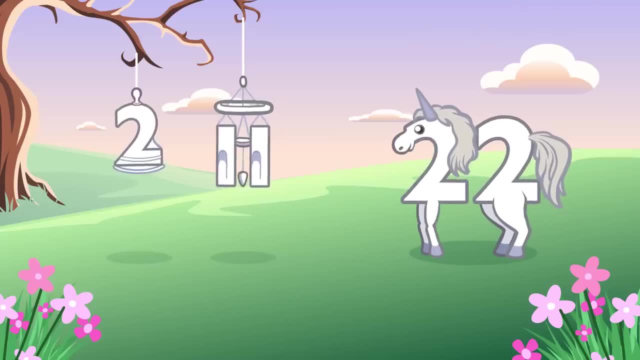 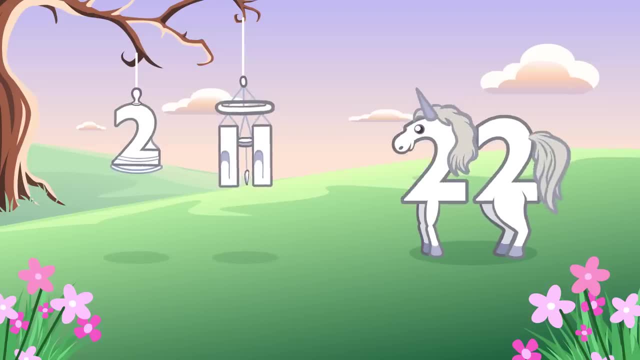 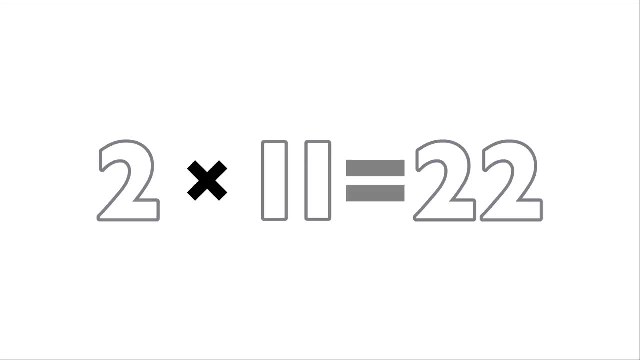 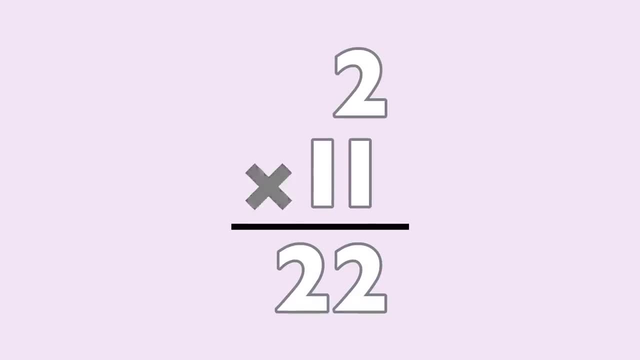 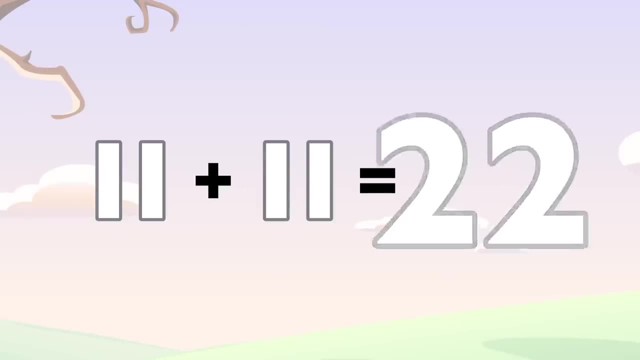 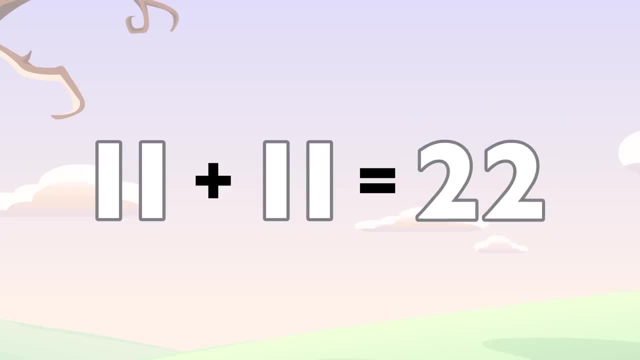 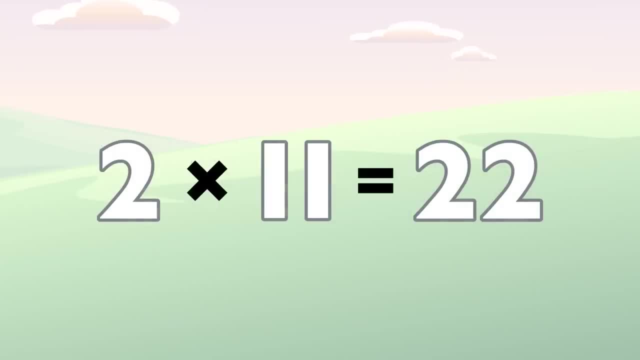 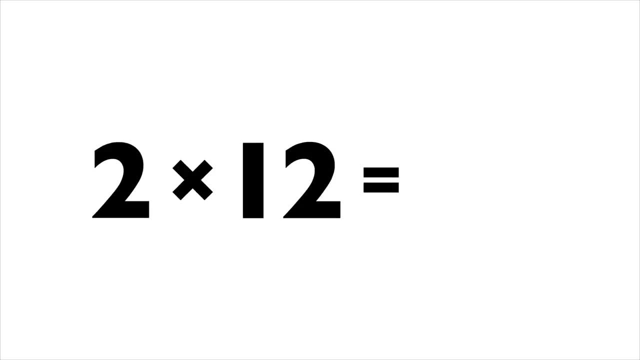 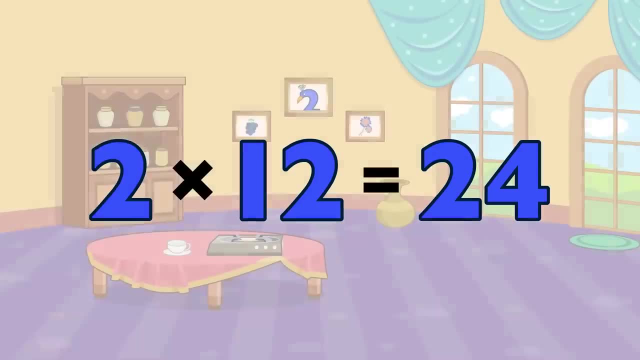 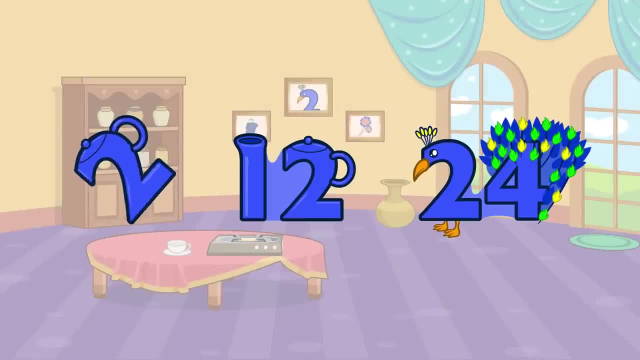 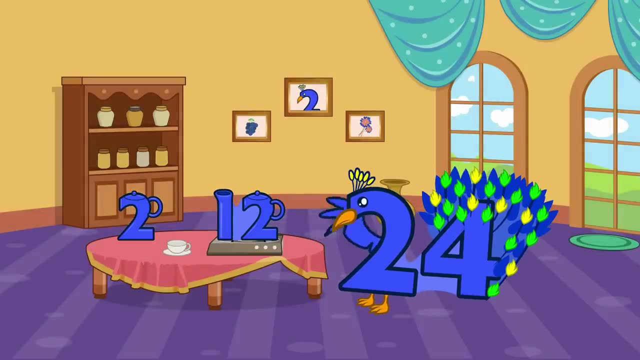 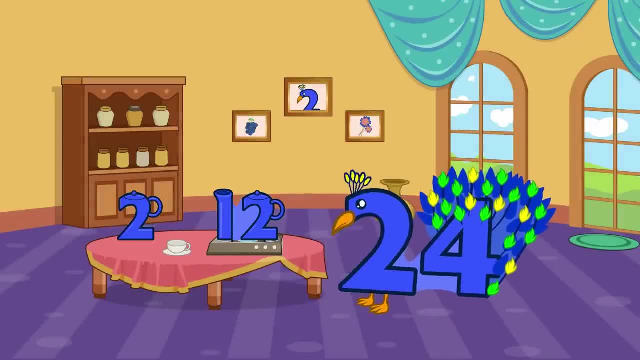 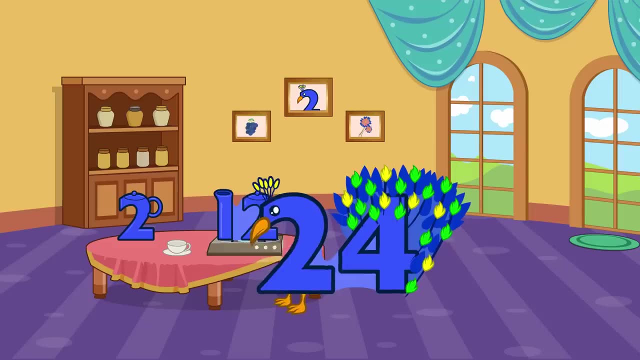 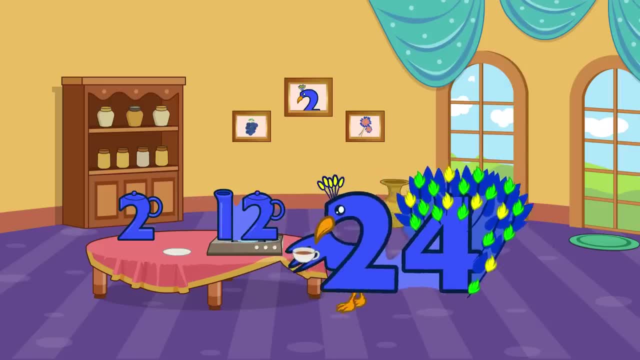 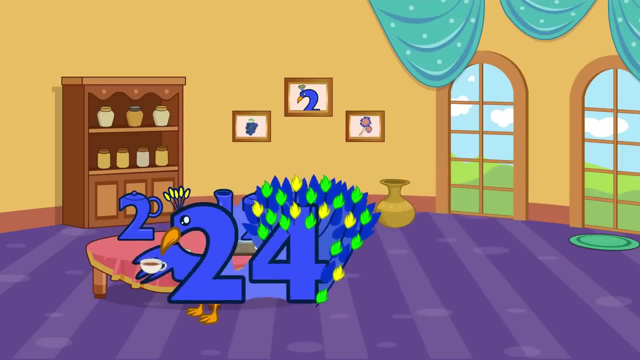 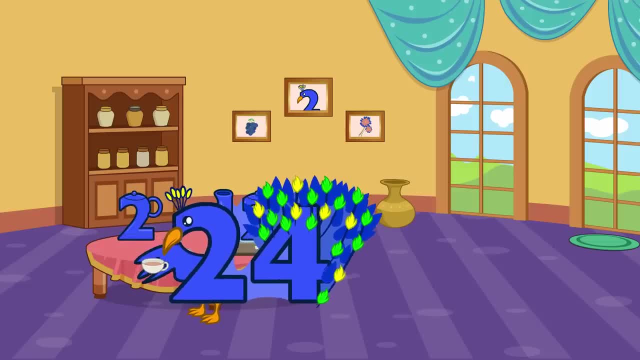 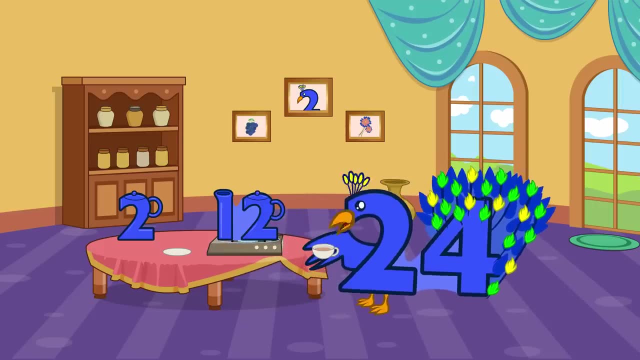 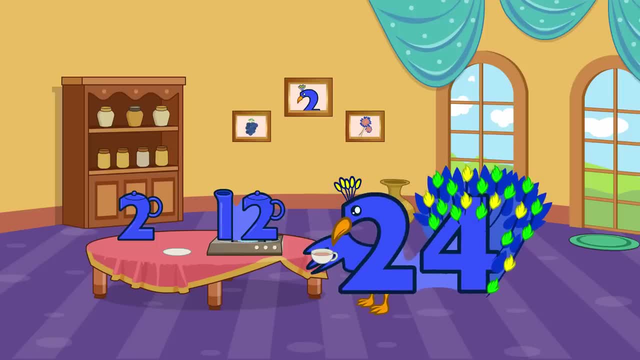 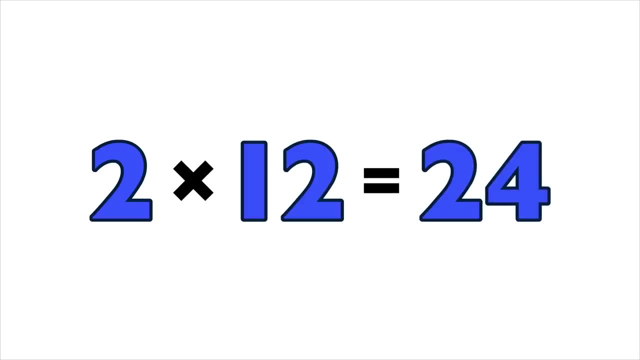 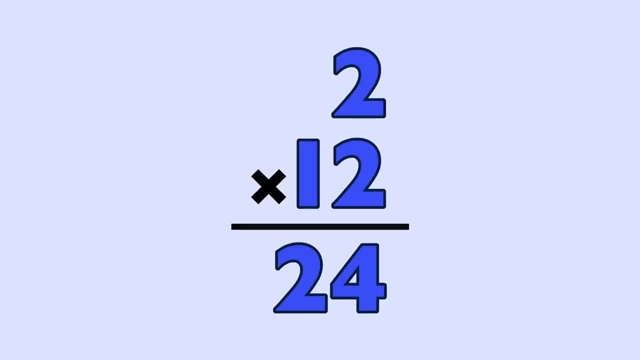 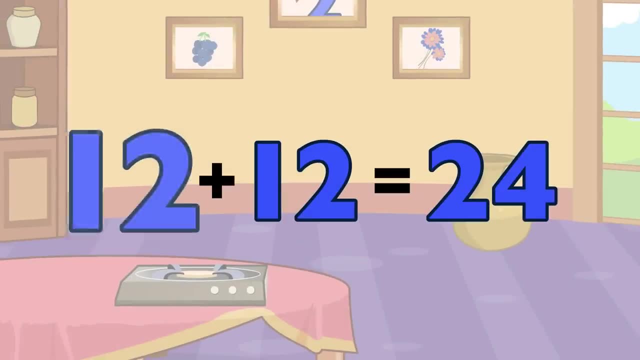 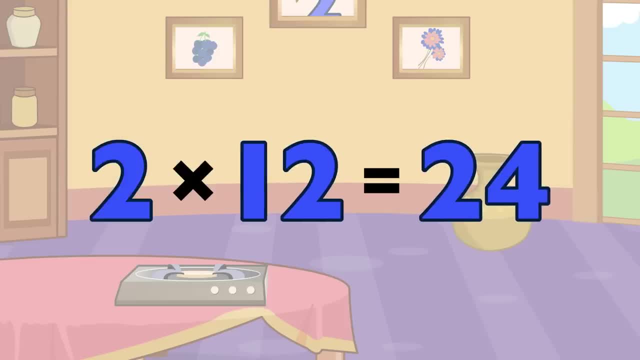 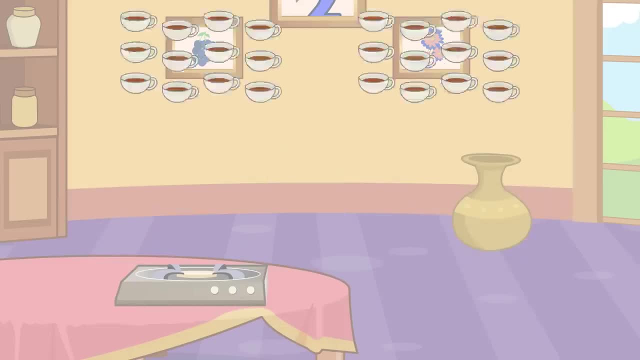 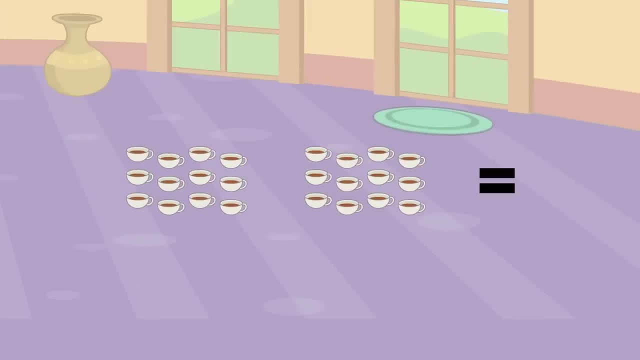 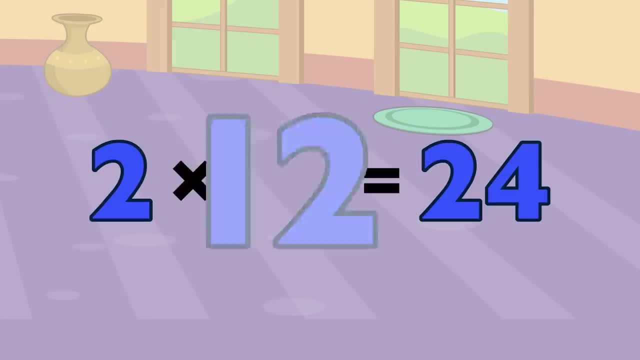 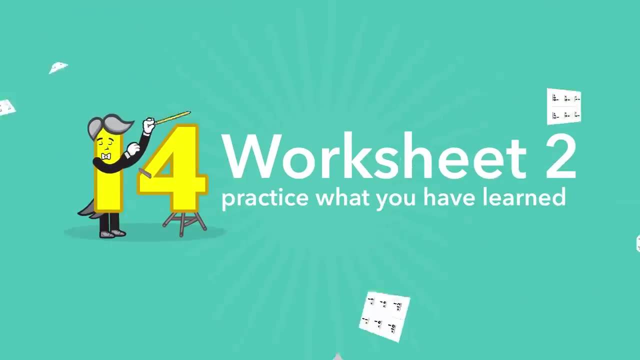 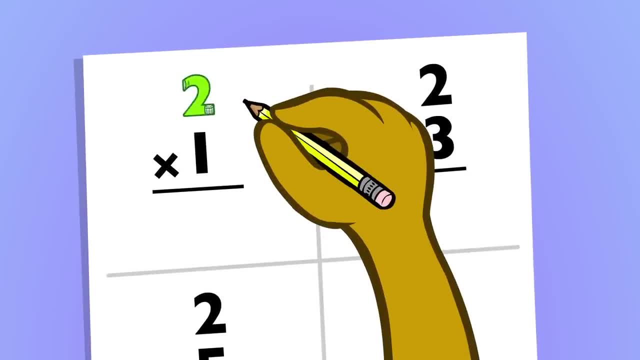 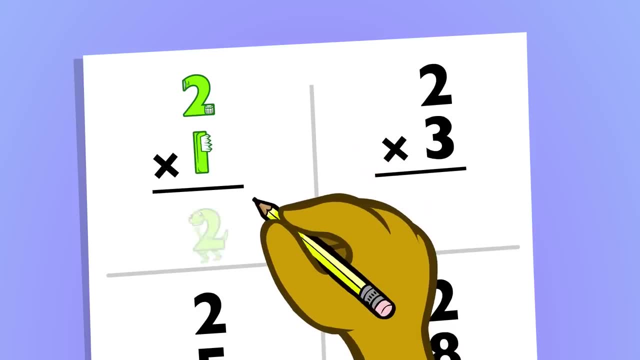 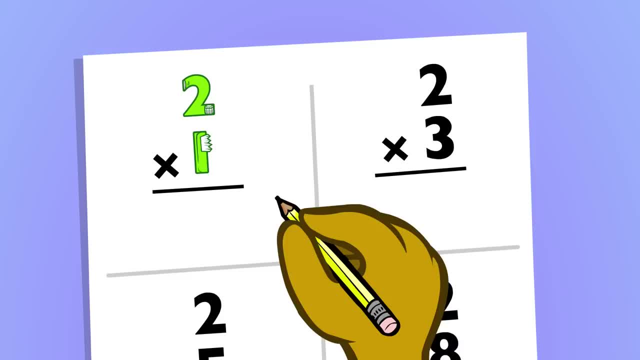 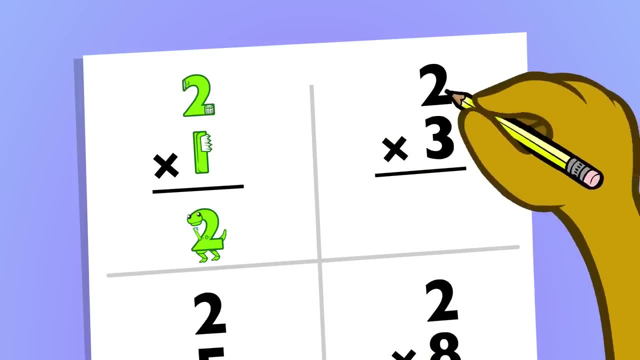 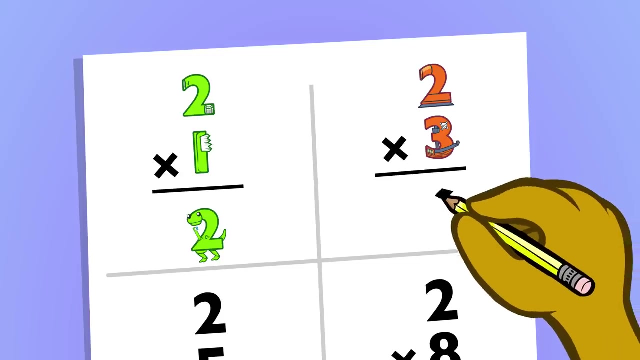 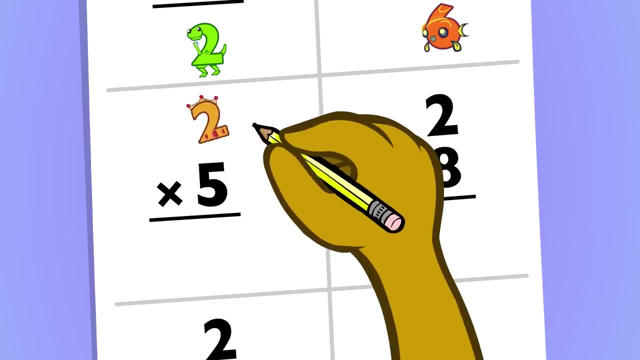 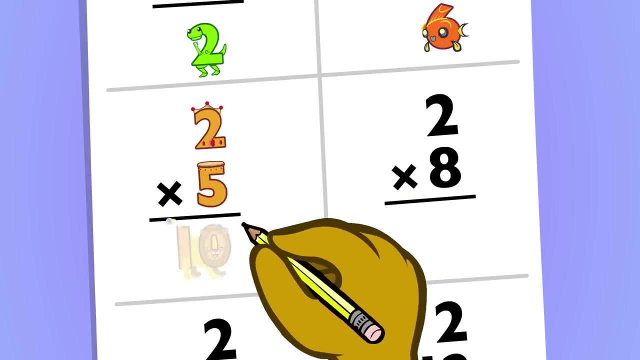 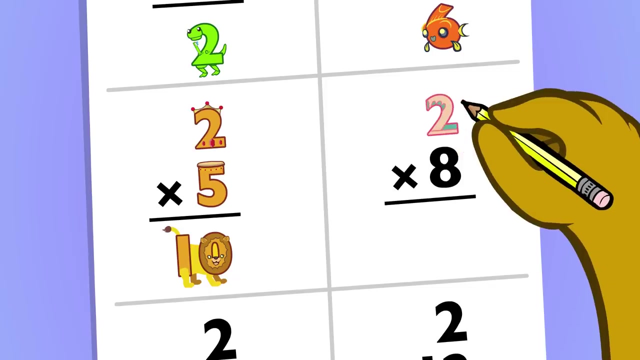 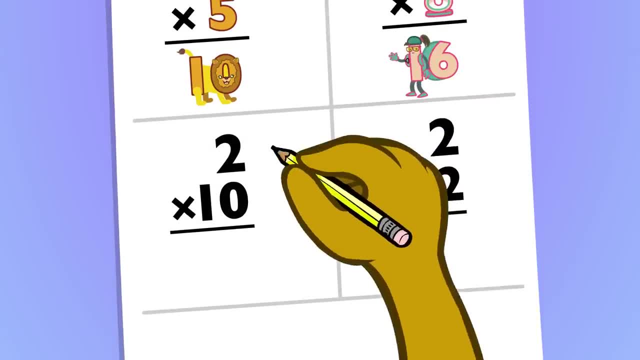 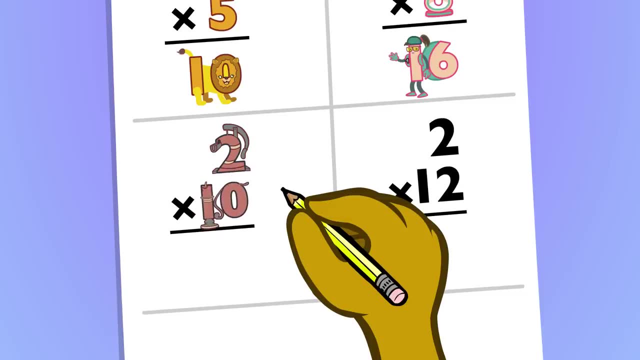 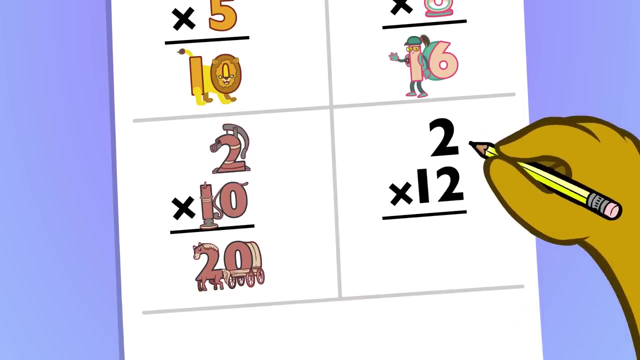 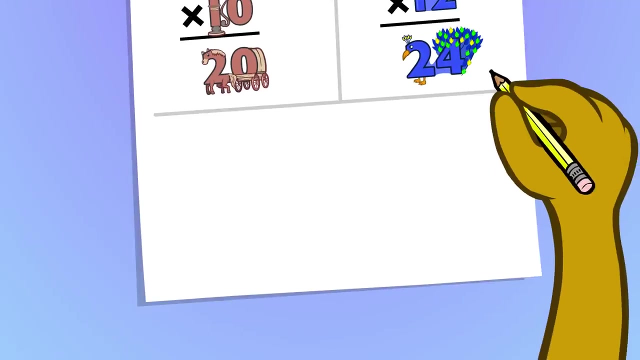 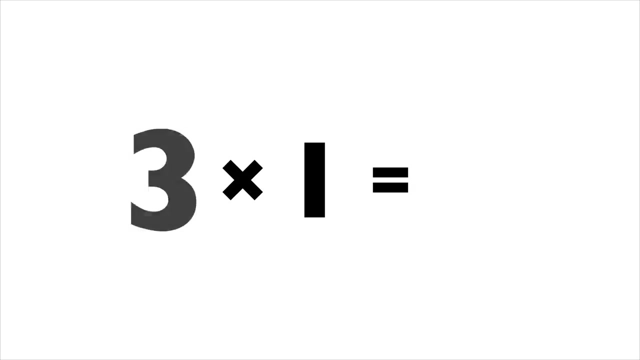 16: 2 times 10: equals 20. 2 times 12: equals 24. 3 times 1: equals 3, 3. 3 times 1: equals 3, 3 times 2. equals 3 times 2, equals 6, 3. 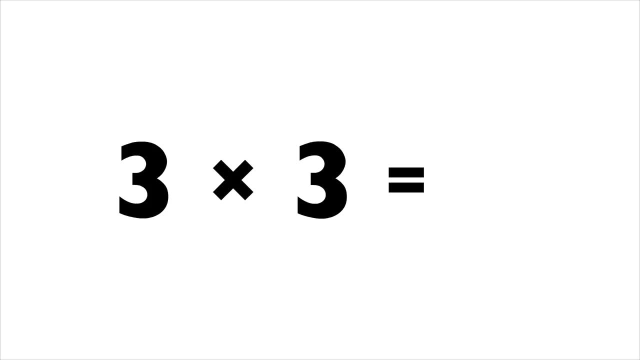 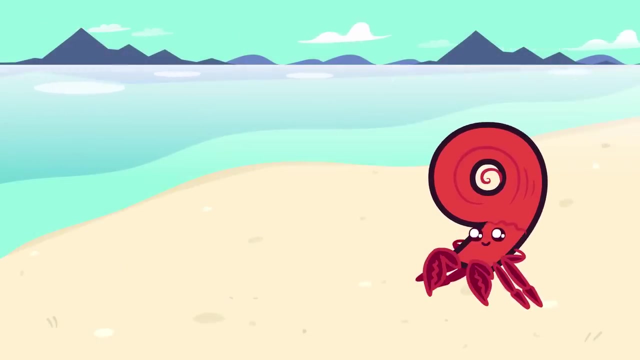 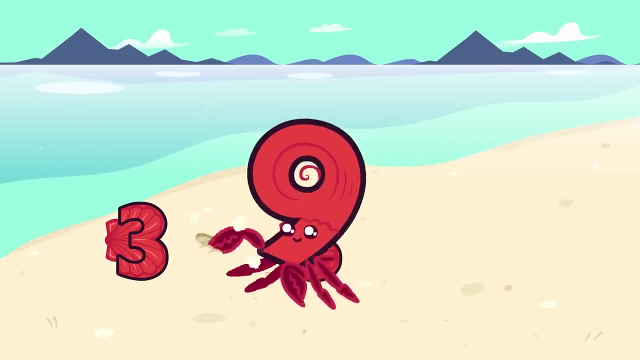 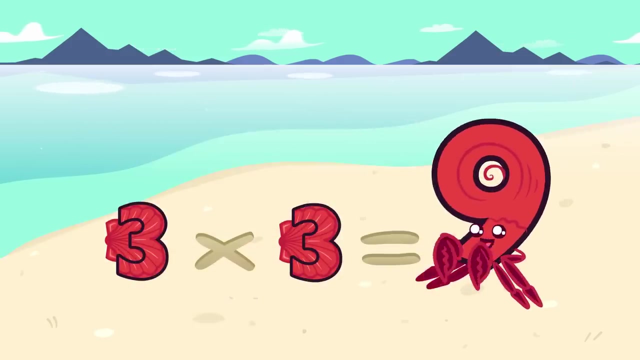 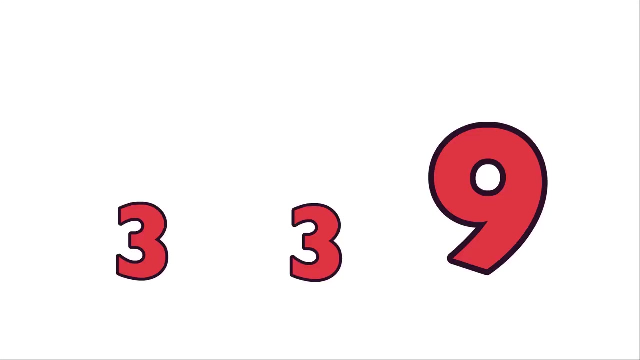 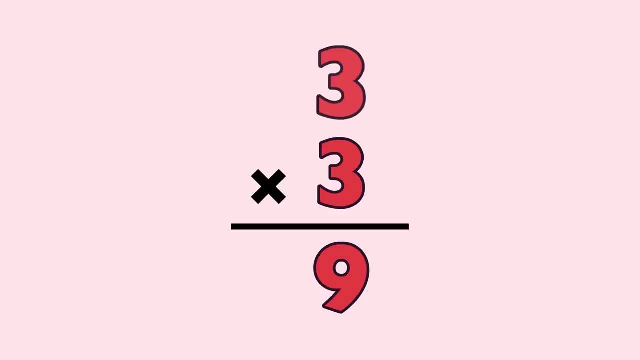 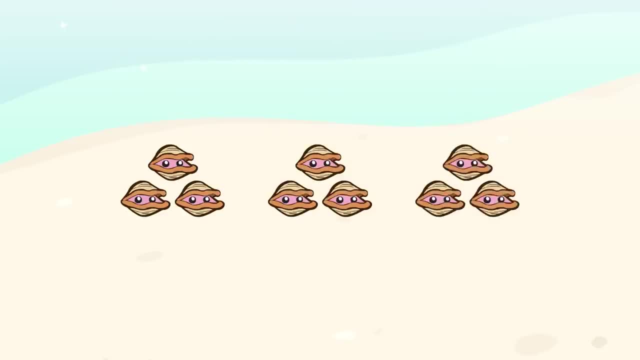 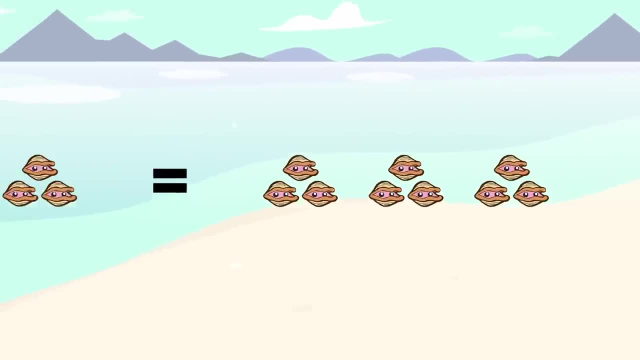 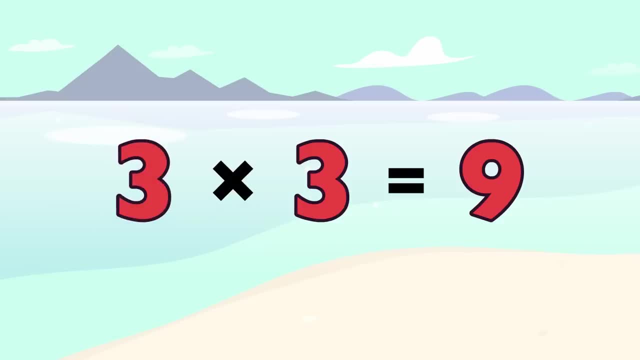 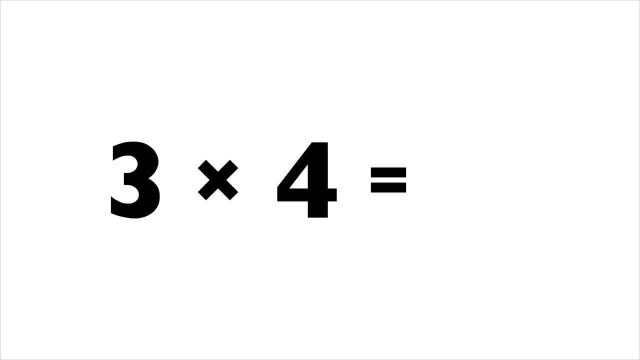 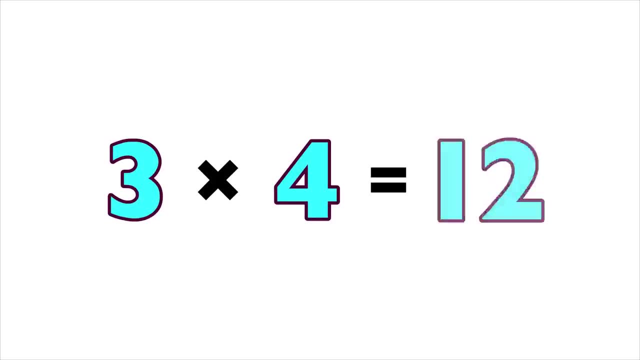 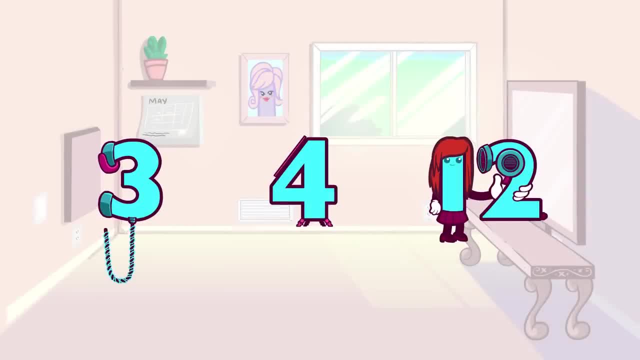 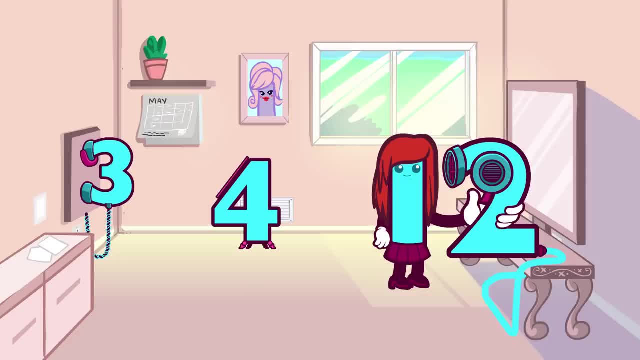 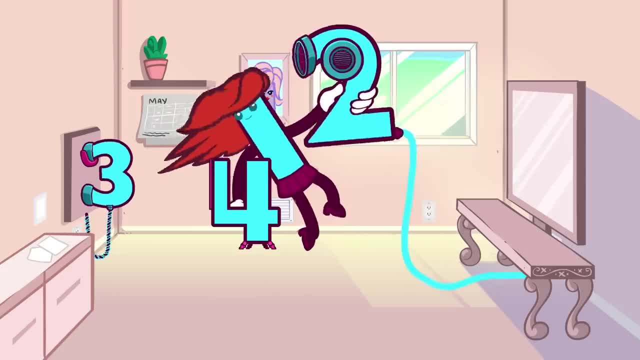 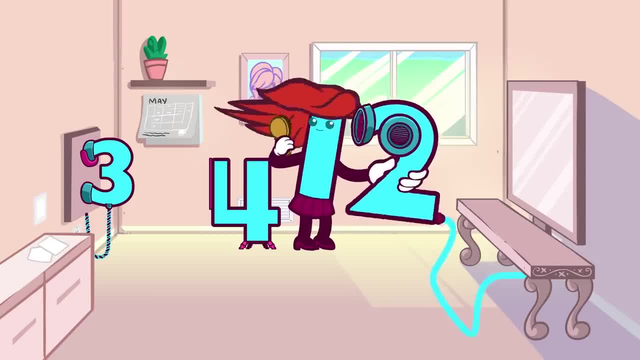 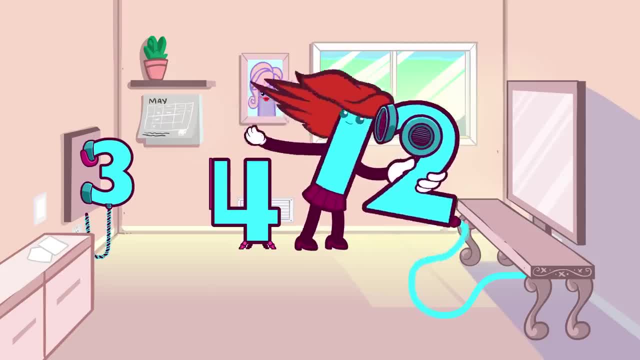 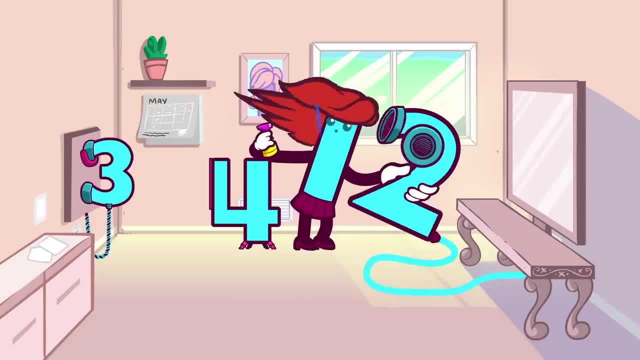 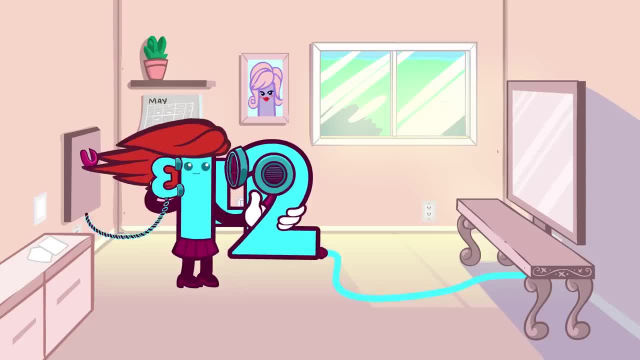 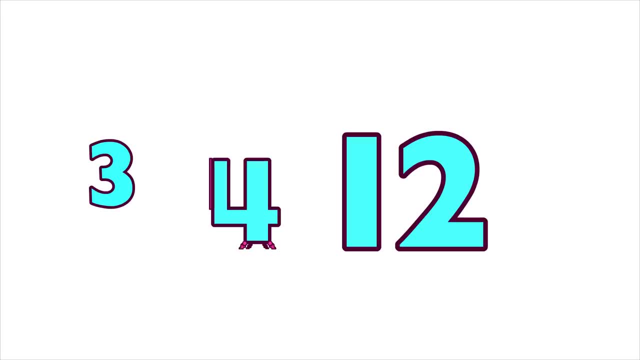 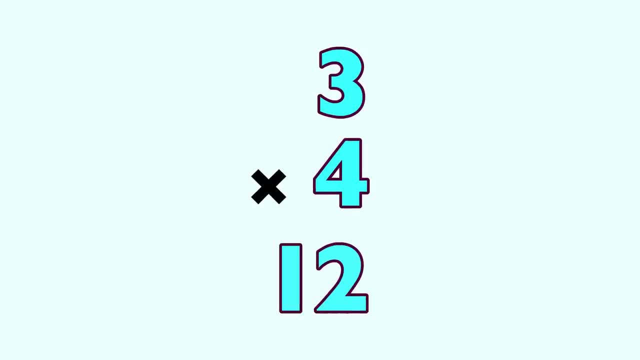 3 × 4 equals 12. 3 × 4 equals 12. 3 × 4 equals 12. 1, 2, 3, 4s equals 12. 1, 2, 3, 4s equals 12. 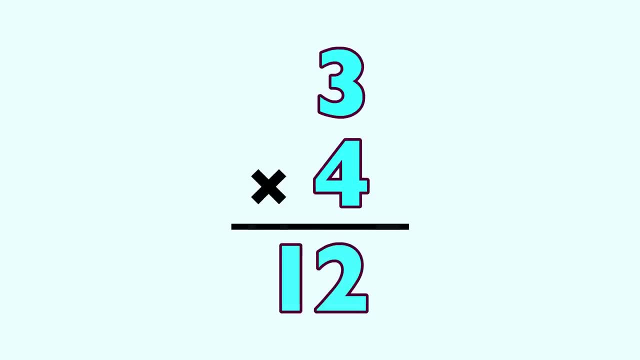 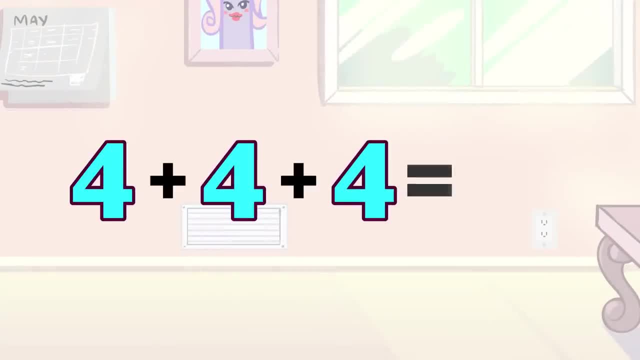 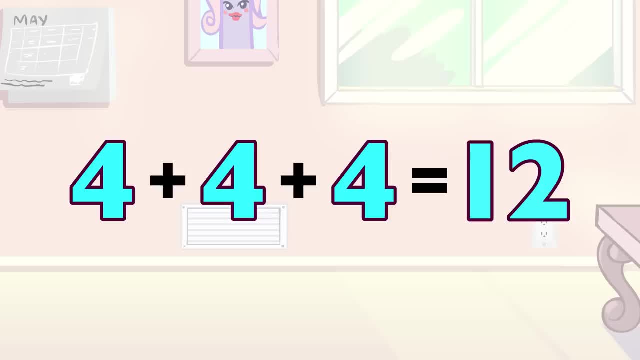 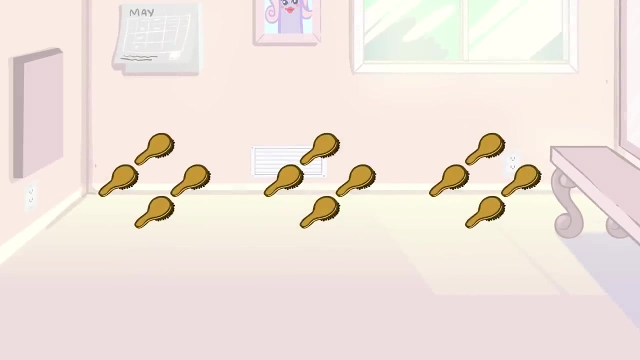 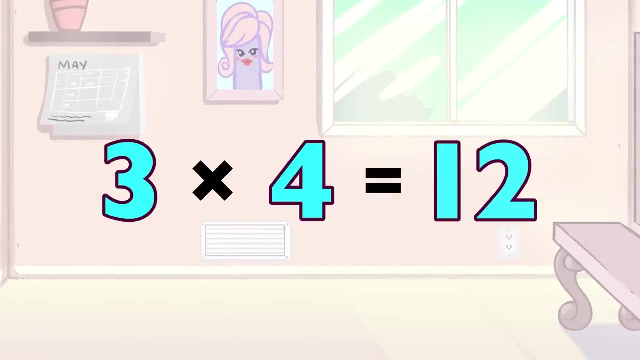 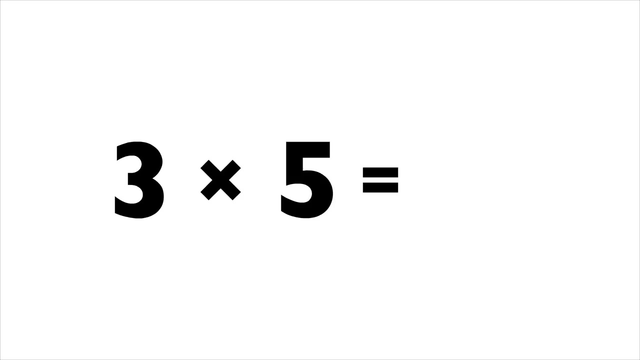 1, 2, 3, 4's equals 12. 3 times 4 equals 12. 4, 8, 12 equals 12. 12 equals 12. 3 times 4 equals 12. 3 times 4 equals 12. 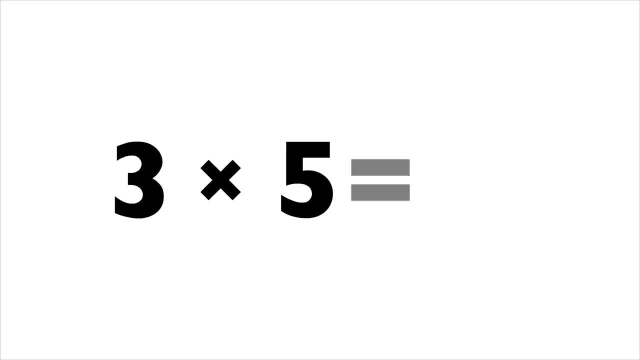 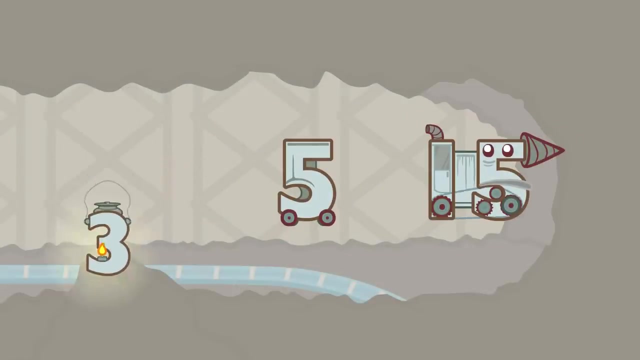 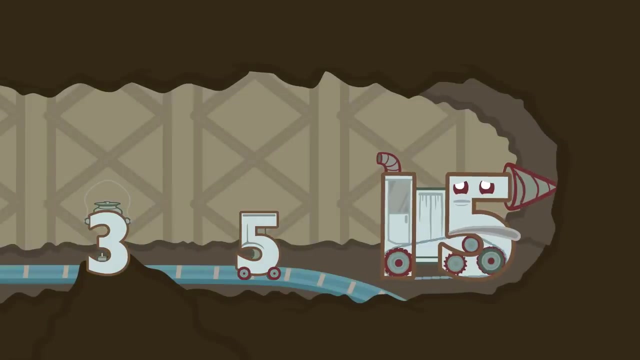 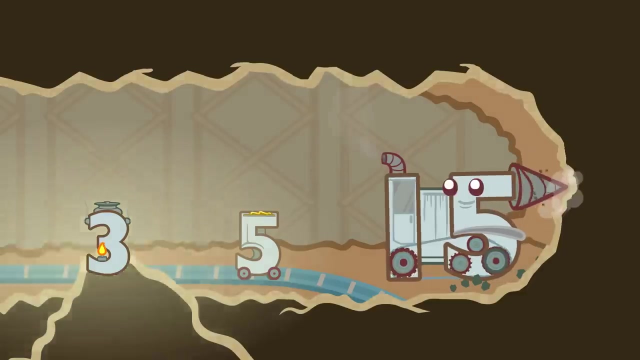 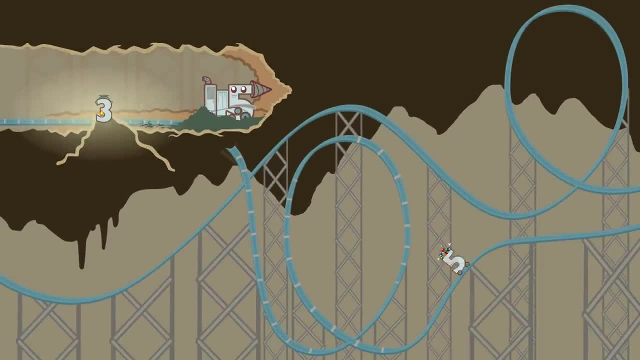 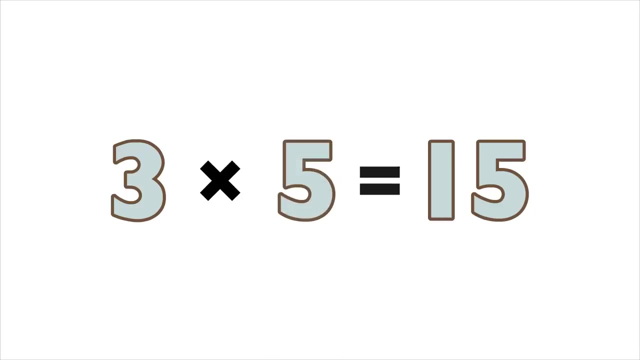 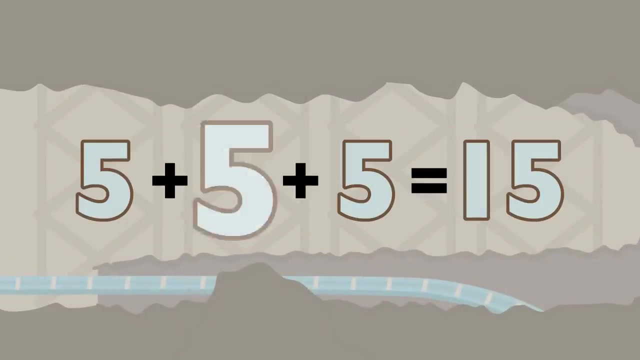 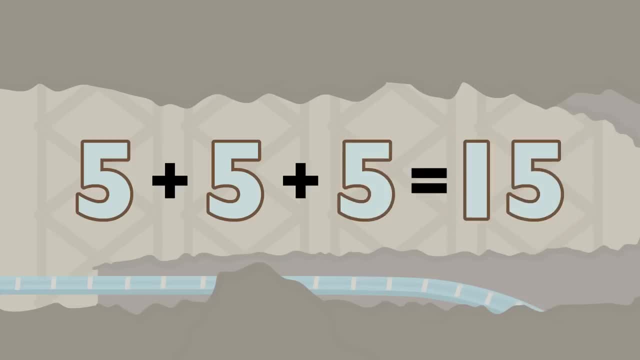 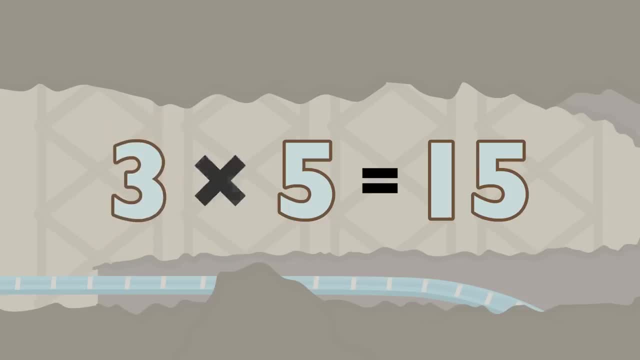 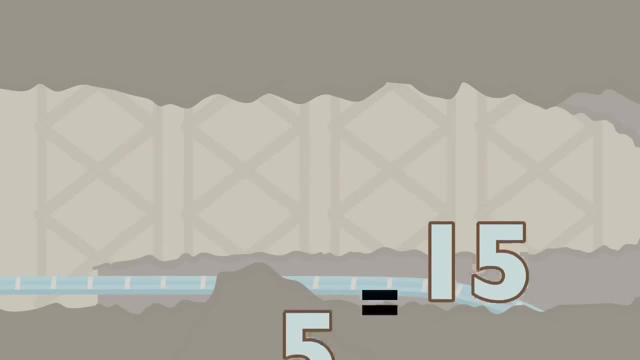 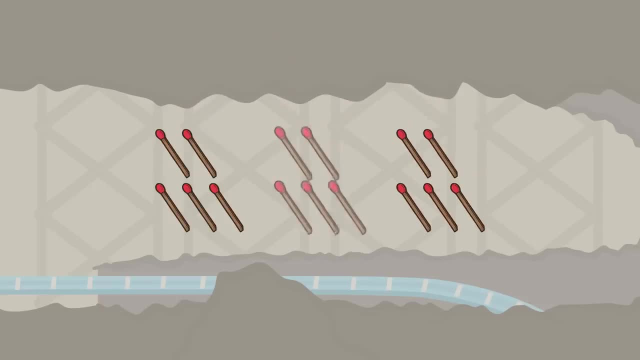 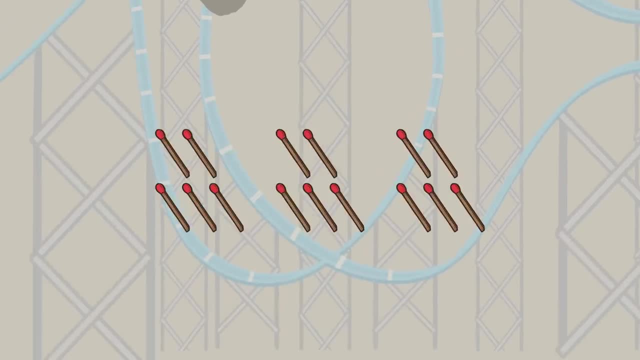 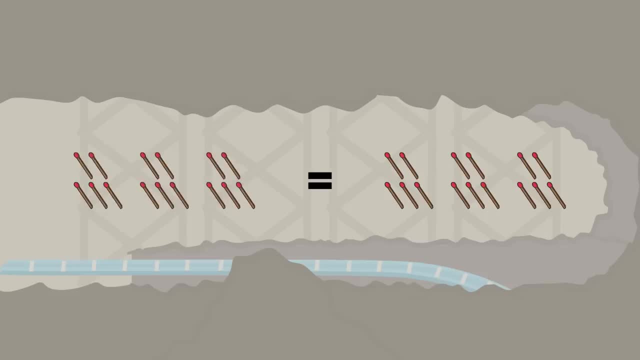 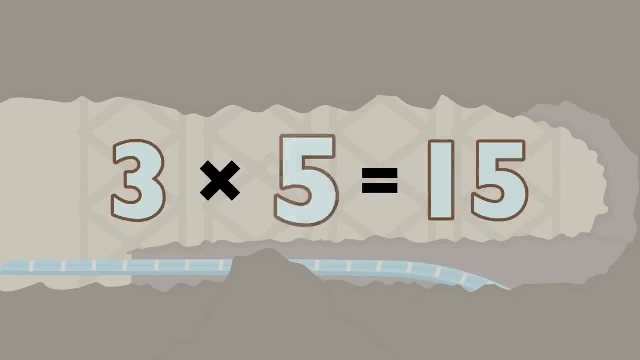 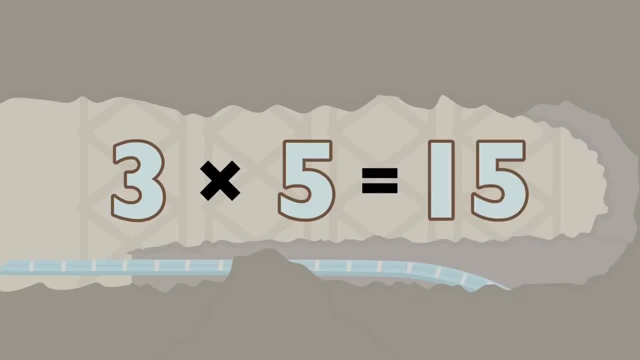 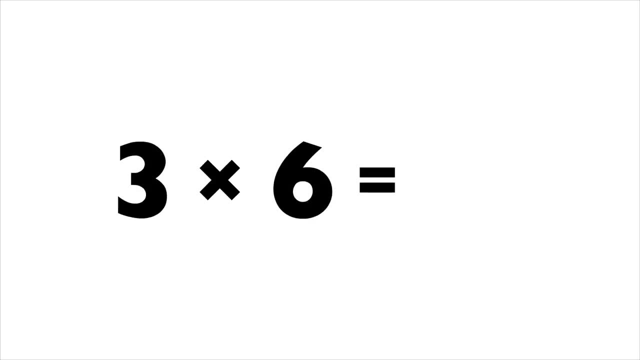 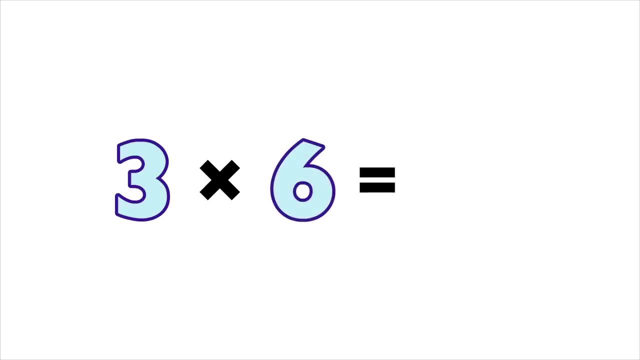 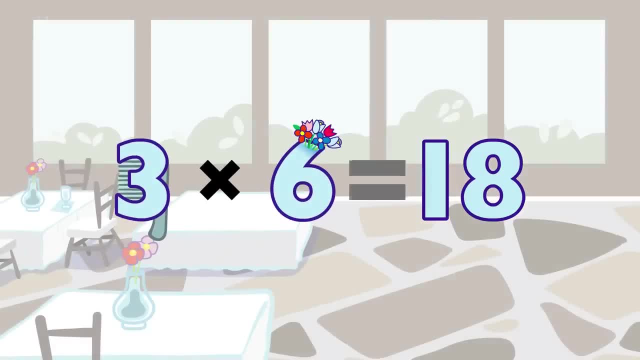 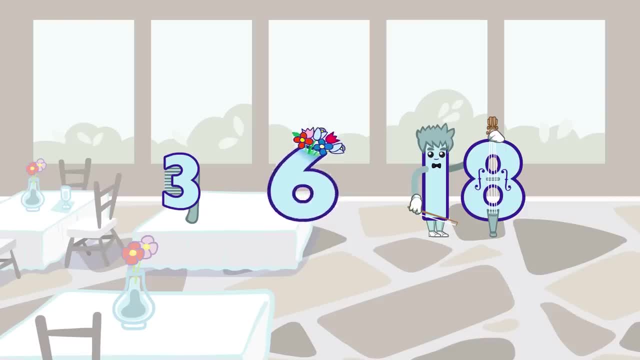 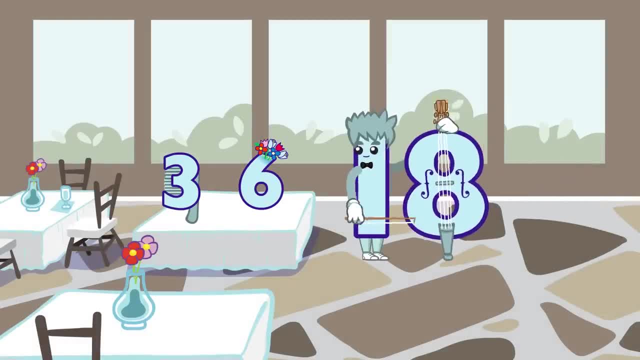 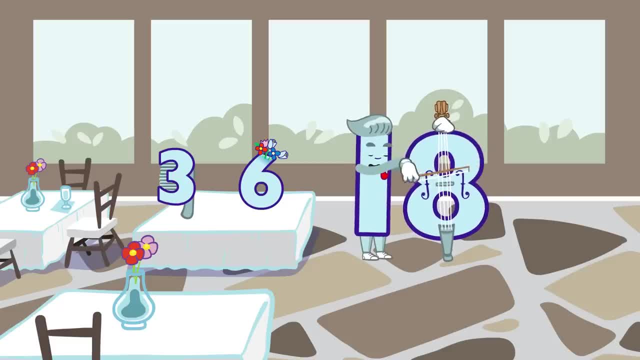 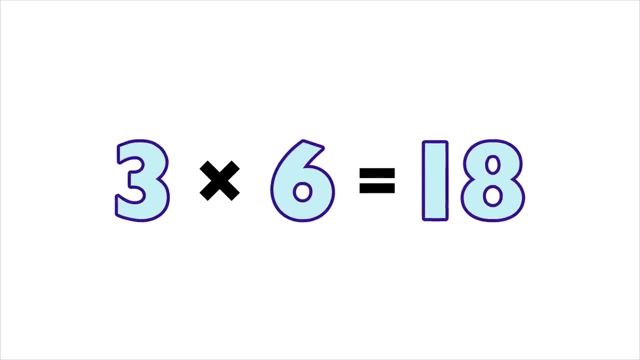 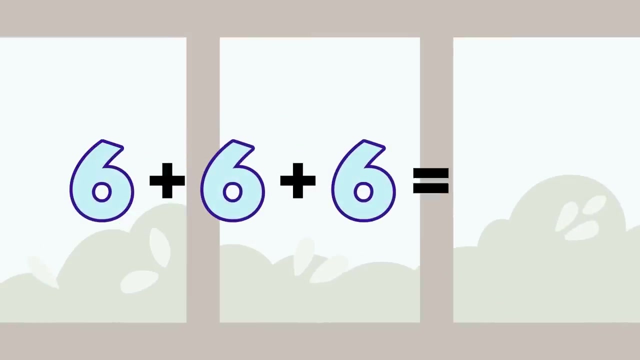 Hmm, 3 times 6 equals 18.. 3 times 6 equals 18.. 3 sixes equals 18.. 1, 2, 3 sixes equals 18.. 3 times 6 equals 18.. 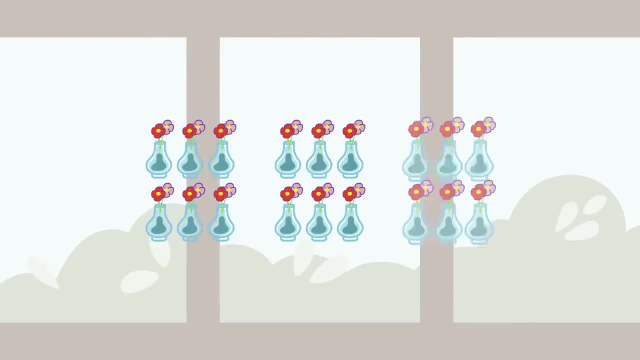 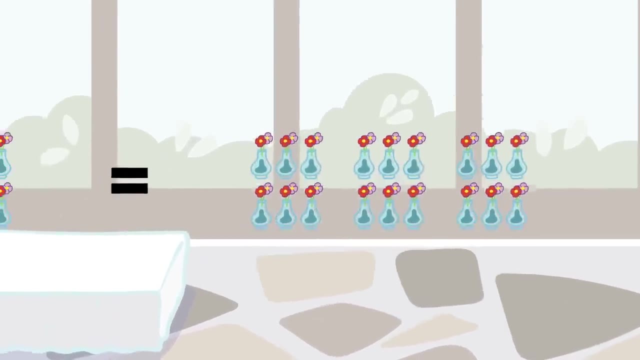 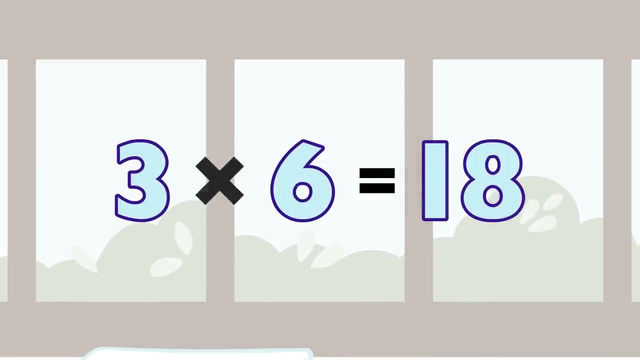 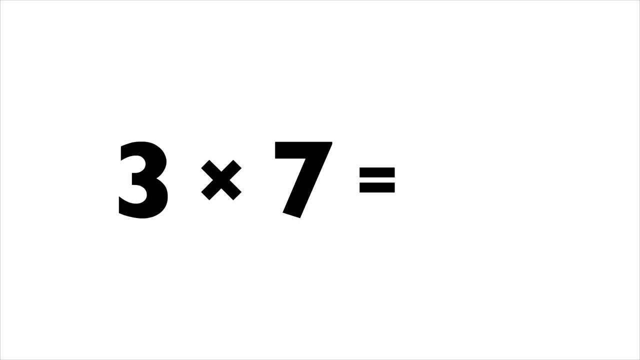 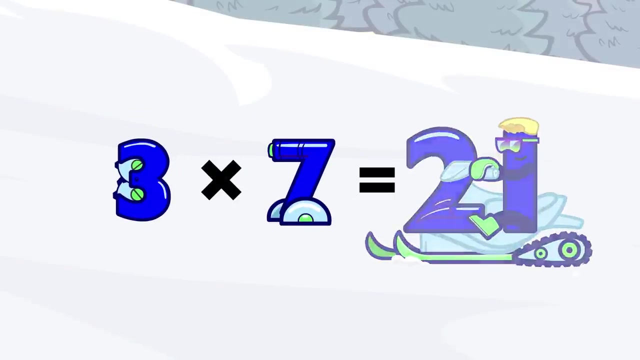 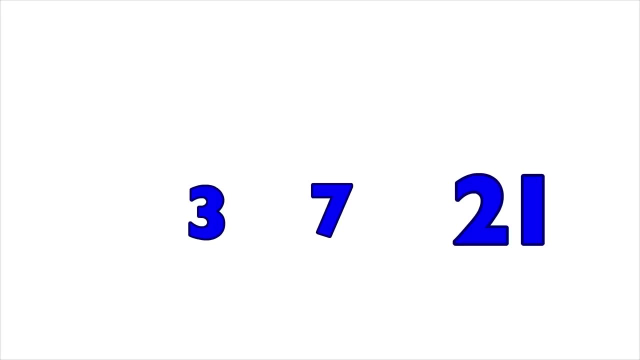 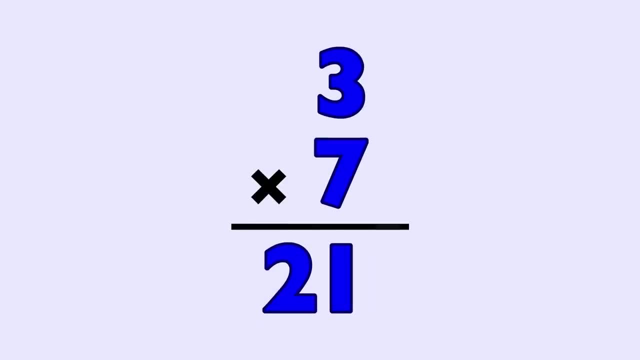 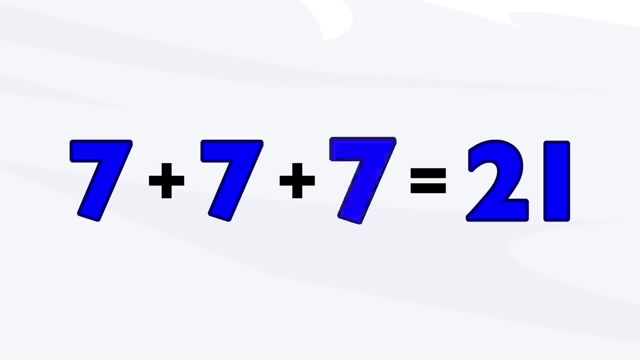 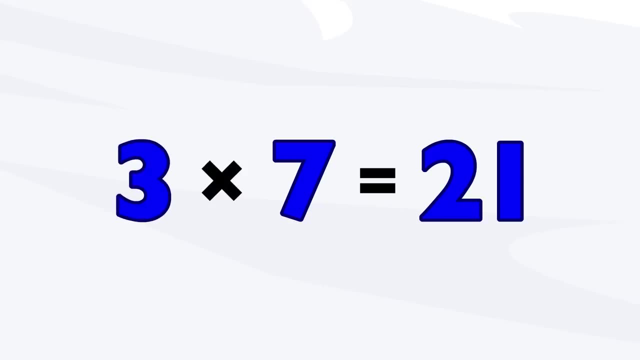 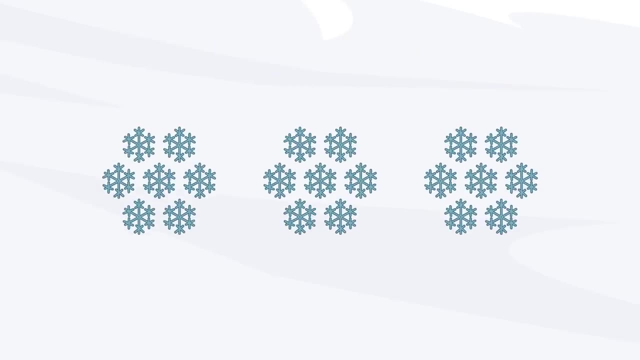 3 times 7 equals 21.. 3 times 7 equals 21.. 3 times 7 equals 21.. 1,, 2, 3, 7s equals 21.. 3 times 7 equals 21.. 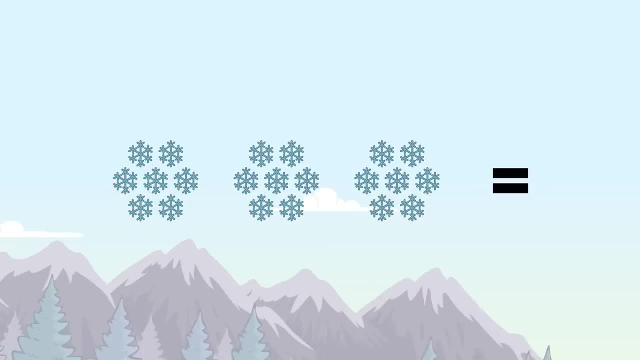 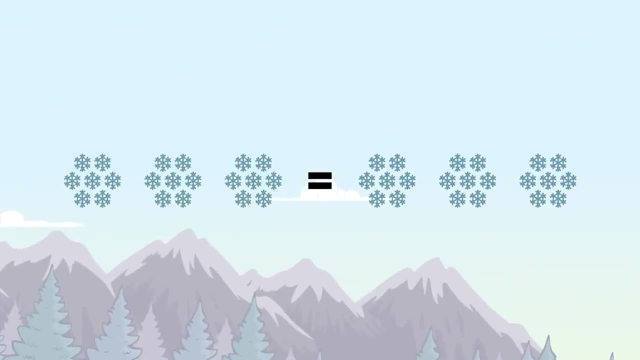 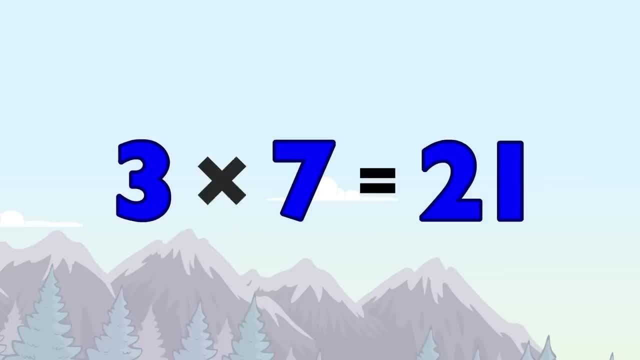 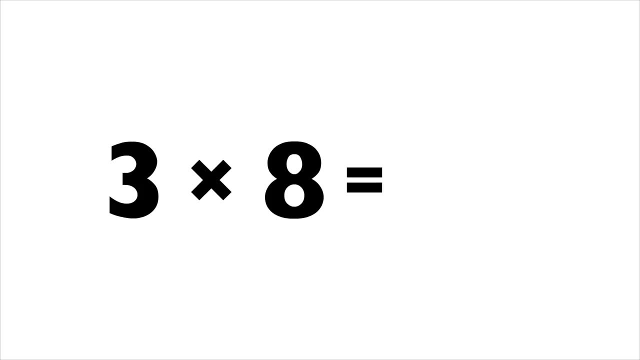 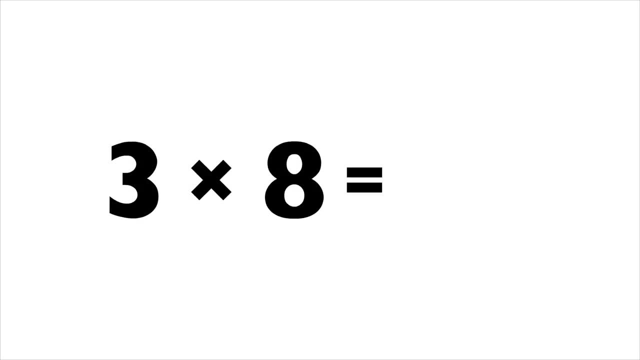 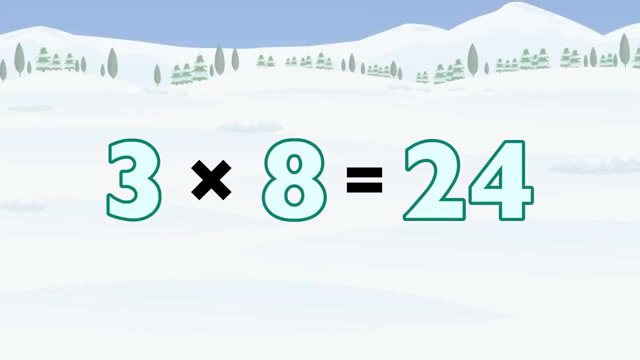 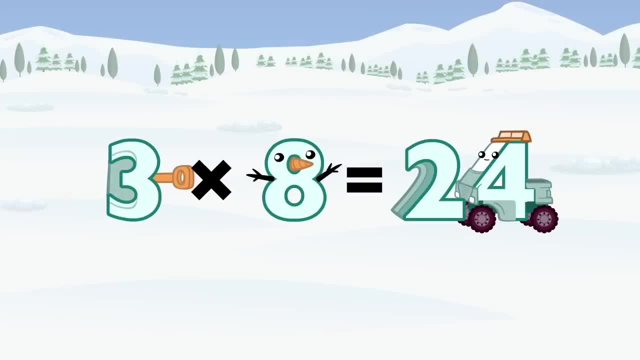 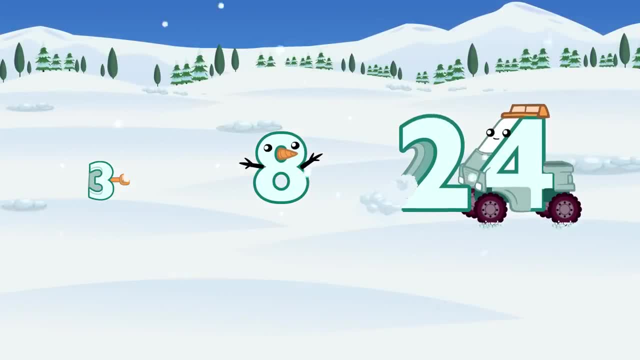 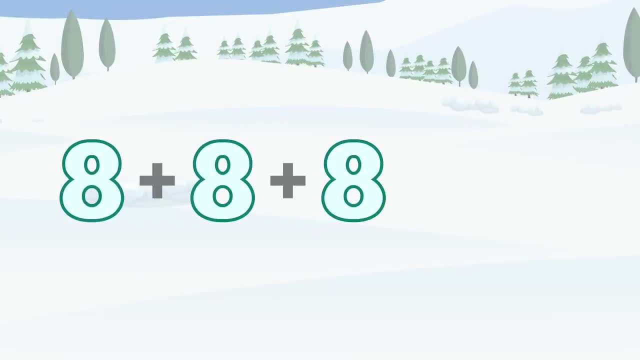 3 times 8 equals. 3 times 8 equals 24.. 3 times 8 equals. 3 times 8 equals 24.. 1, 2, 3, 8 equals 24.. 3 times 8 equals 24.. 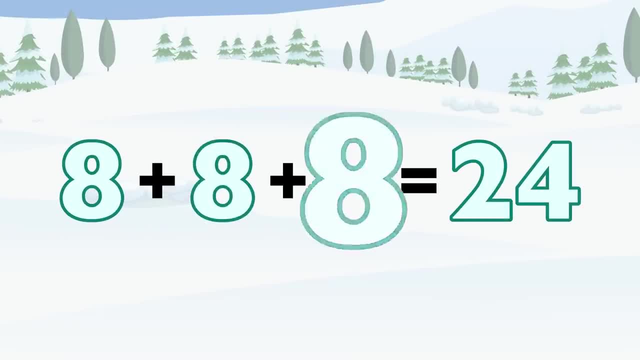 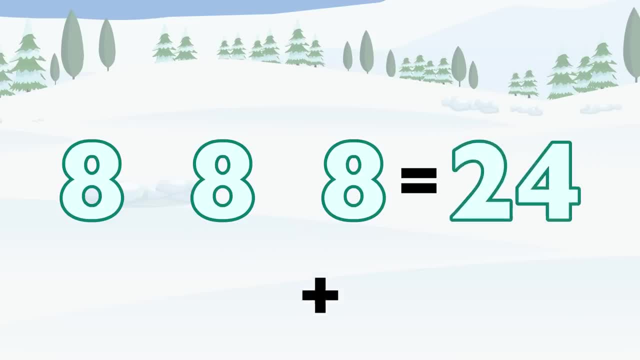 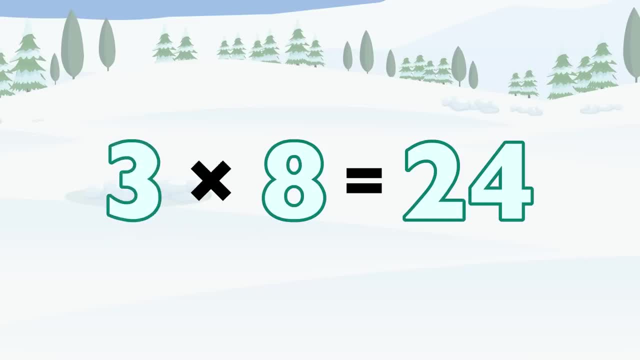 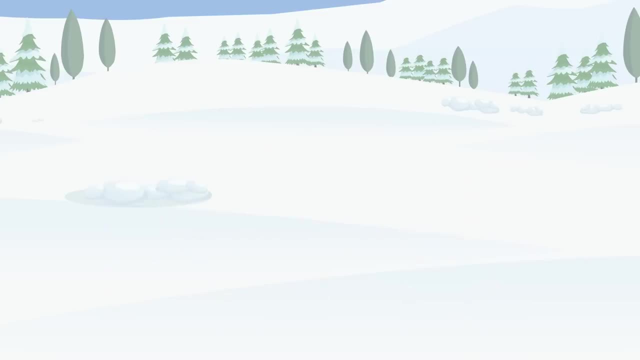 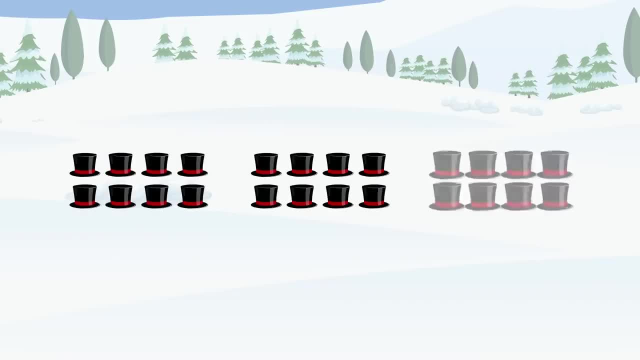 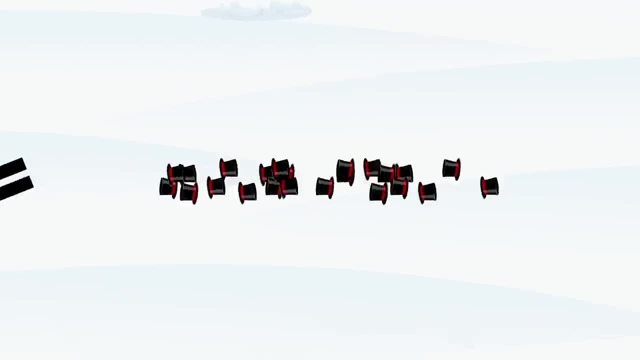 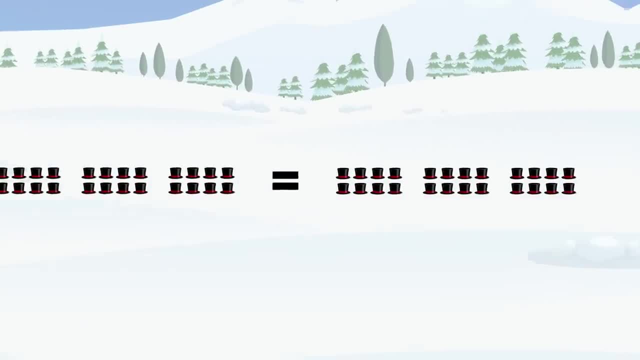 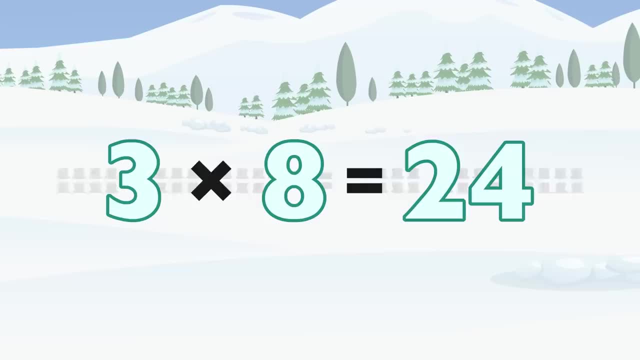 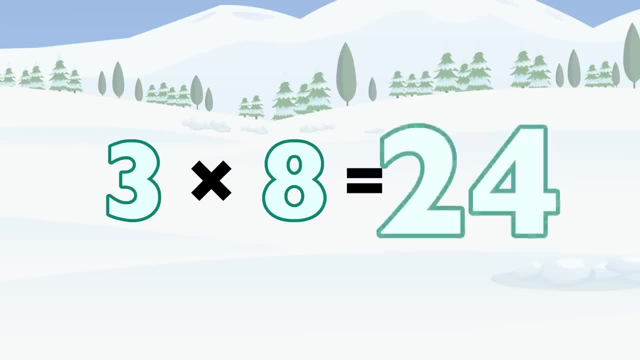 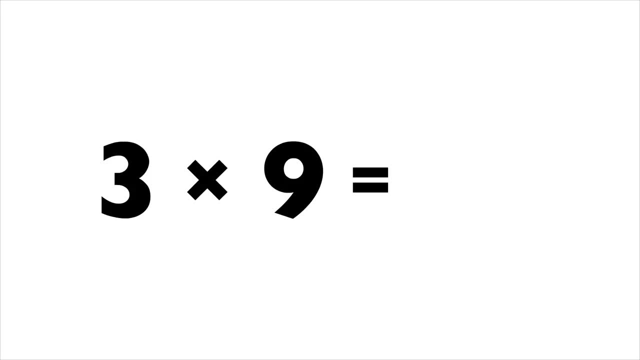 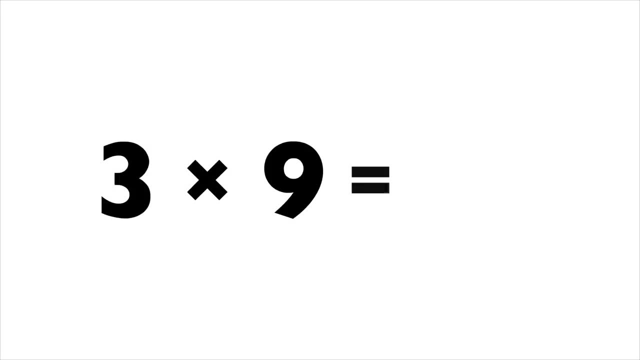 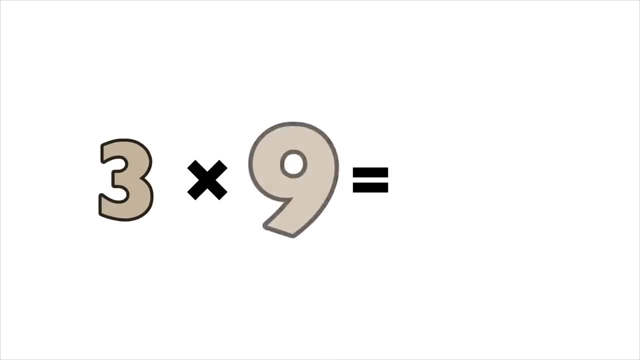 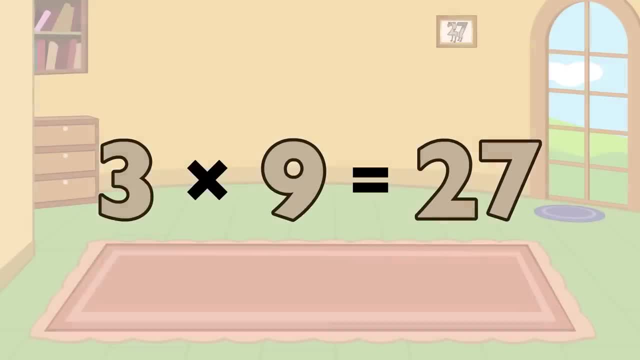 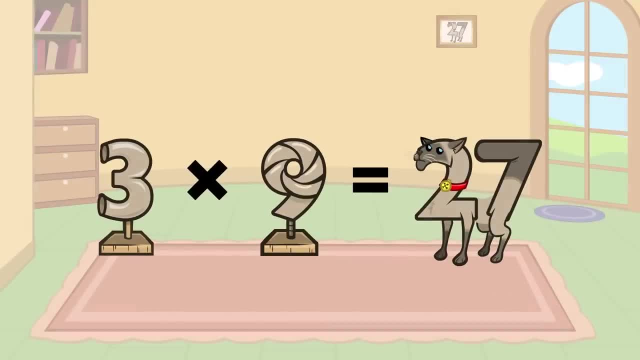 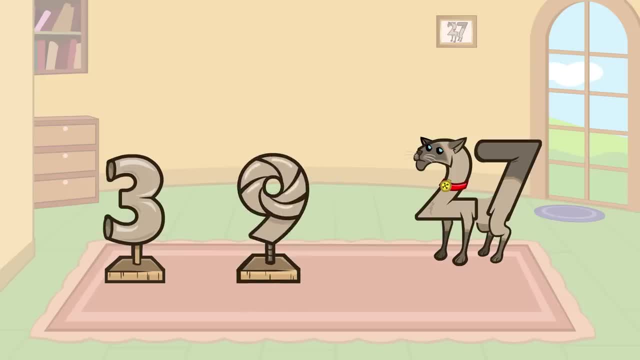 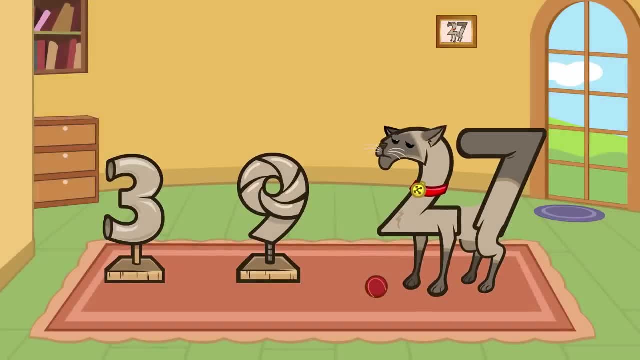 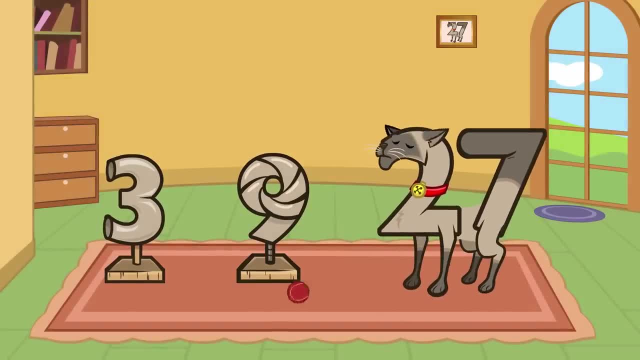 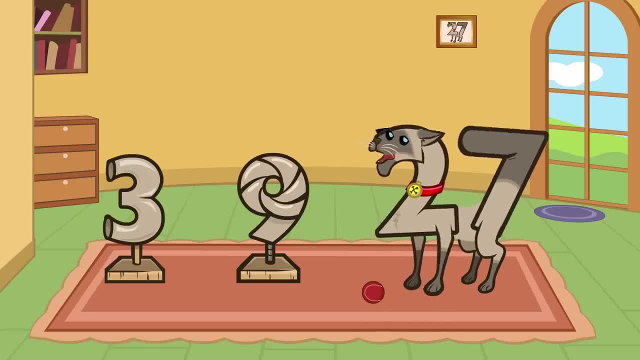 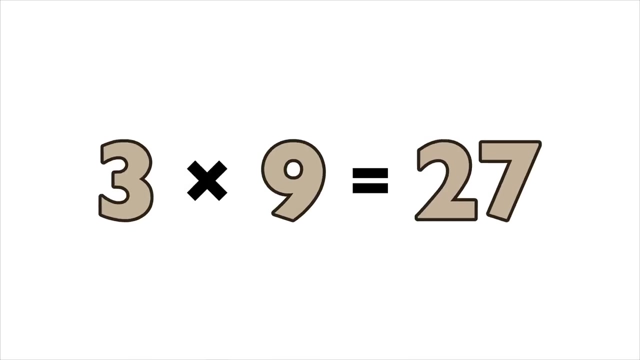 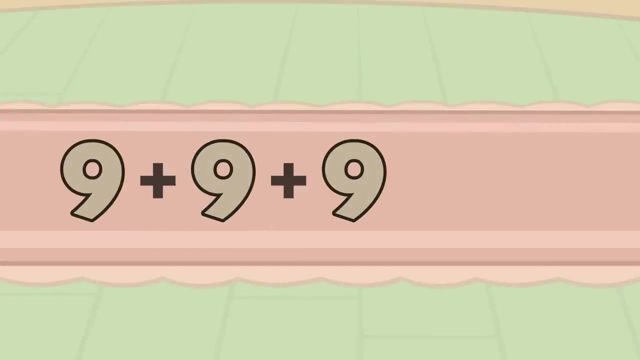 3 times 9 equals 27.. 3 times 9 equals 27.. 3 times 9 equals 27.. Three times nine equals twenty-seven. Three times nine equals twenty-seven. Three nines equals twenty-seven. One, two, three nines equals twenty-seven. 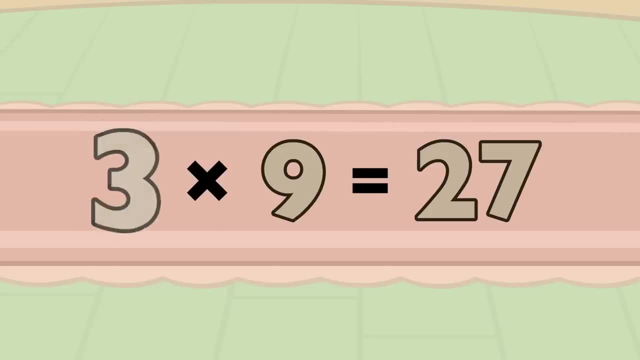 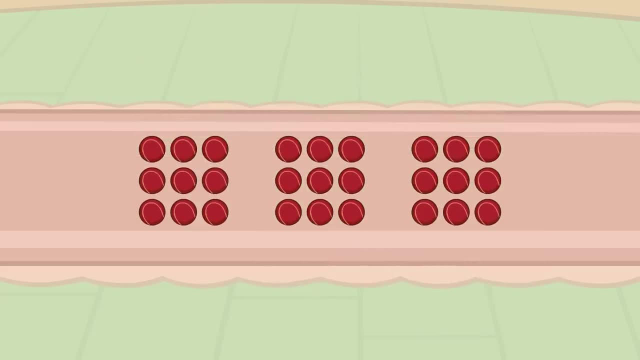 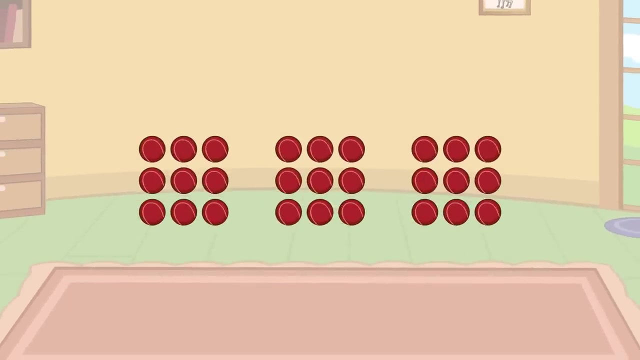 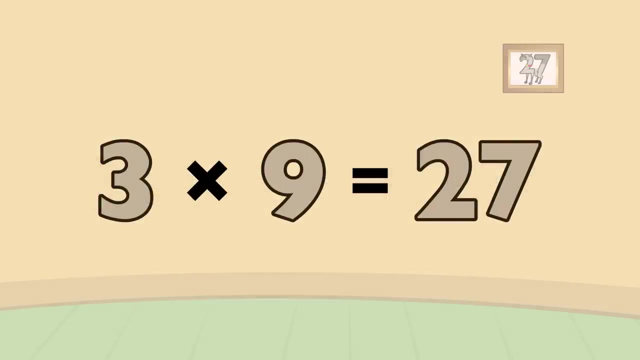 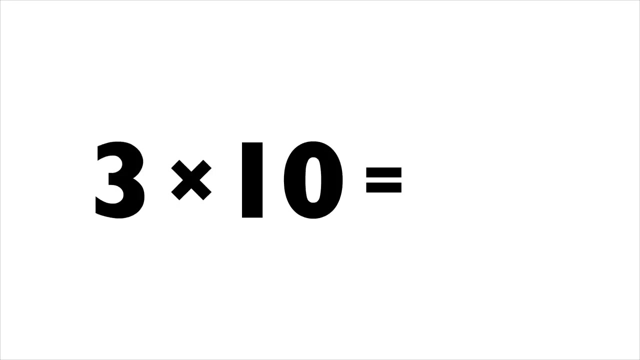 Three times nine equals twenty-seven. Nine, eighteen, twenty-seven equals twenty-seven. Twenty-seven equals twenty-seven. Three times nine equals twenty-seven. Nine, eighteen, twenty-seven equals twenty-seven. Three times ten equals Three times ten equals thirty. 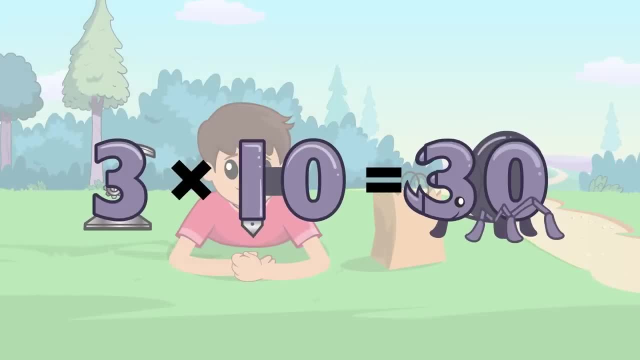 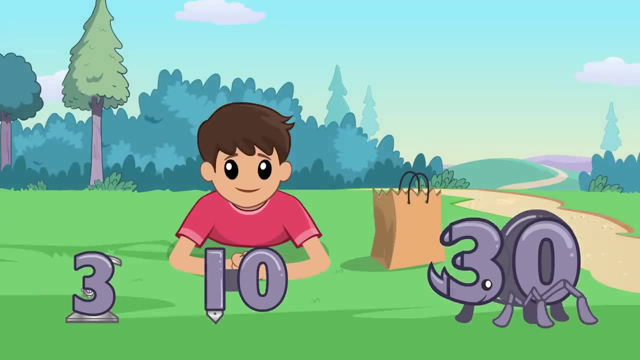 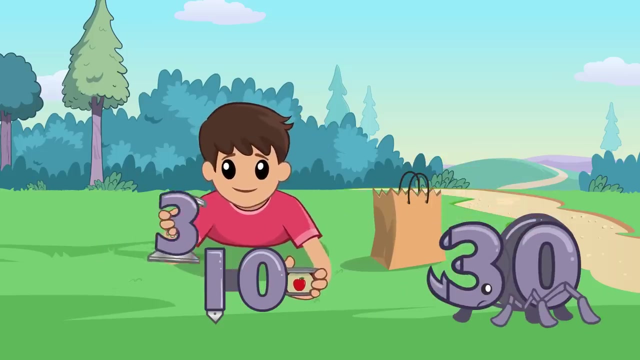 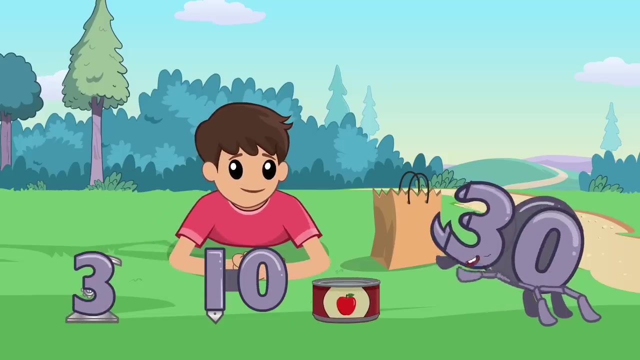 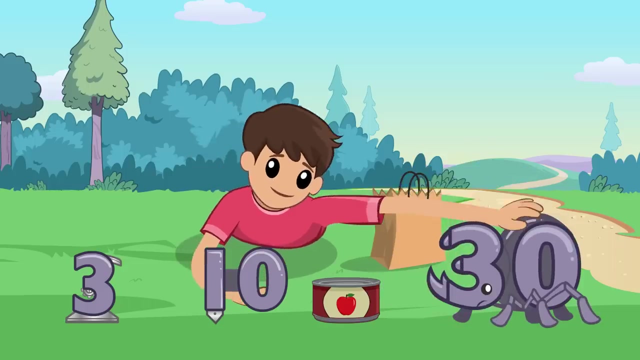 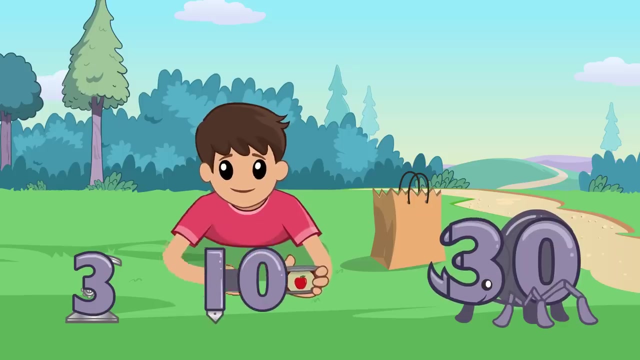 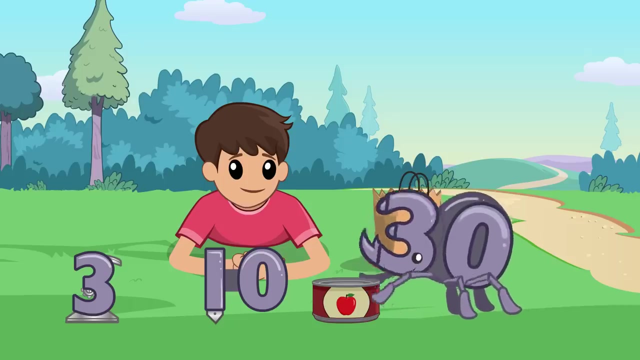 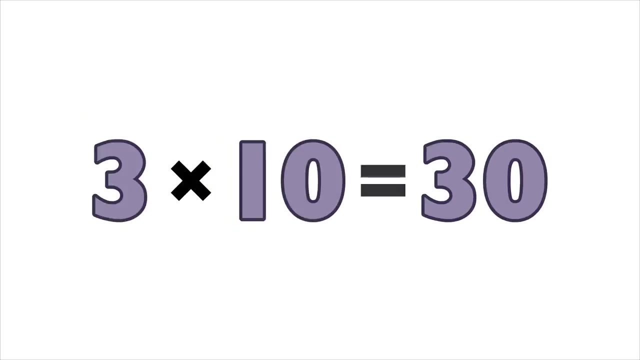 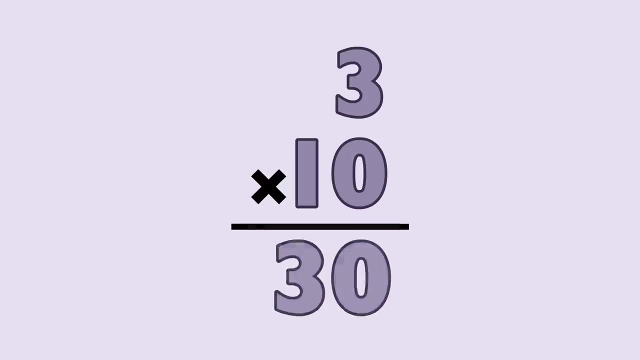 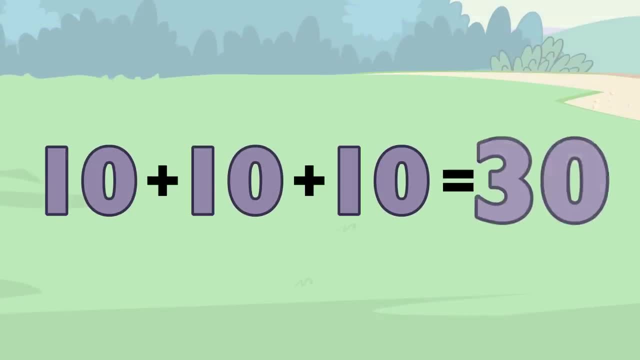 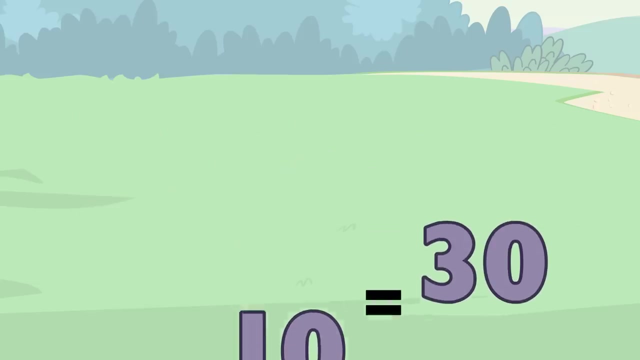 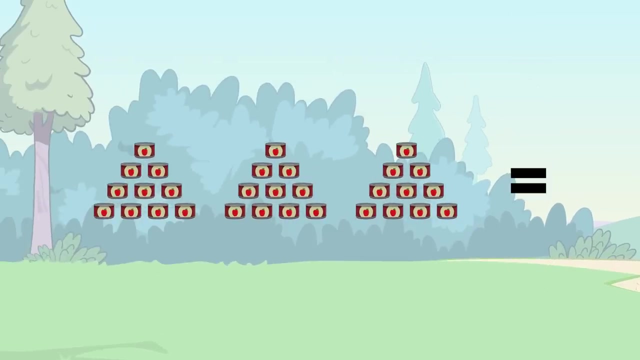 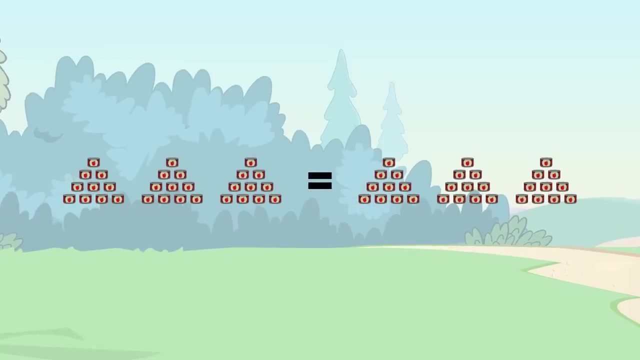 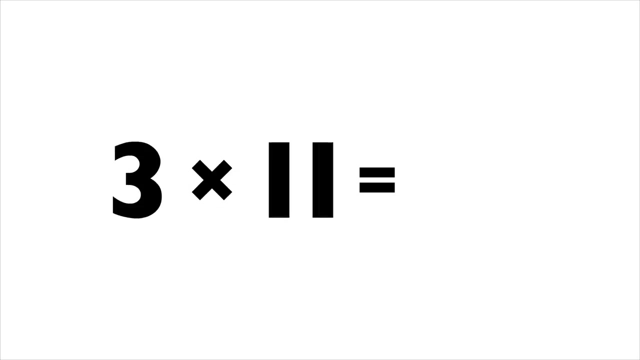 Three tens equals thirty One. two, three tens equals thirty Three times ten equals thirty Three times ten equals thirty Ten. twenty thirty equals thirty Thirty equals thirty Three times ten. equals thirty Three times eleven. equals Three times eleven. equals thirty three. 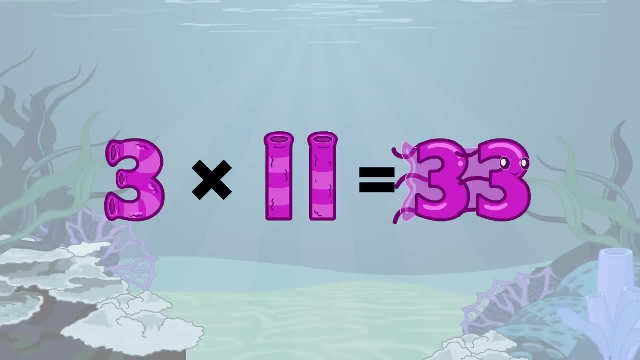 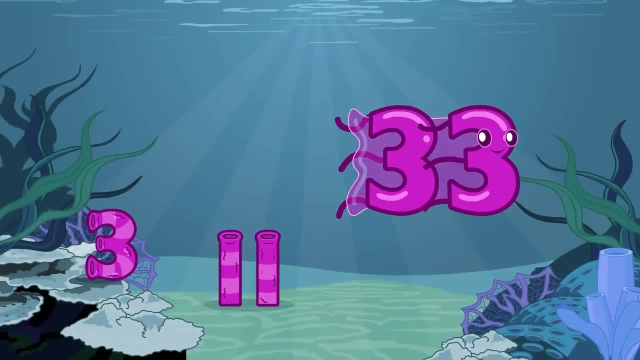 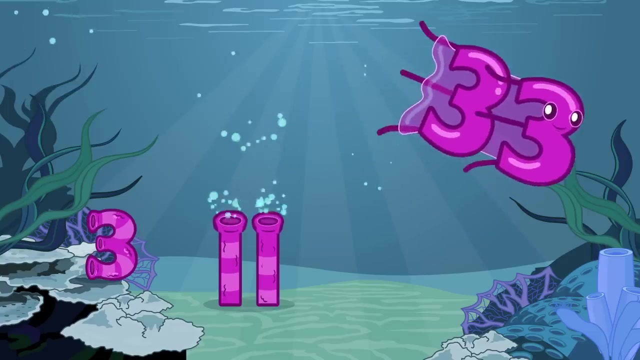 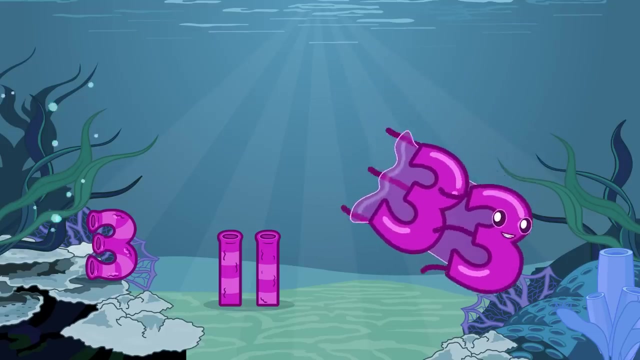 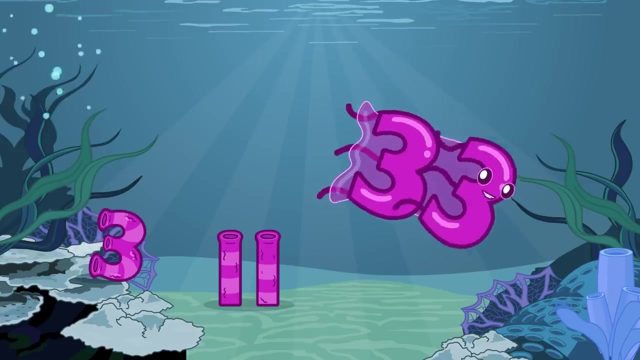 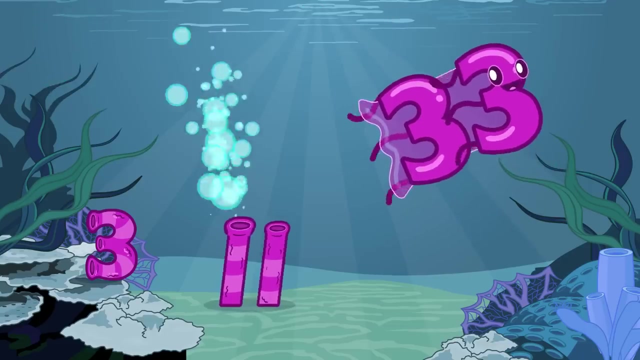 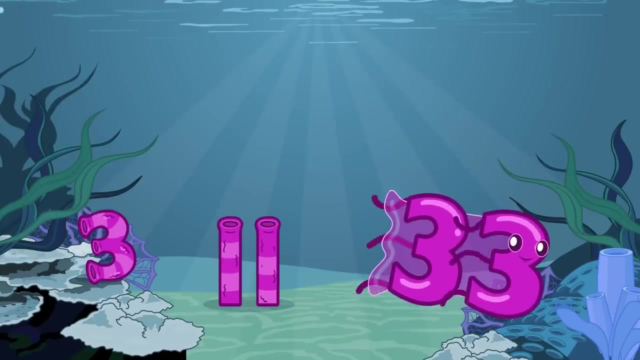 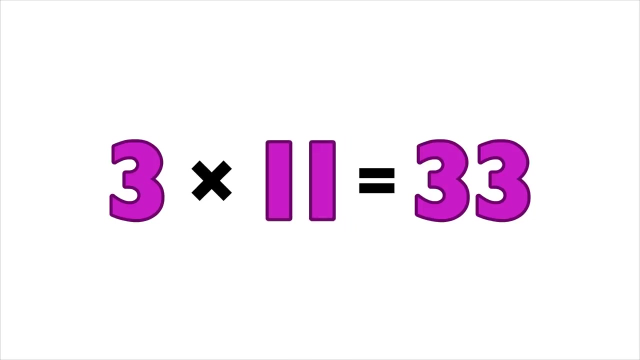 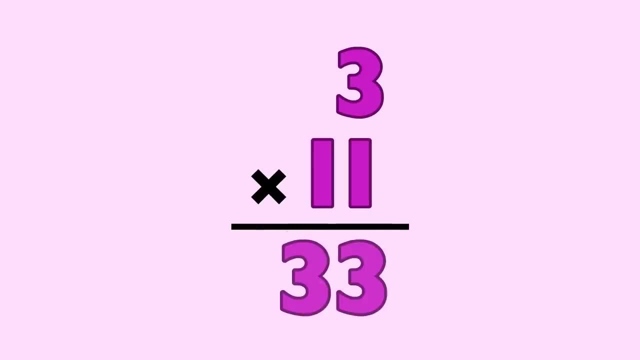 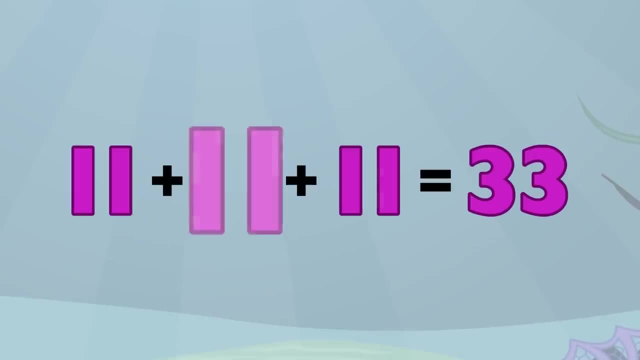 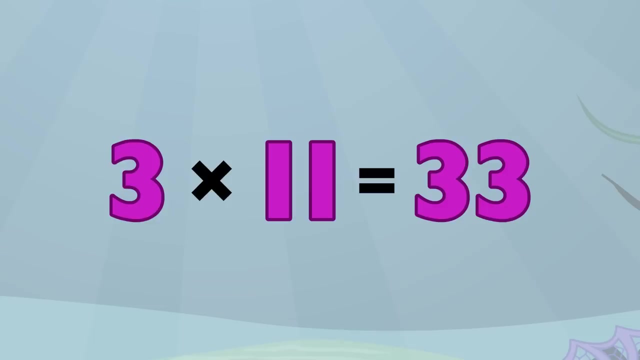 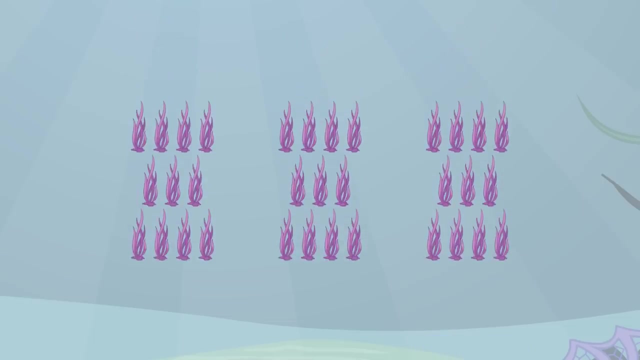 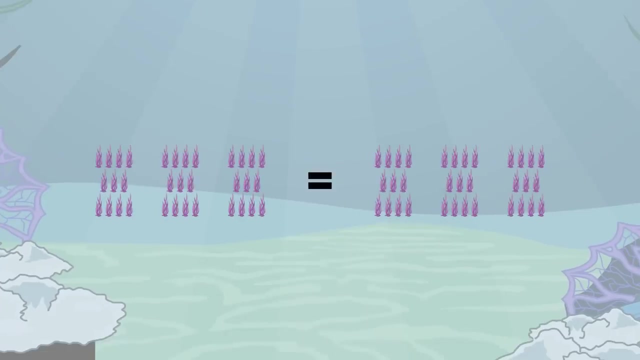 3 x 11 equals 33. 3 x 11 equals 33. 1, 2, 3 x 11 equals 33. 3 x 11 equals 33. 11,. 22, 33 equals 33. 33 equals 33. 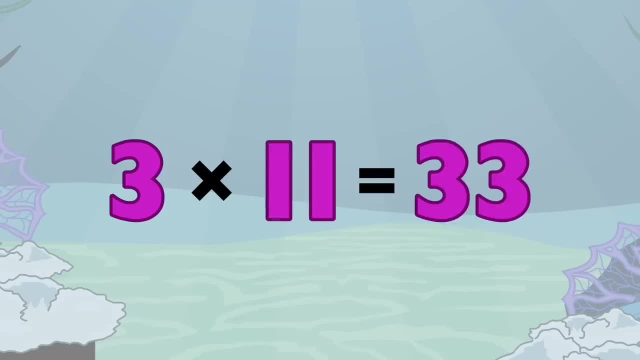 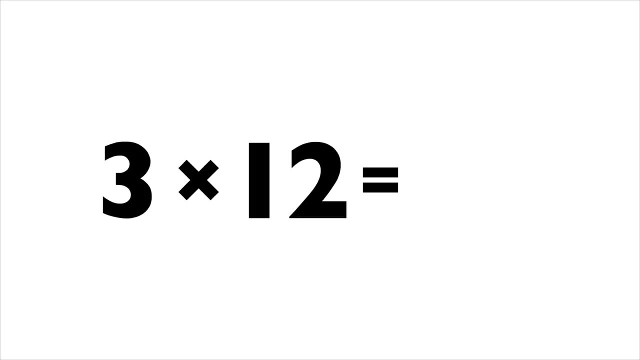 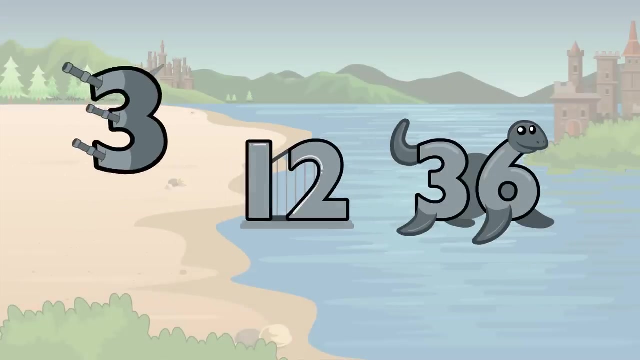 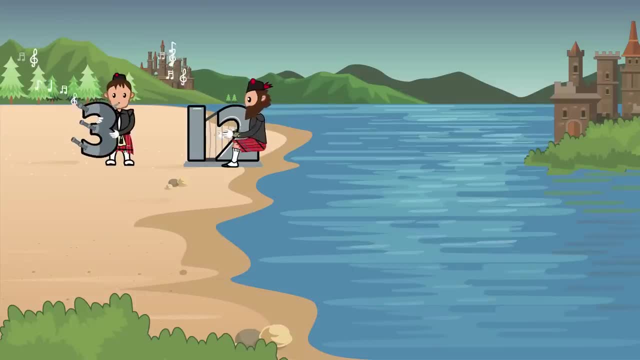 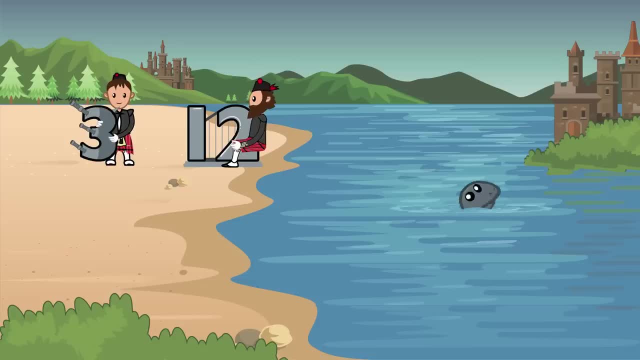 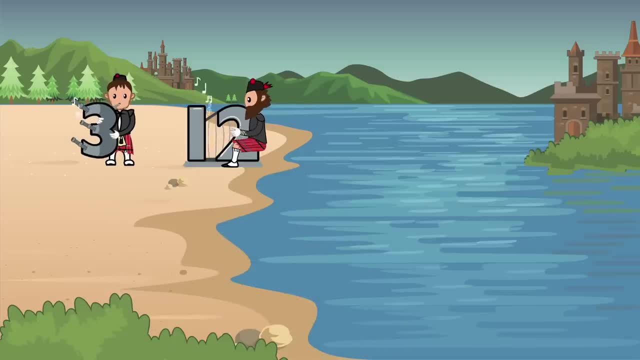 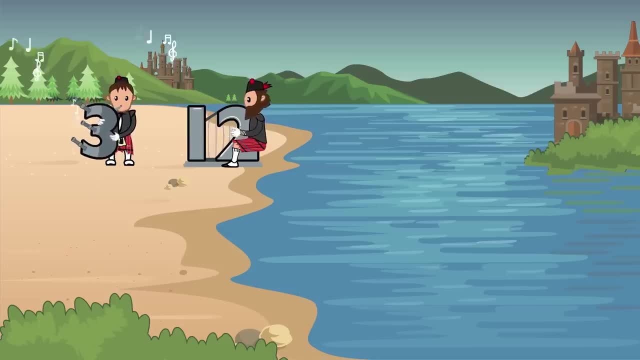 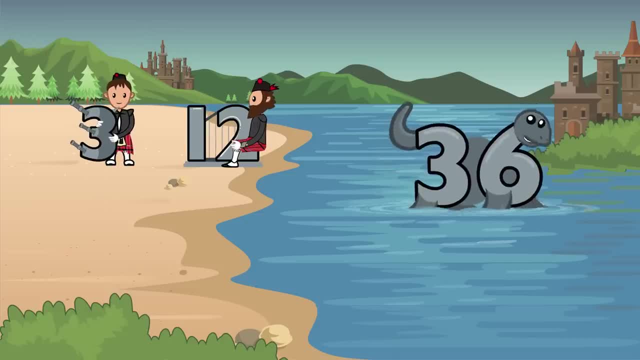 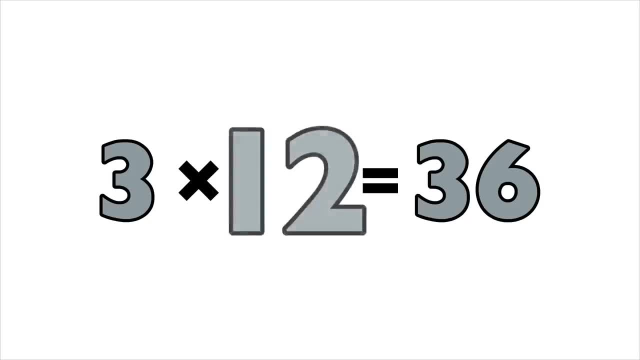 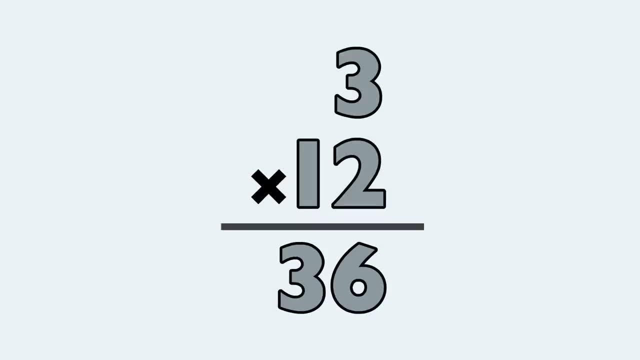 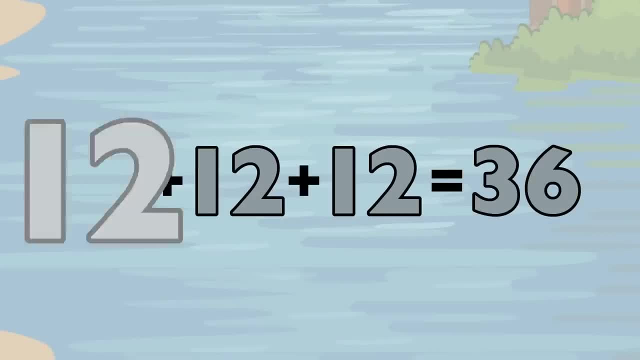 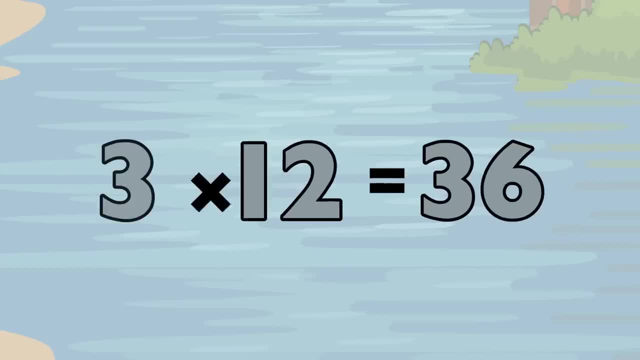 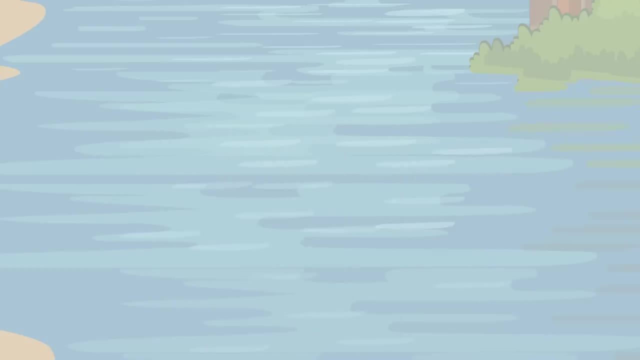 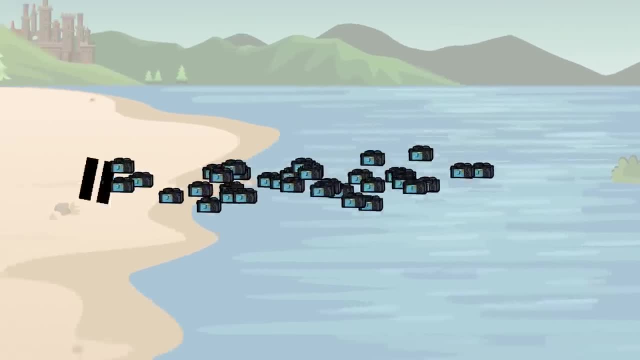 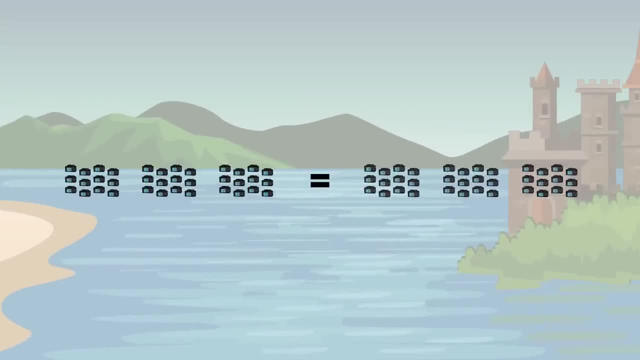 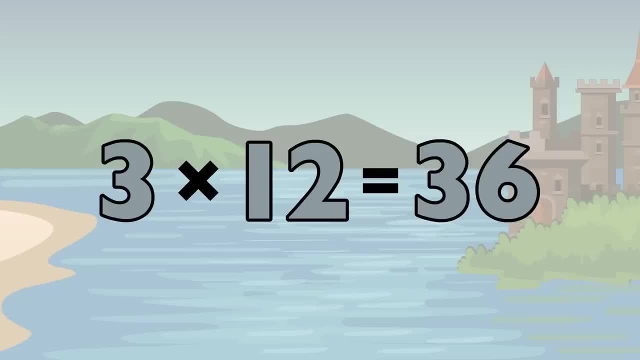 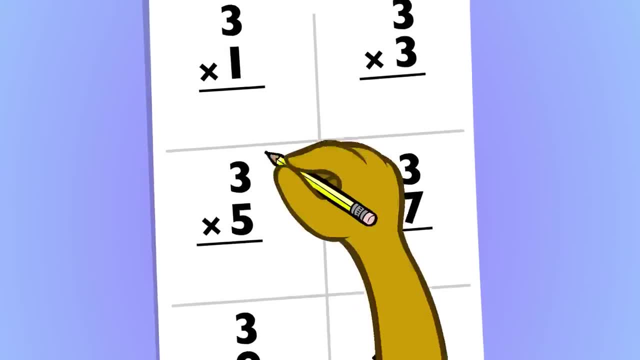 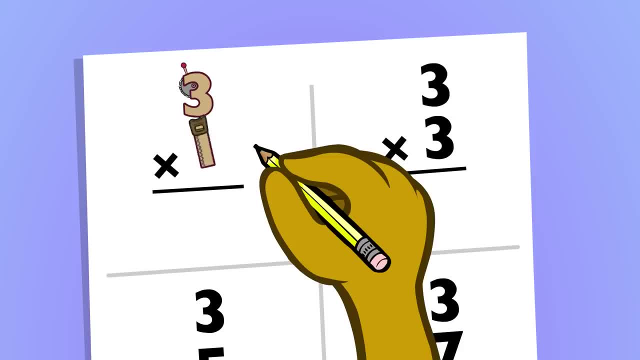 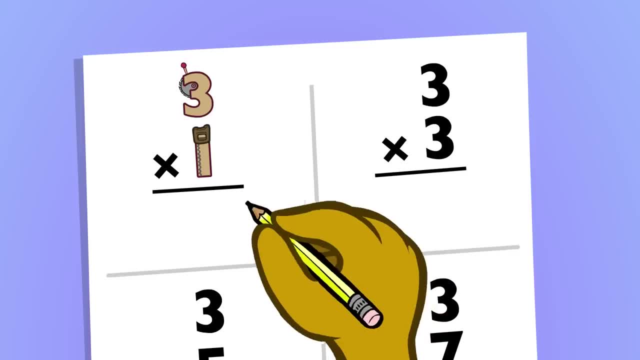 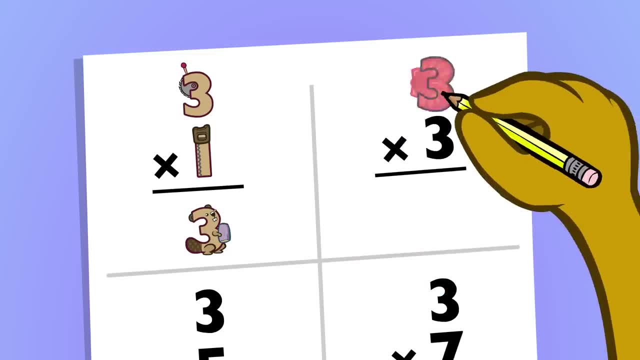 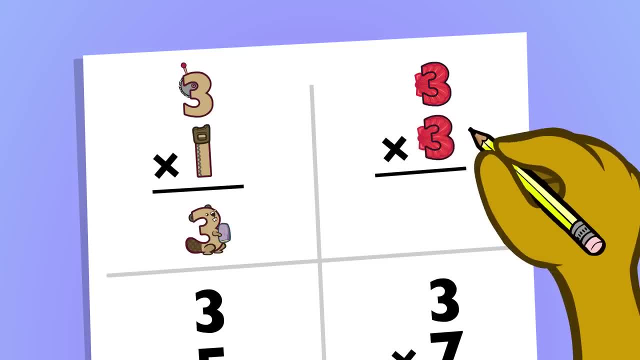 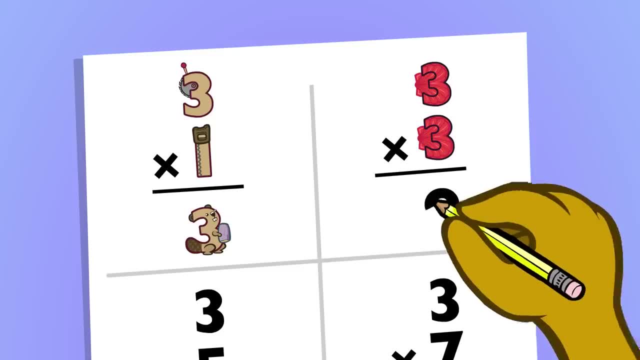 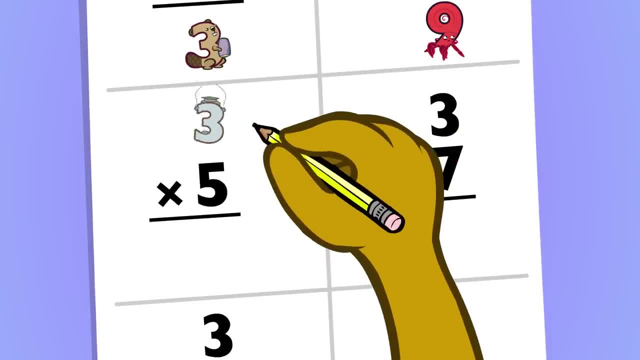 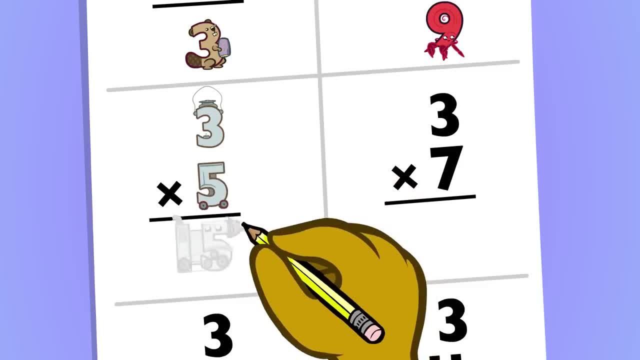 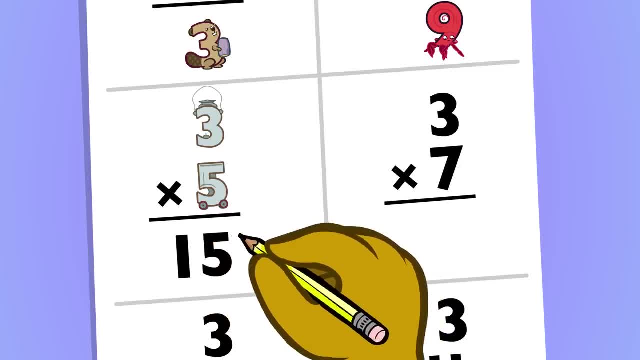 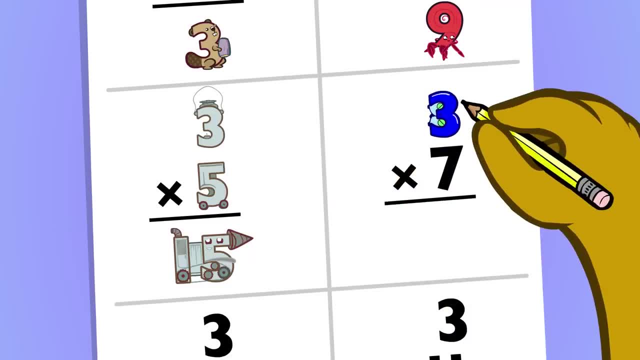 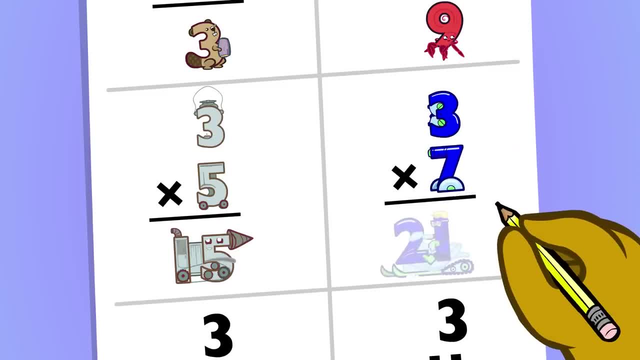 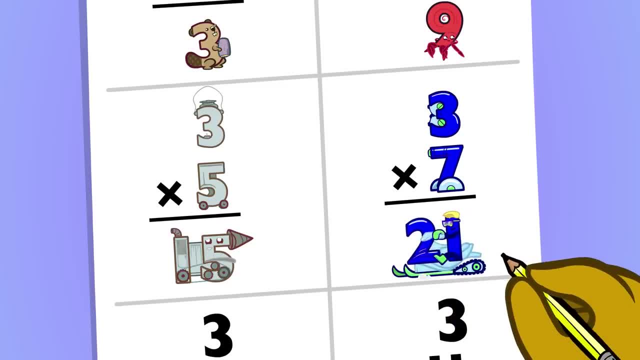 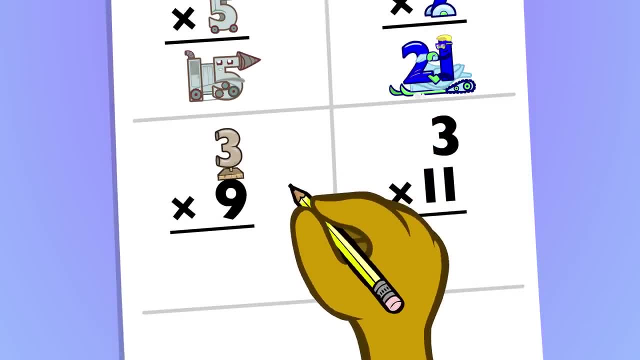 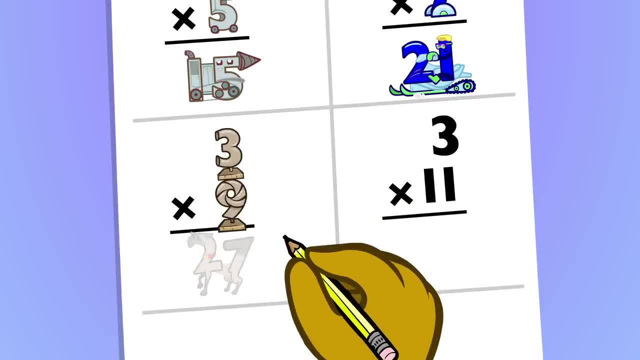 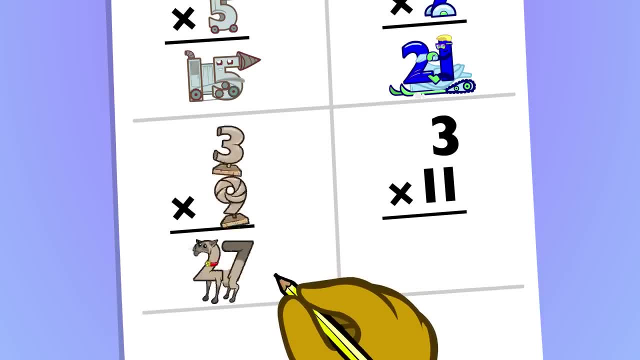 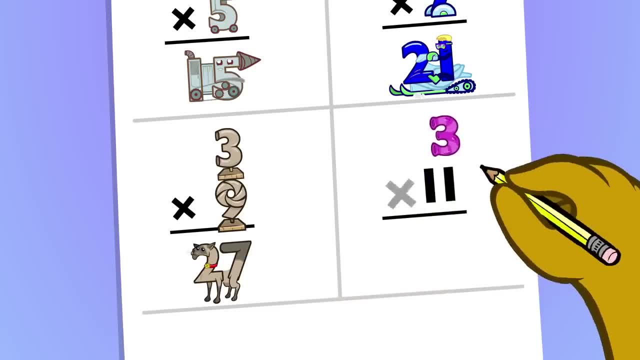 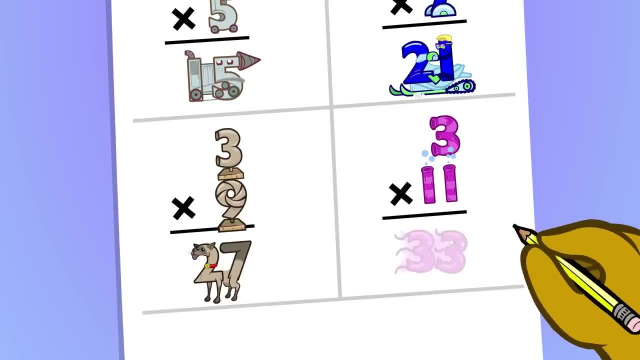 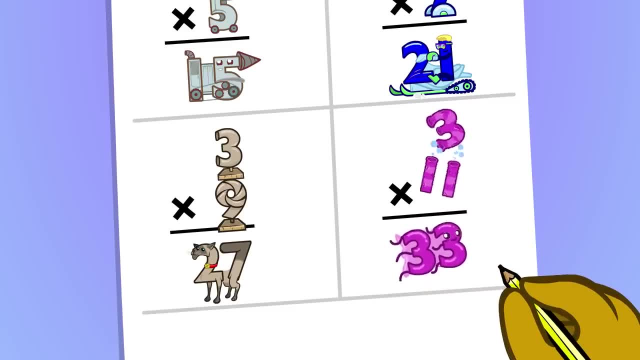 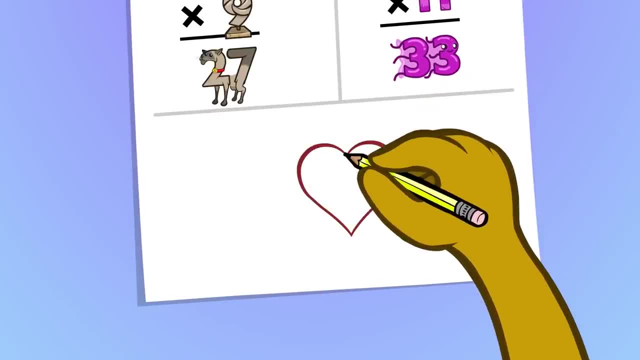 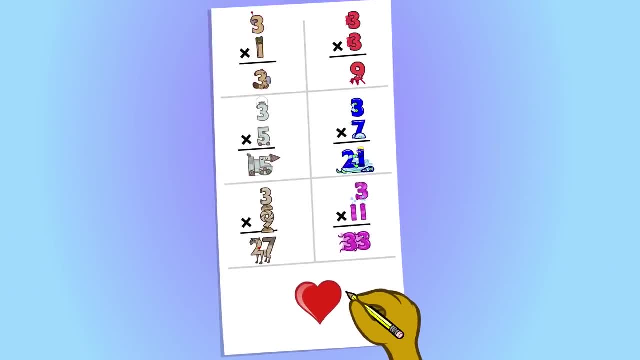 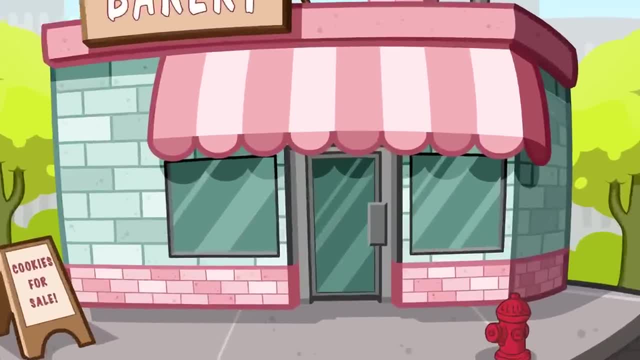 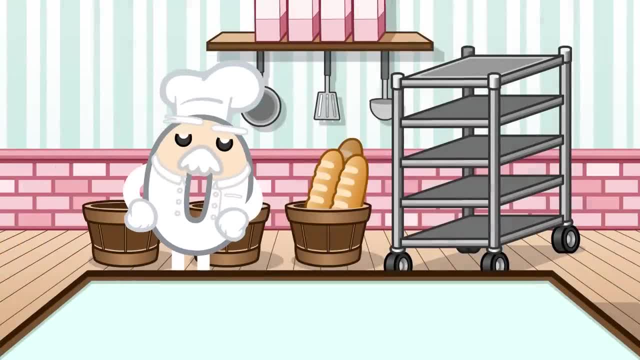 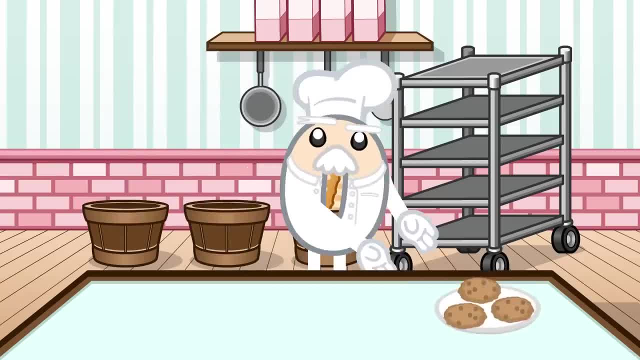 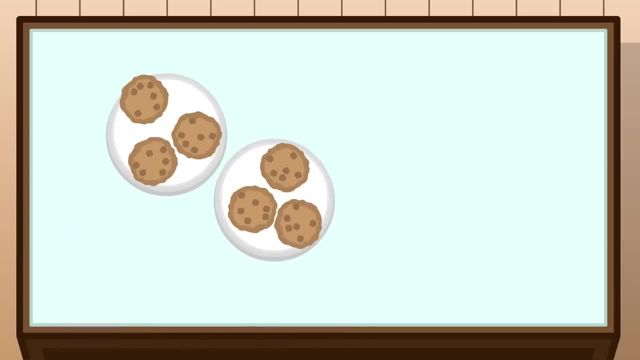 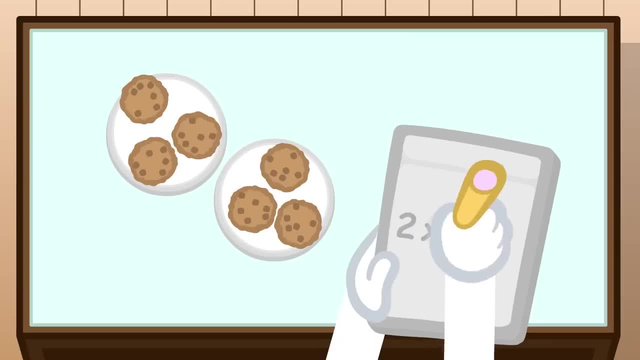 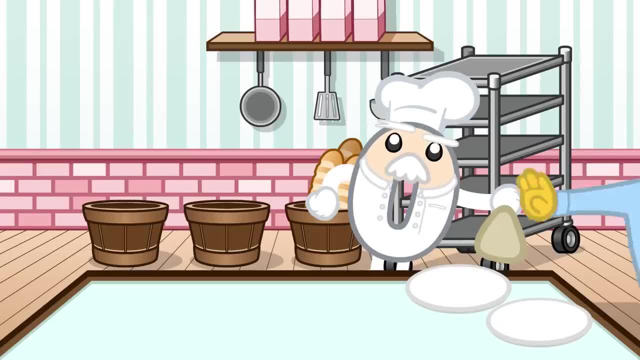 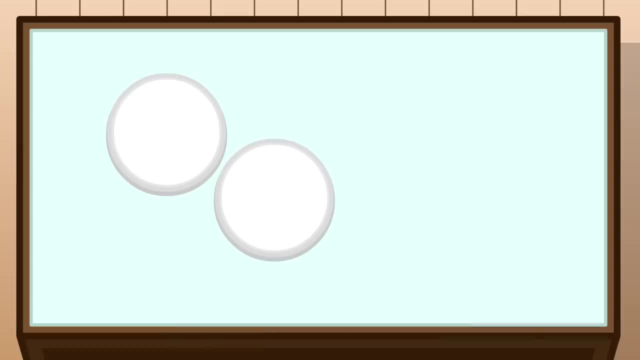 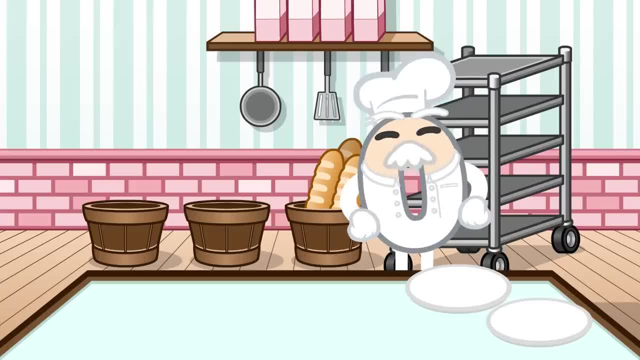 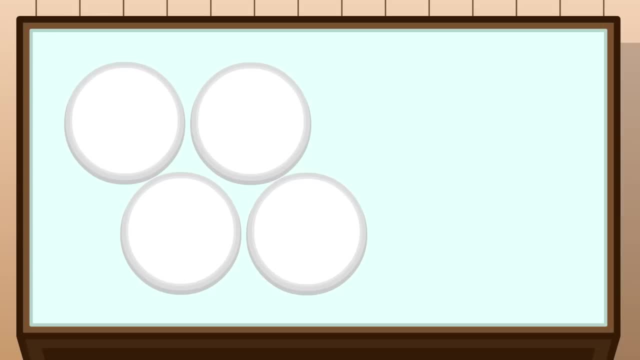 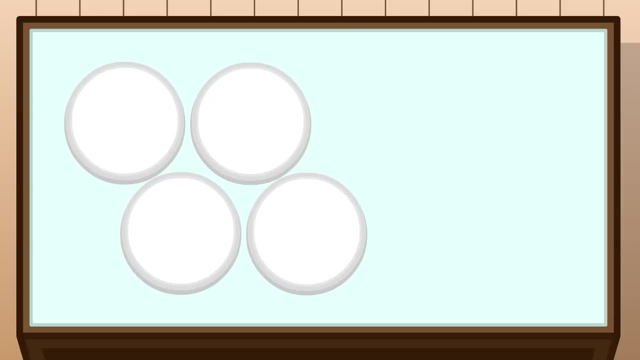 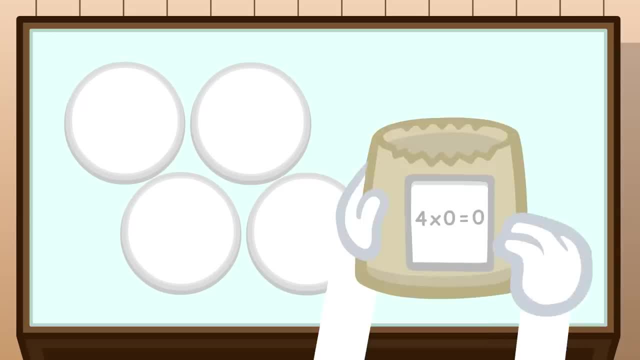 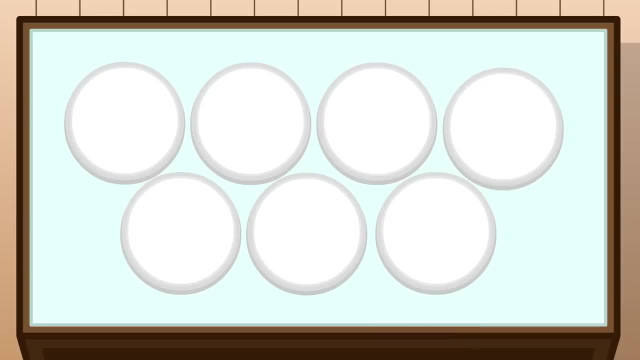 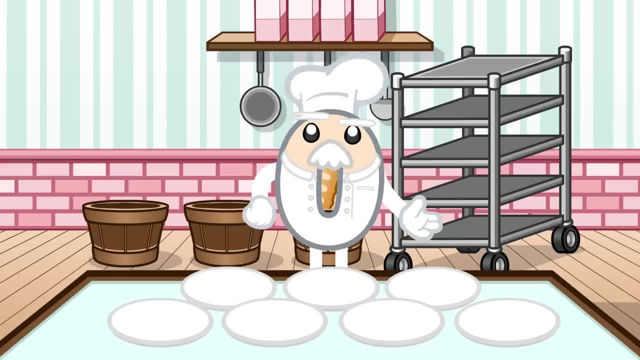 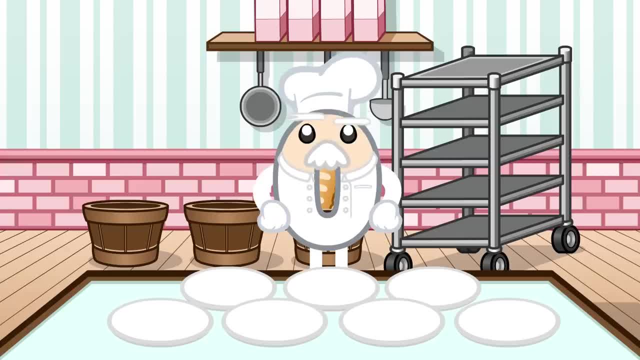 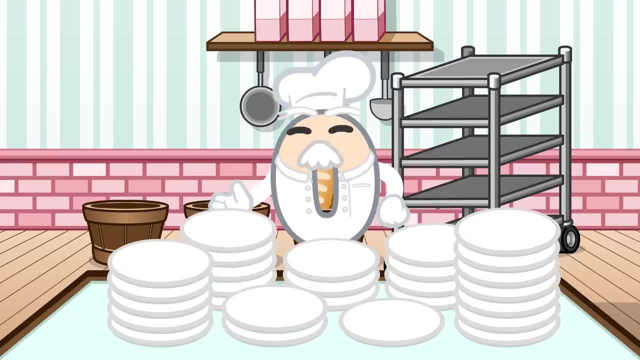 3 x 12 equals 36. 3 x 12 equals 36. 3 x 12 equals 36. Okay, I'm gonna try a very big one Now. I have 27 plates. There are zero cookies on each plate. How many cookies do I have? 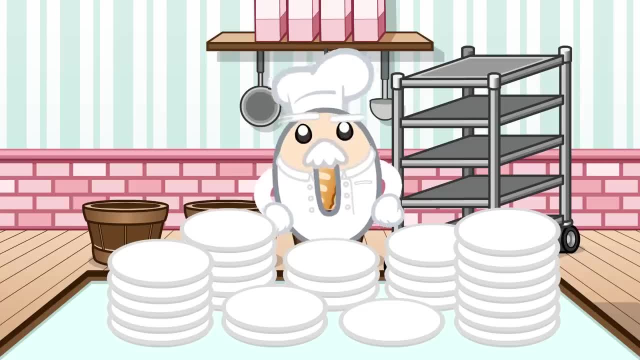 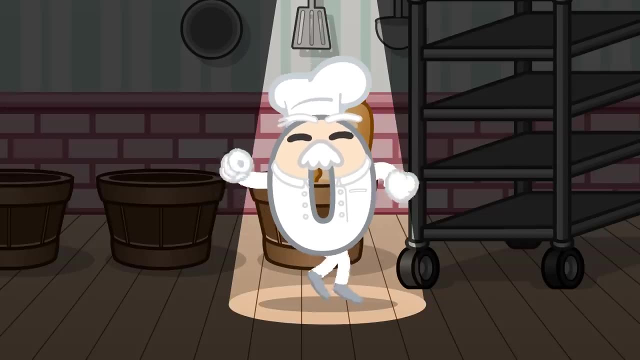 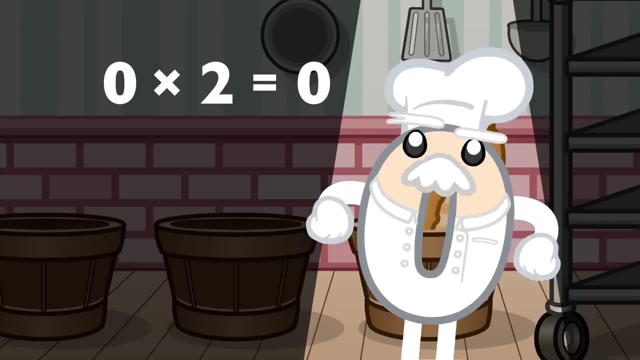 Still zero. It's true. any number times zero equals zero. Looks like we're all out of cookies for the day. We'll make some more tomorrow. Zero times zero equals zero. Zero times one equals zero. Zero times two equals zero. 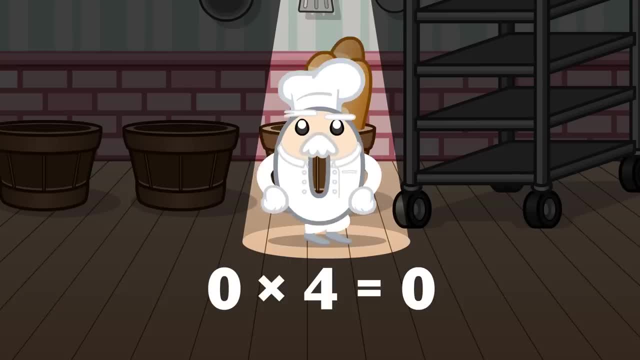 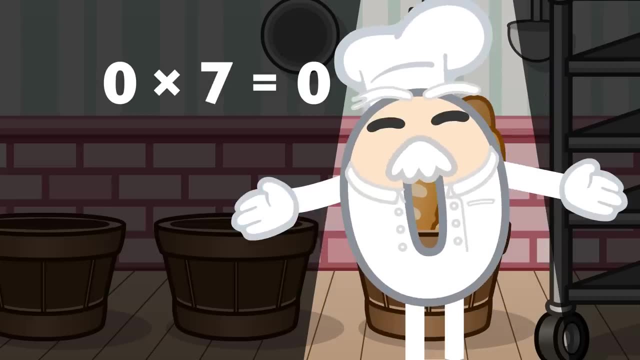 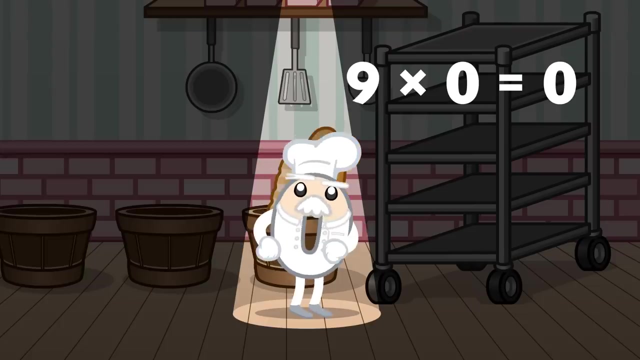 Zero times three equals zero. Zero times four equals zero. Zero times five equals zero. Zero times six equals zero. Zero times seven equals zero. Now let's try it with a zero in the middle. Eight times zero equals zero. Nine times zero equals zero. 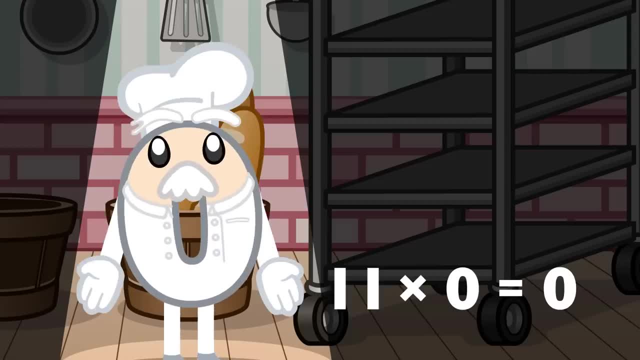 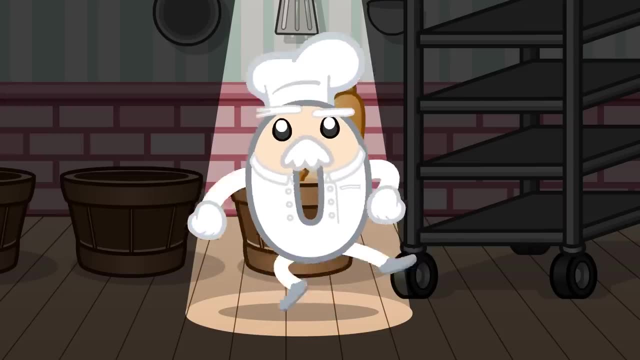 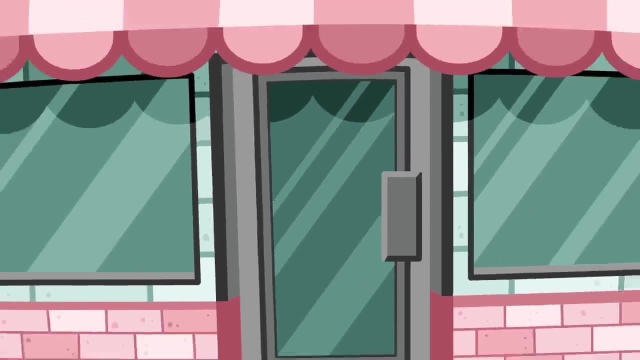 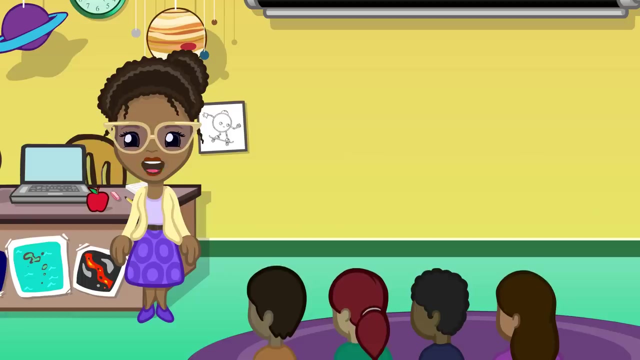 10 times zero equals zero. 11 times zero equals zero. 12 times zero equals zero. And now you can see: when you multiply by zero, the answer will always be zero. Now that you've learned your multiplication math facts, did you know that you can use them to do division too? 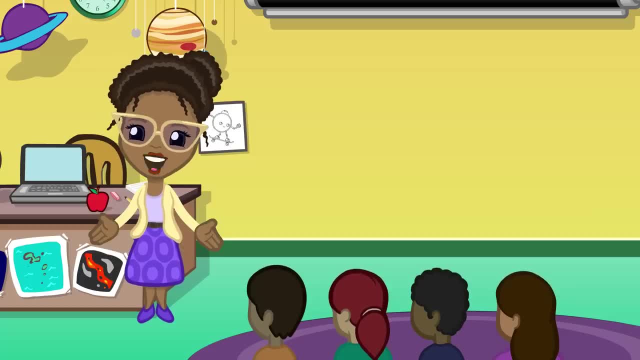 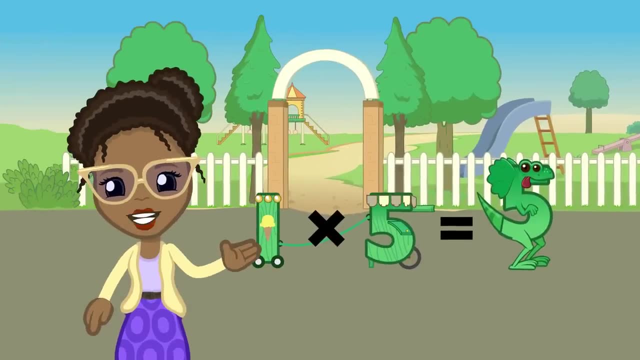 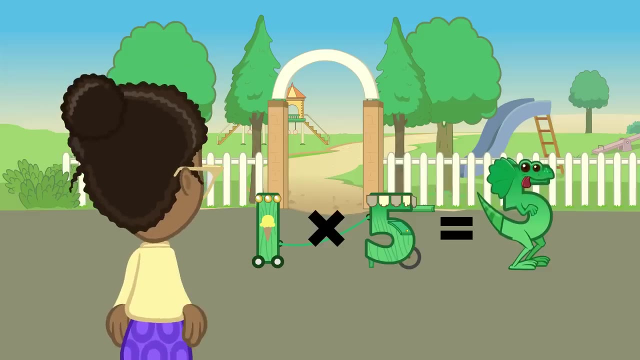 It's easy, With the help of my friends from all around the world. I will show you how Okay. here we have the fact: family one times five equals five. Let's turn this multiplication problem into division. Now let's move the biggest number to the beginning. 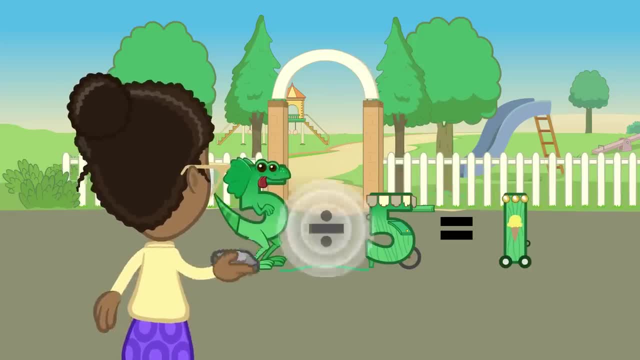 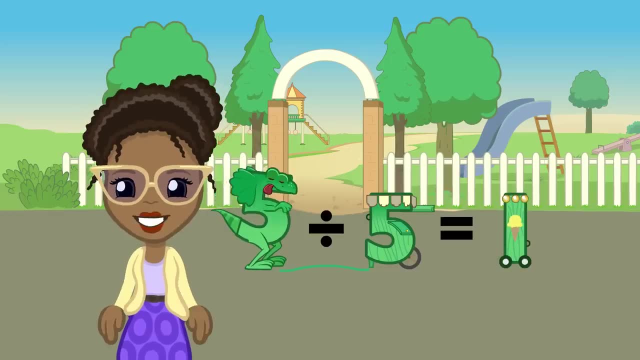 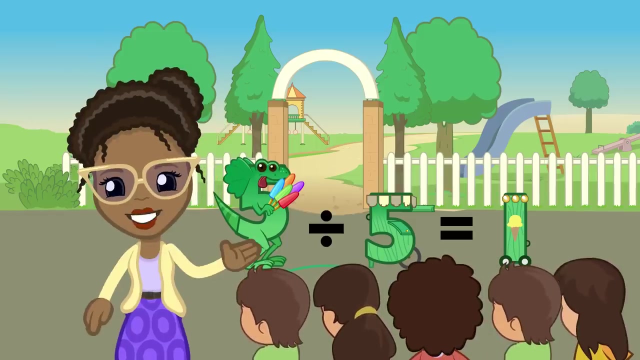 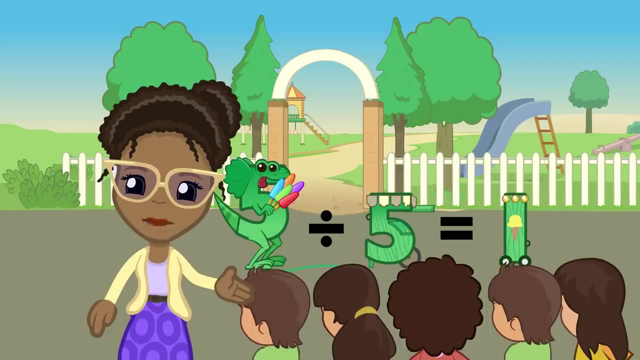 Now there's one more thing. Good, Five divided by five equals one. Five divided by five equals one. There are five ice pops. There are five children. How many ice pops does each child get? One, That's right. Five ice pops divided by five kids equals one. 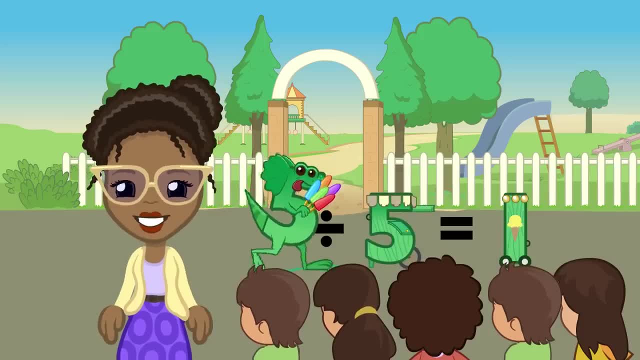 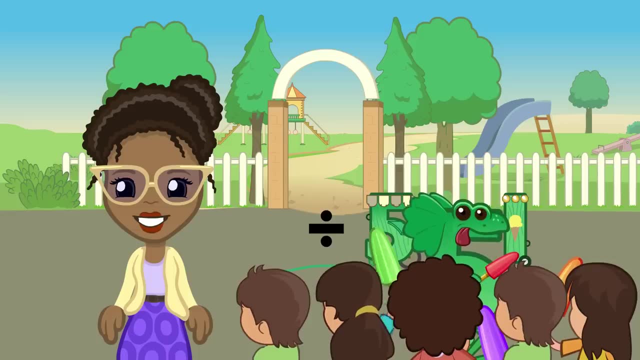 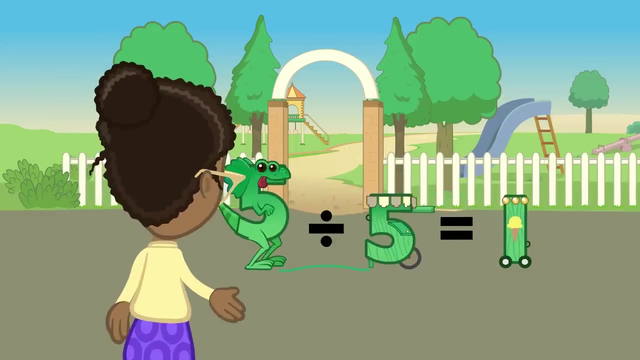 Five divided by five equals one. That's right. Five ice pops divided by five kids equals one. Five divided by five equals one One. Now let's make another division equation: 5 divided by 5 equals 1. And 5 divided by 1 equals 5.. 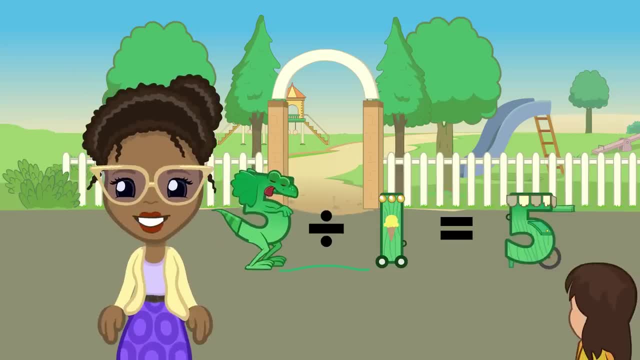 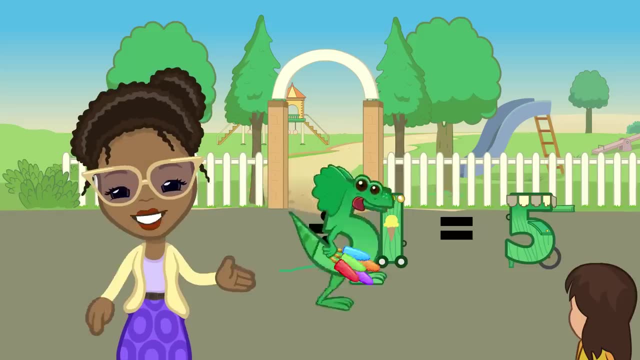 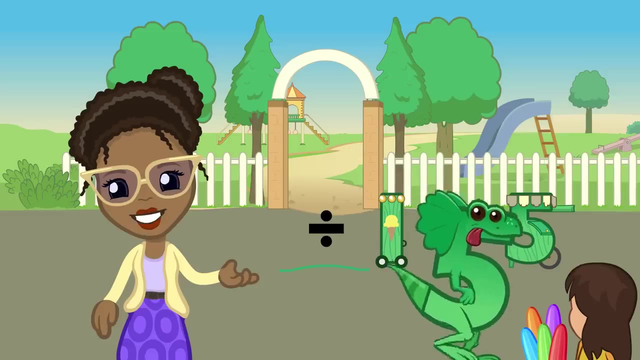 What if there is only one child? 5 divided by 1 equals 5! That's right. If you have 5 pots to give away and only one child, she gets to take them all. Don't worry, I'm sure she will share them. 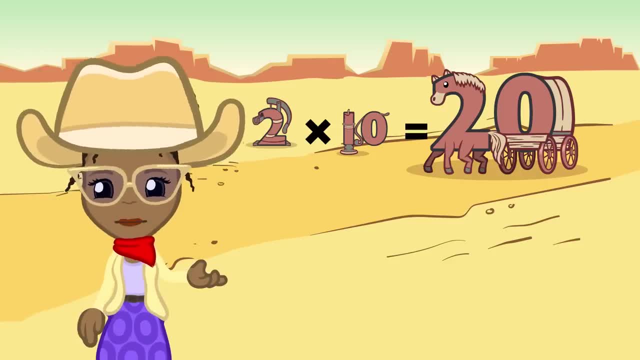 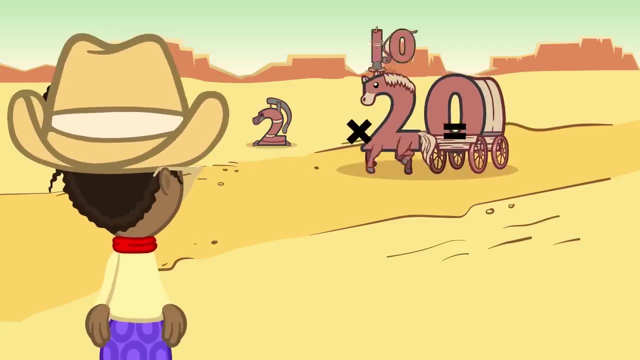 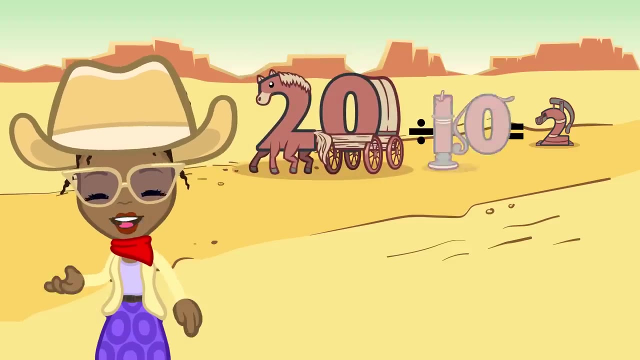 Howdy partner. Let's turn this multiplication problem into division. 2 times 10 equals 20.. Now let's move the biggest number to the beginning. 20 divided by 10 equals 2.. He has 20 gold nuggets. 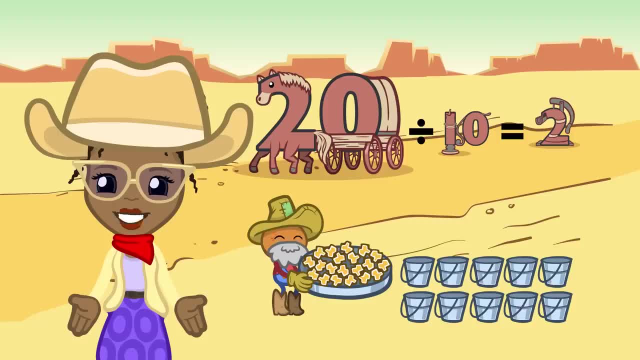 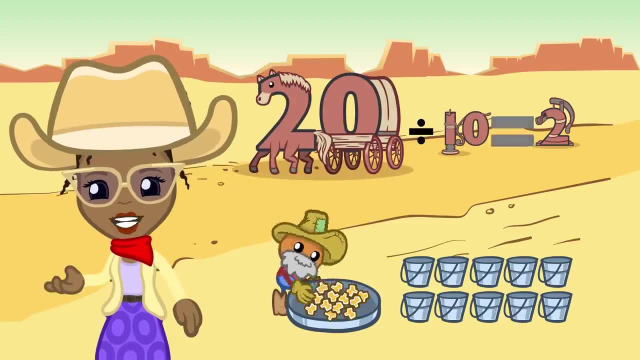 He has 10 buckets. How many gold nuggets will he put in each bucket? 2!, That's right. 20 divided by 10 equals 2.. He puts 2 gold nuggets in each bucket. Let's do another division problem. 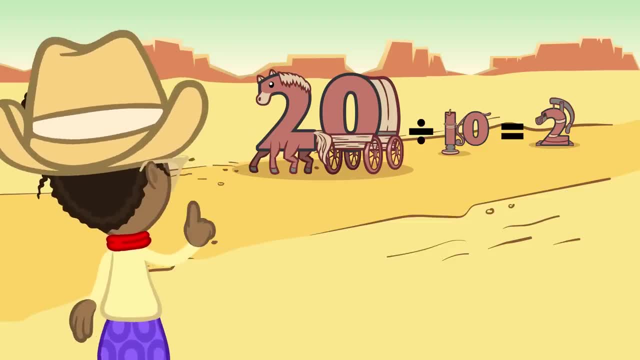 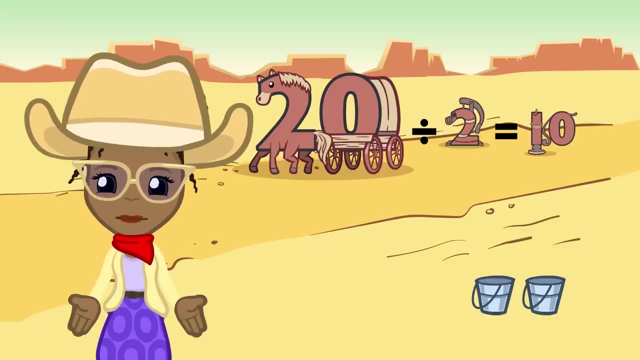 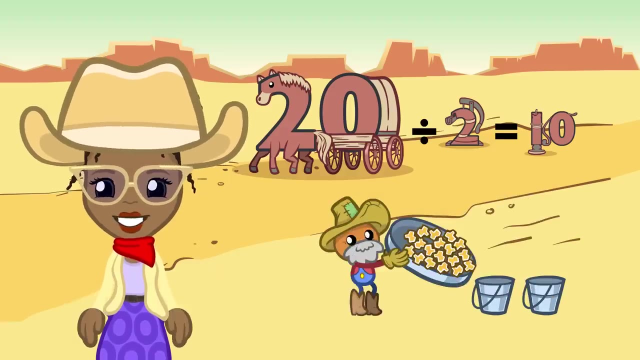 20 divided by 10 equals 2.. And 20 divided by 2 equals 10.. Now there are only 2 buckets. There are 20 gold nuggets And 100 gold nuggets. That's right. How many gold nuggets should he put in each bucket? 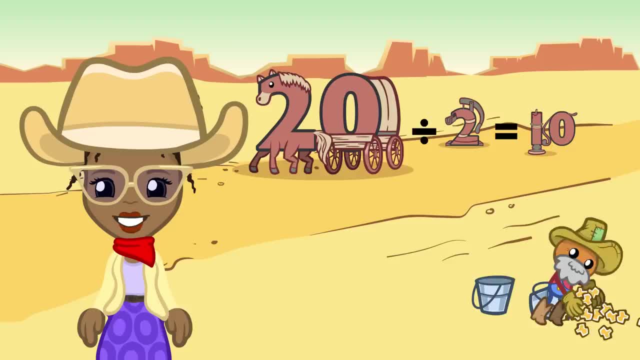 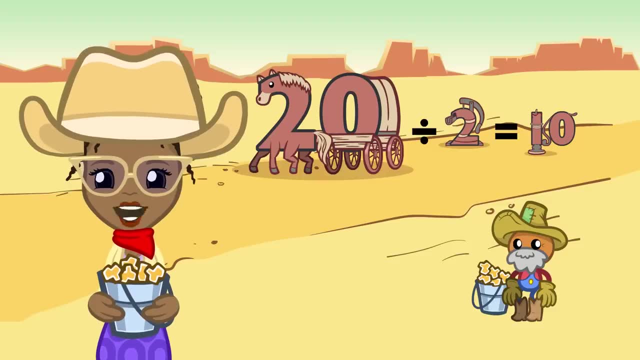 He puts more 2 forgettes into the bucket. How many gold nuggets should he put in each bucket? Only 2 points. No, You have to make it even. That's right. When you are doing division, you have to divide into equal amounts. 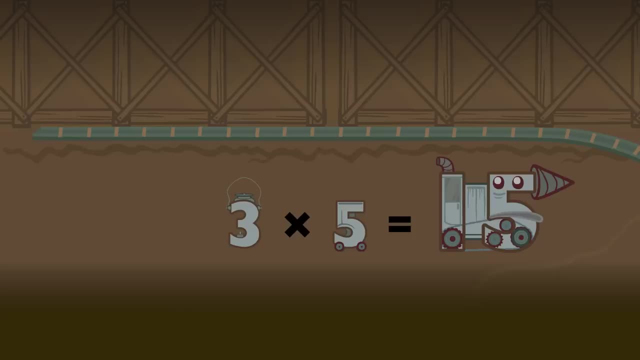 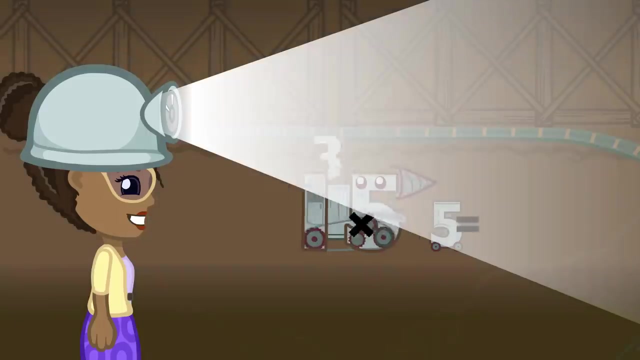 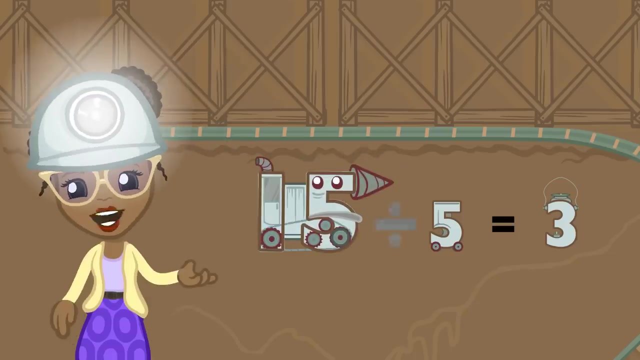 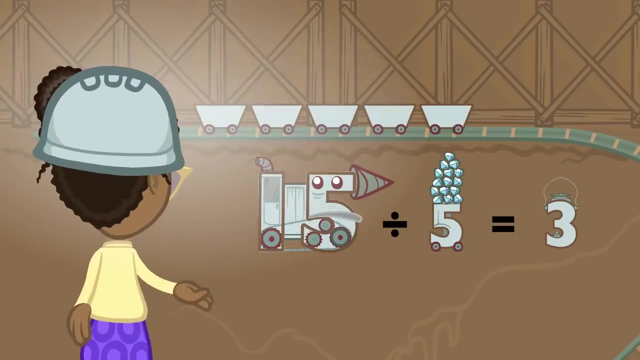 So the answer is 10.. Wow, it's dark in here. Now let's move the biggest number to the beginning. 15 divided by 5 equals 3.. There are 15 gems and we need to divide them evenly into 5 carts. 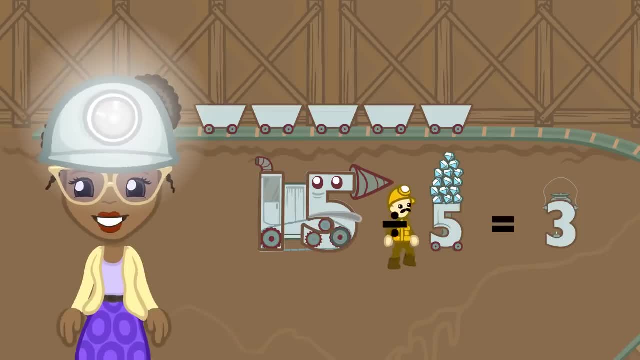 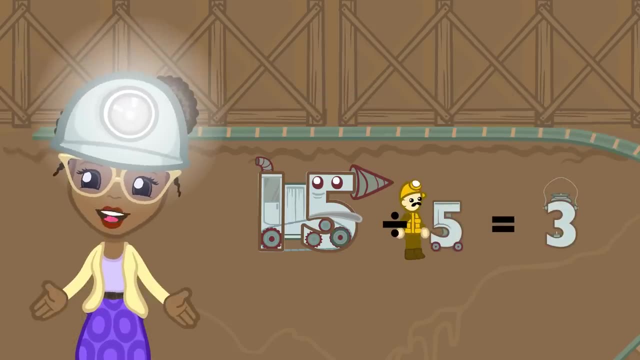 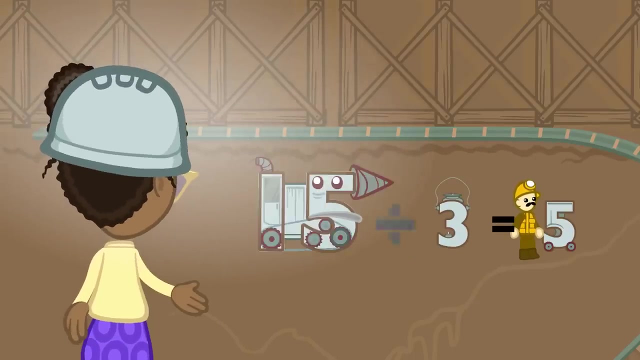 How many gems go in each cart? 3! Yes, 15 divided by 5 equals 3.. Let's try another: 15 divided by 5 equals 3.. And 15 divided by 3 equals 5. There are 3 carts. 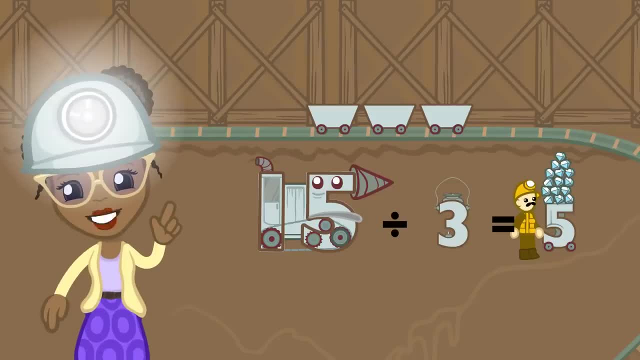 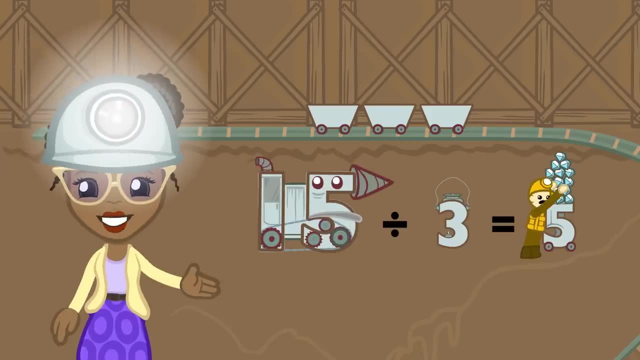 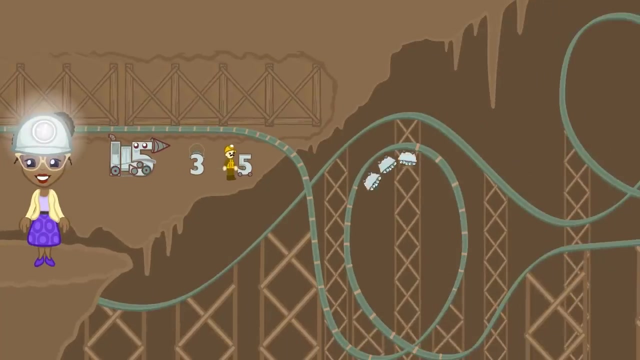 There are 15 gems. How many gems can be divided evenly into 3 carts? 5!, That's right. 15 divided by 3 equals 5.. He put 5 gems in each cart. Oh, doesn't that look like fun. 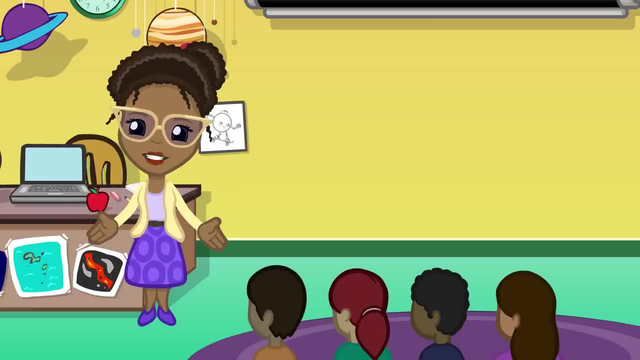 Learning to divide was so much fun, and I want to tell you one more thing. There are many ways to write a division equation. I will show you a few: 8., 8., 8., 8., 9., 6.. 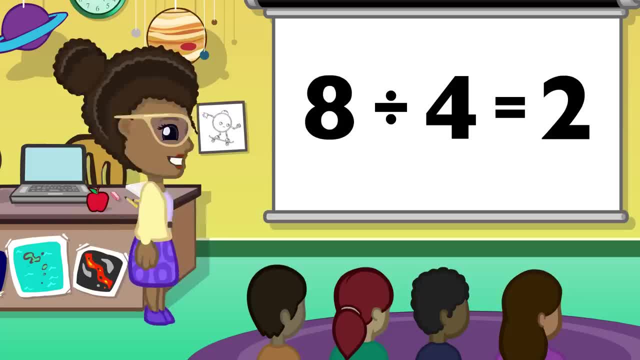 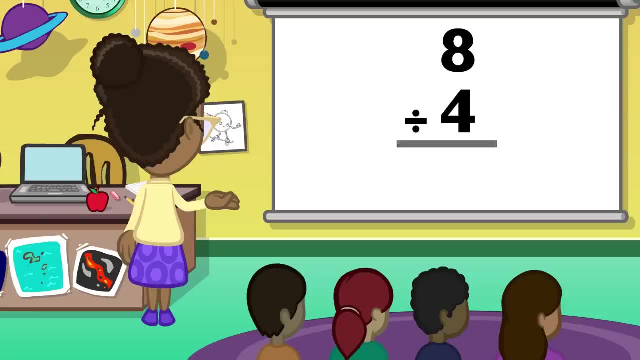 6., 7., 2., 8.. ereye, 6., 6., 6., 6.. 8 divided by 4 equals 2.. There is another way to write this equation: 8 divided by 4 equals 2!. 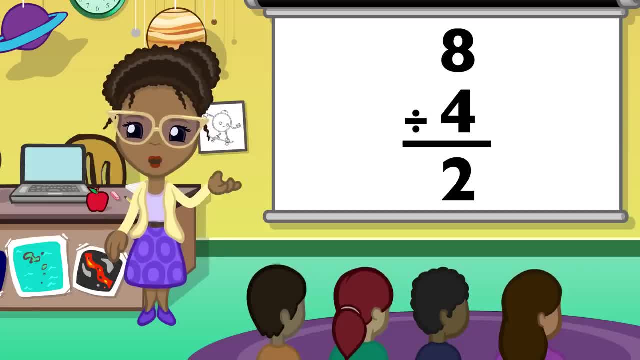 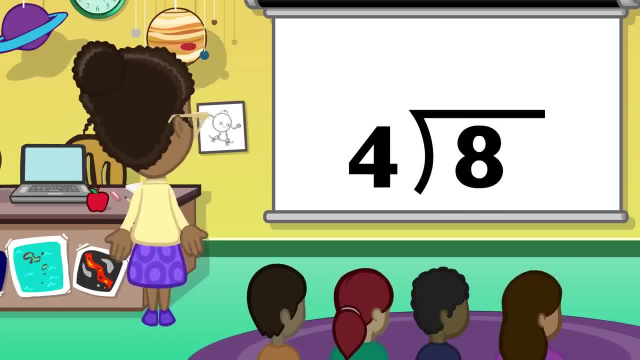 Guess what We are not done. There are a couple of other ways to write this equation. I know this looks strange, but it means the same thing: 8 divided by 4 equals 2.. 8 divided by 4 equals 2.. You might also see it written: 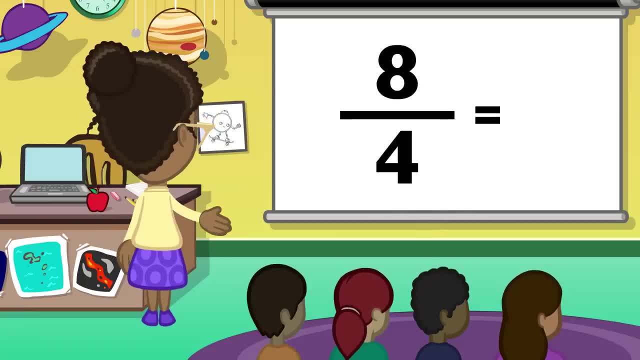 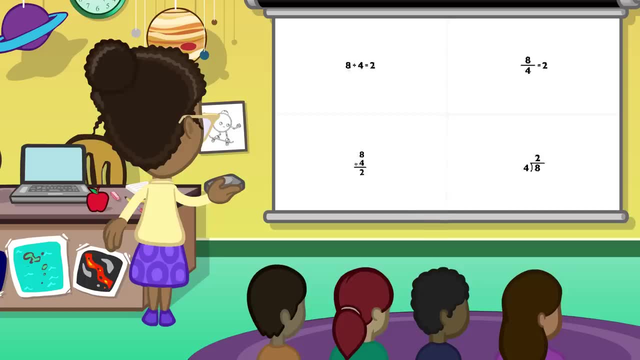 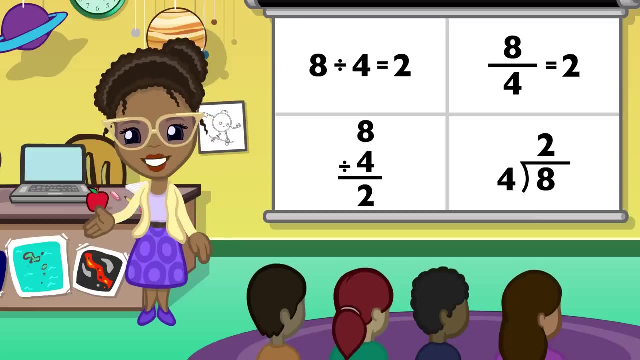 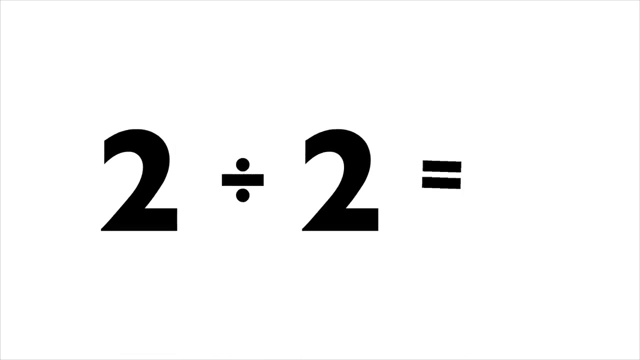 this way, 8 divided by 4 equals 2.. 8 divided by 4 equals 2.. In other words, all four equations that you see on the board mean the same thing. They just look a bit different. Let's practice: 2 divided by 2 equals 1.. 4 divided by 1 equals 4.. 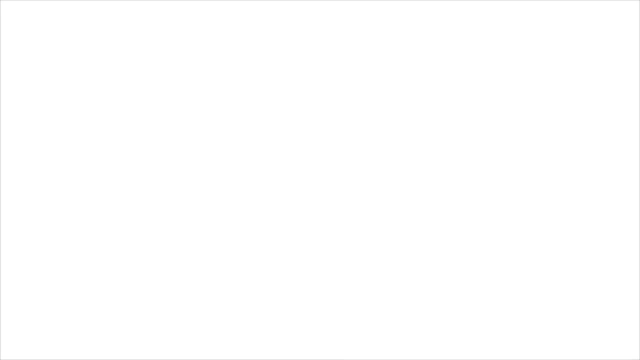 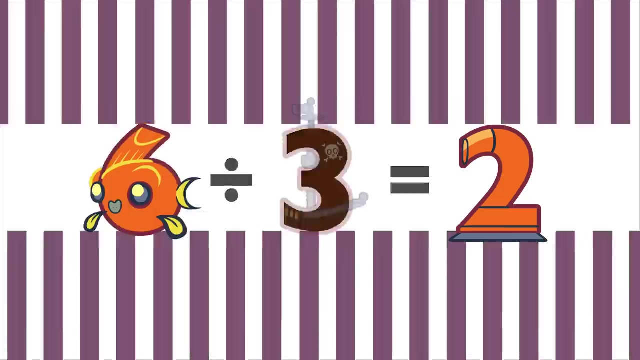 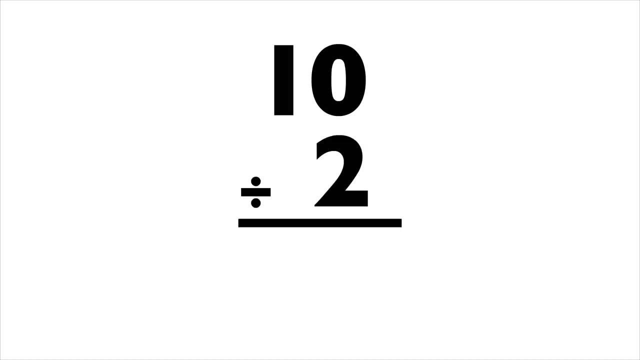 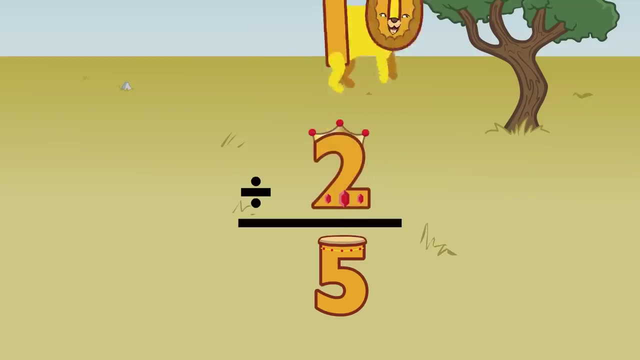 8 divided by 8 equals: 1. 0 divided by 10 equals 0.. 6 divided by 3 equals: 2. 10 divided by 2 equals: 5.. 11 divided by 12 equals 6.. You're done. 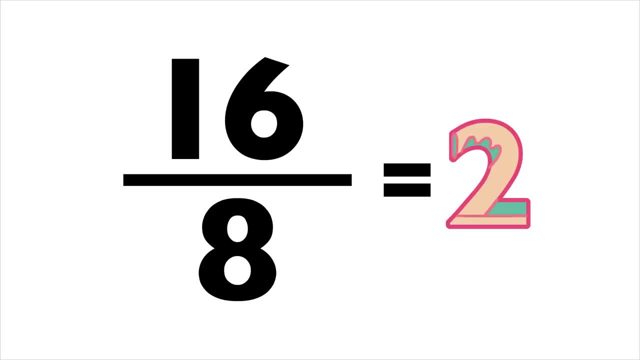 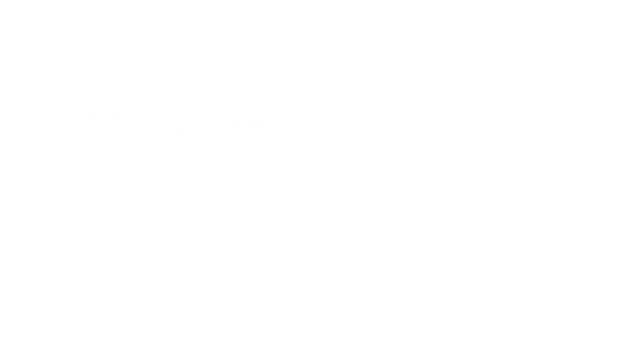 16 divided by 11 equals. 6. 9 divided by 8 equals. 2. 9 divided by 3 equals. 3. 21 divided by 7 equals. 3. 30 divided by 3 equals. 10. 20 divided by 3 equals: 3.. 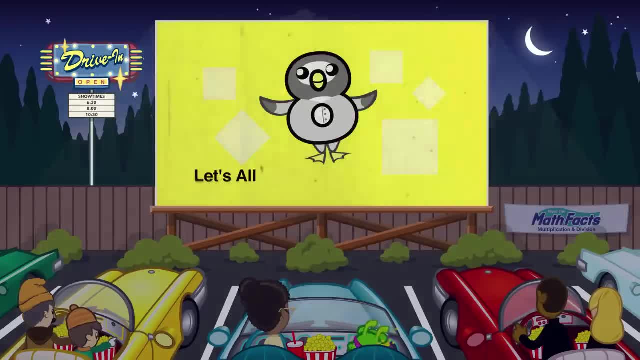 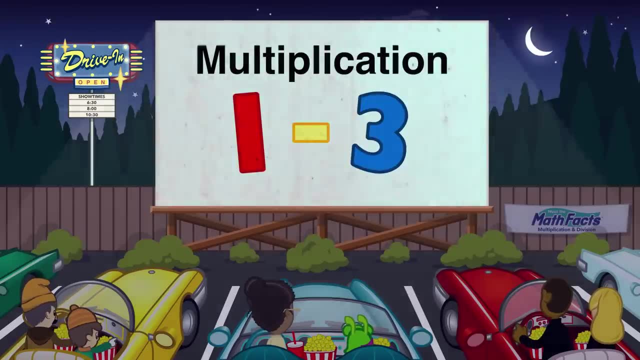 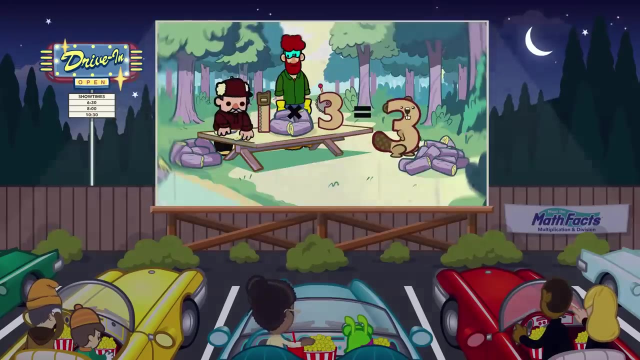 Let's all practice our math facts. Let's all practice our math facts. Let's all practice our math facts. Multiplication 1 through 3.. 1 times 1 equals 1.. 1 times 2 equals 2.. 1 times 3 equals 3.. 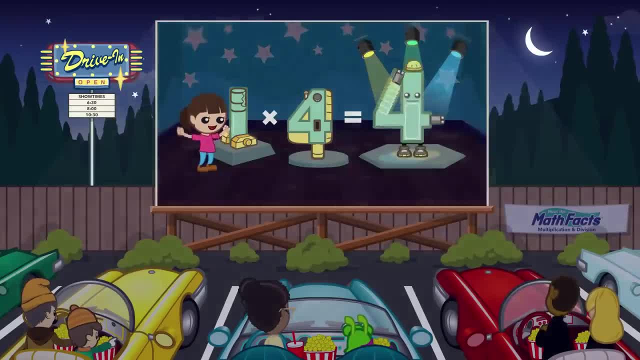 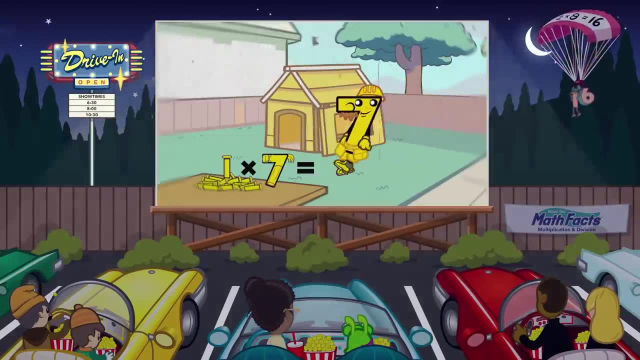 1 times 4 equals, 4.. 1 times 5 equals, 5.. 1 times 6 equals. 6.. 1 times 7 equals, 7.. 1 times 8 equals, 8.. 1 times 9 equals, 9.. 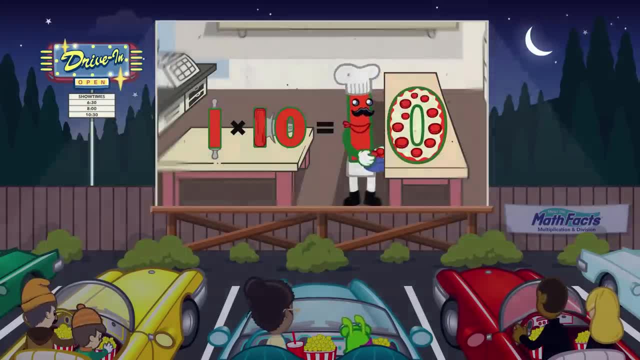 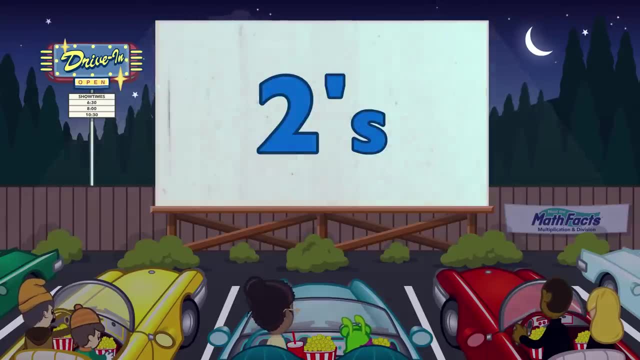 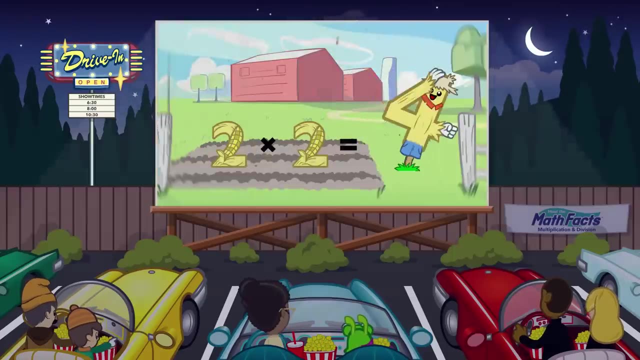 1 times 10 equals 10.. 1 times 11 equals 11.. 1 times 12 equals 12.. Now let's try twos: 2 times 1 equals 2.. 2 times 6 equals 4.. 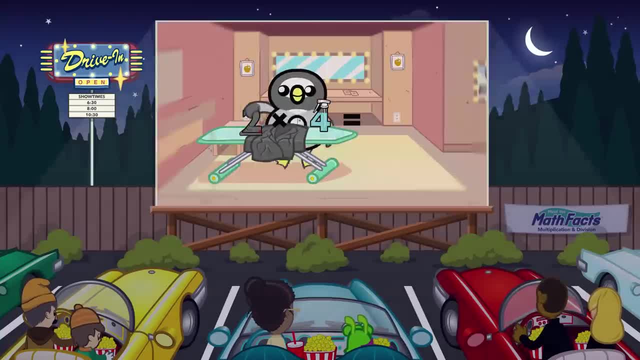 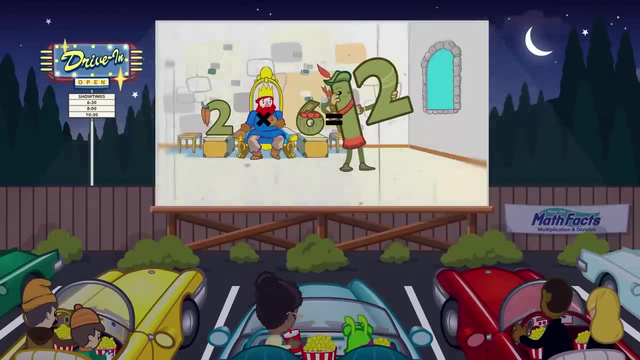 2 times 3 equals 6.. 2 times 4 equals 8.. 2 times 5 equals 10.. 2 times 6 equals 12.. 2 times 7 equals 14.. 2 times 8 equals 16.. 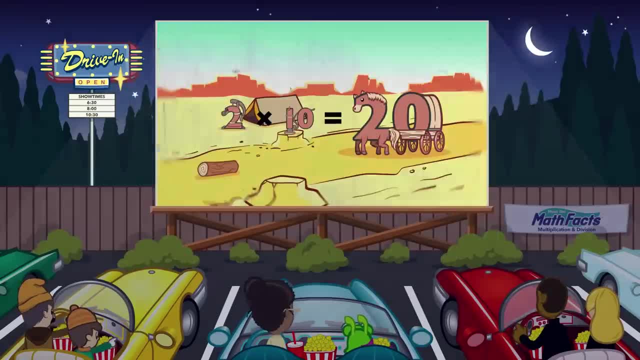 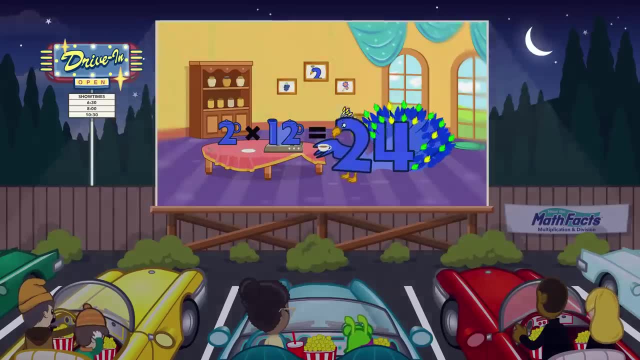 2 times 9 equals 18.. 2 times 10 equals 20.. 2 times 11 equals 22.. 2 times 12 equals 24.. Let's try threes: 3 times 1 equals 3..